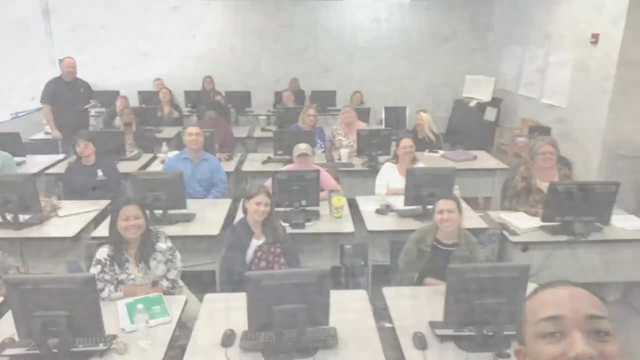 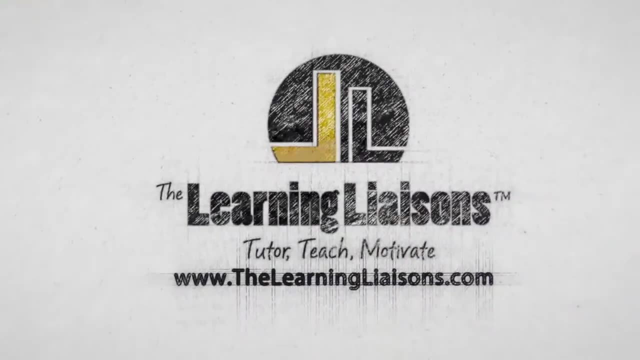 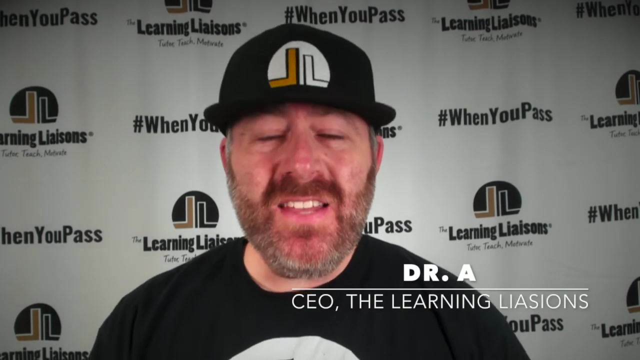 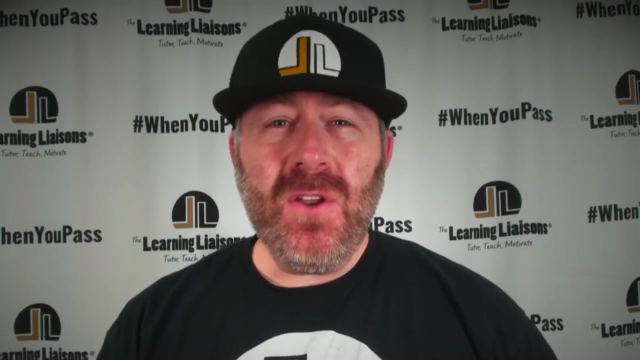 When you pass, not if you pass. Hey there, Dr Ray here, CEO of the Learning Liaisons, and in this video you're going to be able to watch one of our recent webinar recordings where our math director, Anderson Duran, is going. 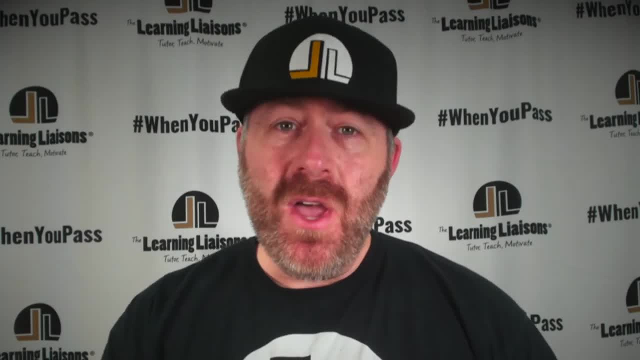 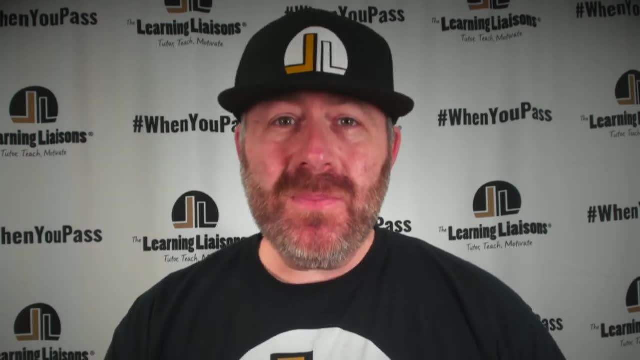 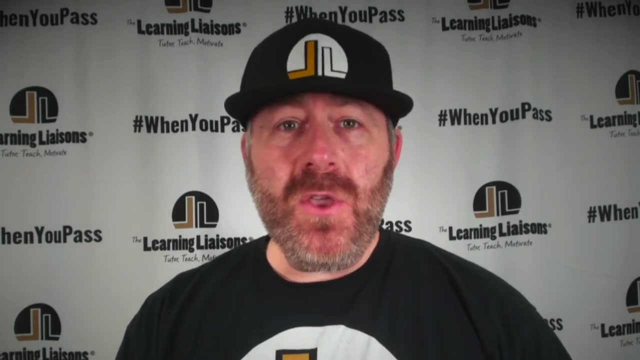 to focus its efforts on helping teachers. if one of you guys fall into this category- teachers who have to pass their praxis exam for elementary education math subtest, as well as your K-6 subject area exam for our Florida teacher certification exam. So, whether you are in, 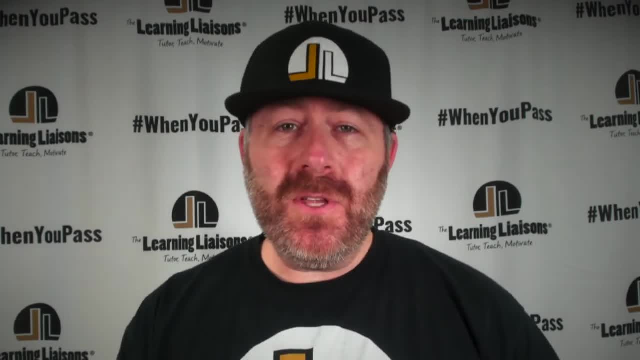 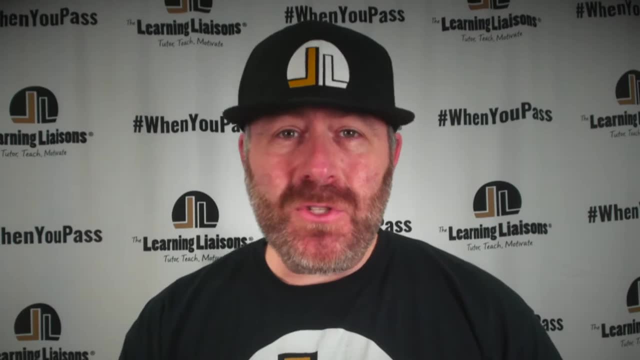 the state of Florida or outside, and you have to take the praxis exam. this is going to be a great webinar recording for you to watch- To watch as our math director Anderson shows you how to break down those ever so difficult word problems that you'll see on your upcoming certification. 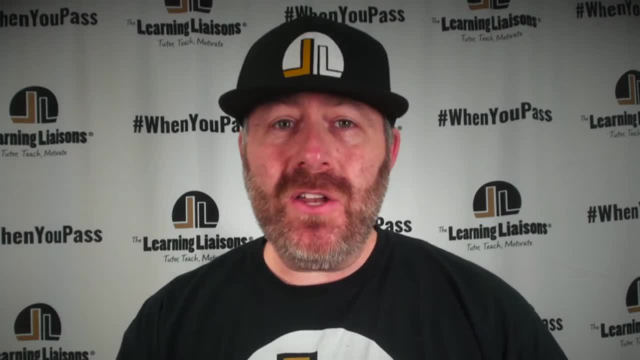 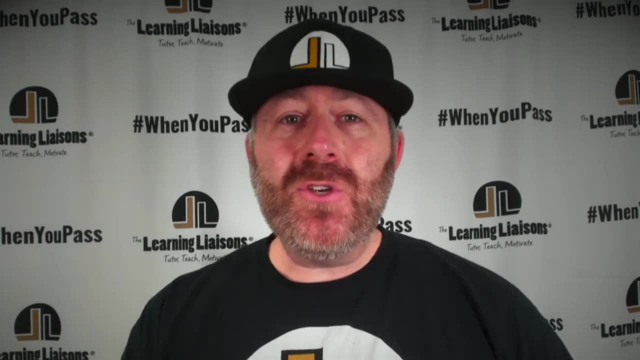 exams. He's going to introduce you to our proven test-taking strategy on how to analyze word problems in math. and that is Destination Plan Follow. So stay tuned, watch the video, make sure you like, subscribe and comment, and please share. 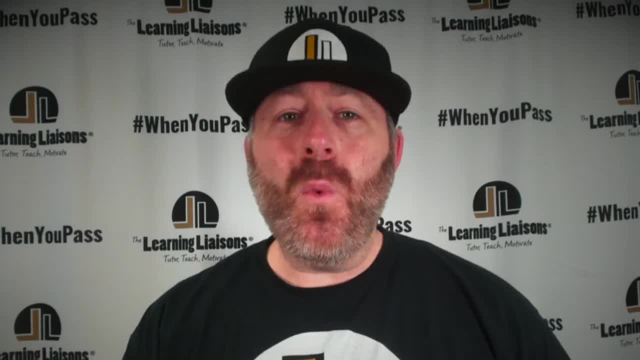 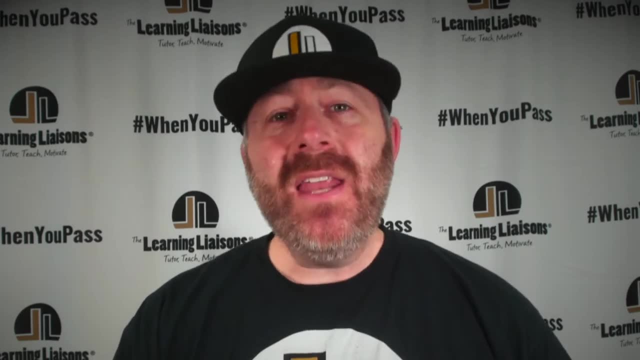 this YouTube channel with your friends who are in that same field of working towards their certification. So here at the Learning Liaisons, we always like to tell our teachers and college students: always remember it's when you pass, not if you pass your certification exams. Enjoy the. 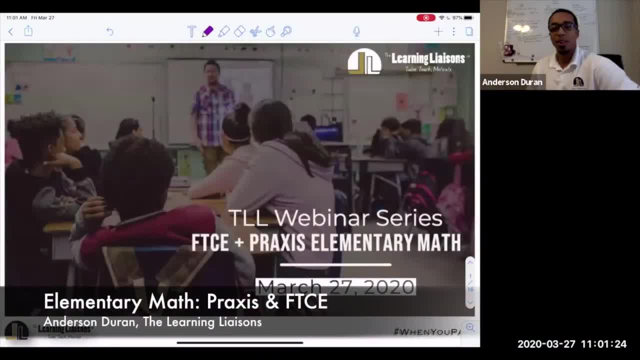 video and let us know what you think. All right. all right, and we are back. It is 1101, and it looks like there's a few people here, quite a few people here actually. This is awesome, So let's go. 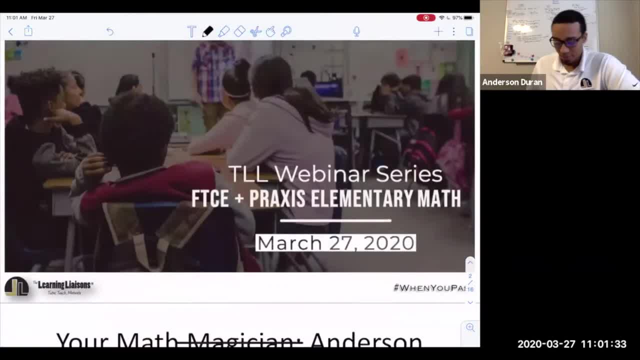 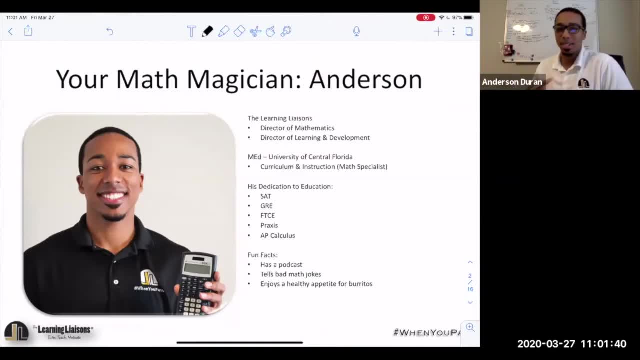 ahead and dive right in. everybody, Let's go ahead and dive right in. So just want to make sure I introduce myself, to make sure that everybody here feels comfortable learning from me. I am not here to waste anybody's time. So my name is Anderson, last name: Duran. first name is Anderson. I'm the. 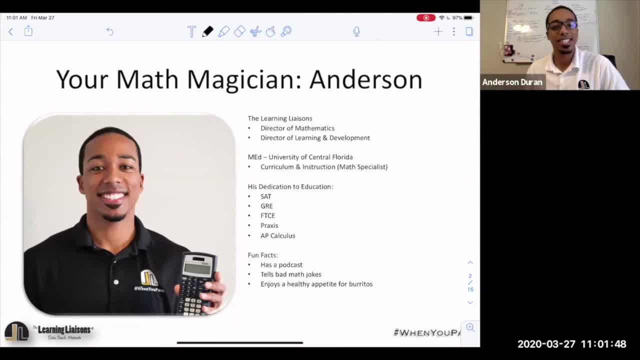 math director and the director of learning and development at the Learning Liaisons, and I've been here for a little over two and a half years now and it's just been, honestly, the best experience I've ever had. So I can't wait to begin the course. So let's dive right in. Hi, I'm Anderson. I'm 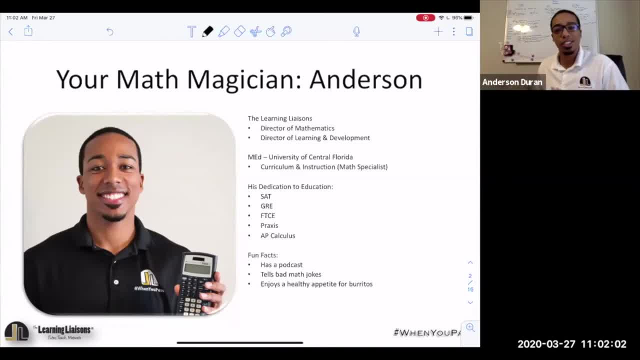 an assistant departmentu. I'm a continuing education advisor. My Name is Anderson and I teach technology at the Learning Liaisons. for a number of reasons, My main purpose in continuing education has been to help other people succeed, So doing everything here, you know, helping other. 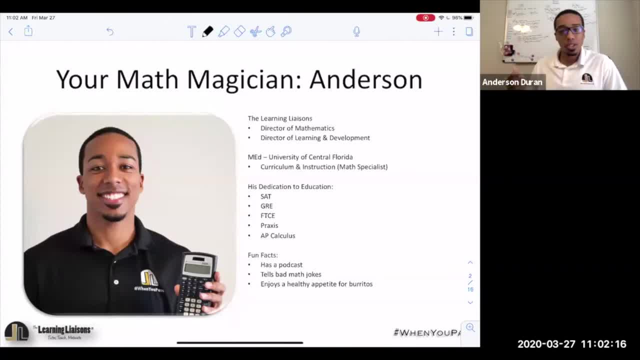 teachers get their certifications and then go on to help hundreds of kids a year. You know that's just that means the world to me. So I thank you guys for joining together here in this tough time. Praxis, as you guys know, and AP Calculus. 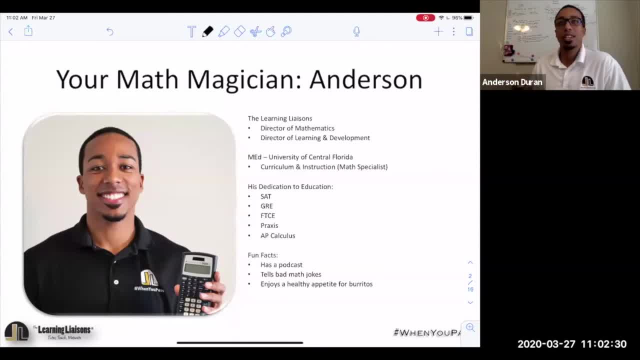 So again, I have some experience here in education, especially when it comes to teaching math, because the reason I became a teacher was because my professors in college- as much as I knew they were getting paid- I realized they were reading straight out of a textbook. 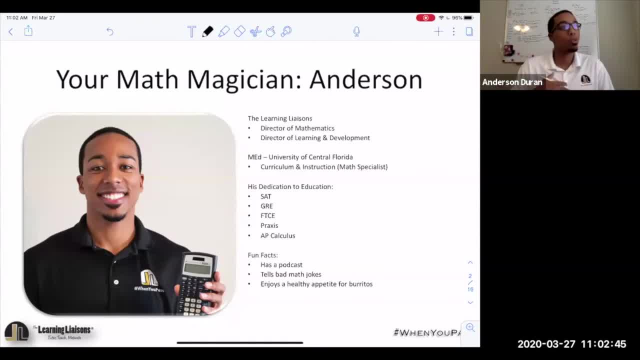 They didn't know how to teach. They didn't put the students first. Most of them were there for research grants and things like that in that math department And that was cool and all, but I saw that there was a little gap in terms of their ability to bring us. 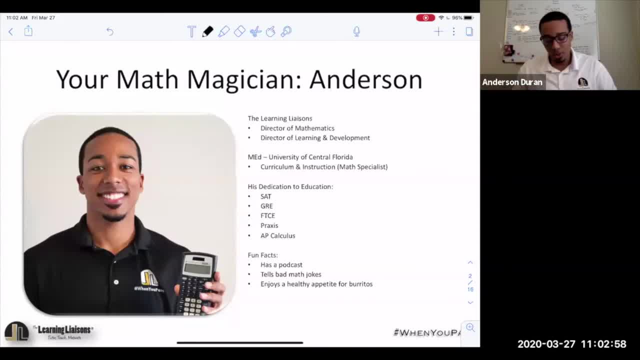 from where we were to what they knew. And so from that day, I kind of started dedicating my life to education and helping other people help themselves. And so you guys are in the same boat. You wanna become certified teachers, you wanna help yourself. 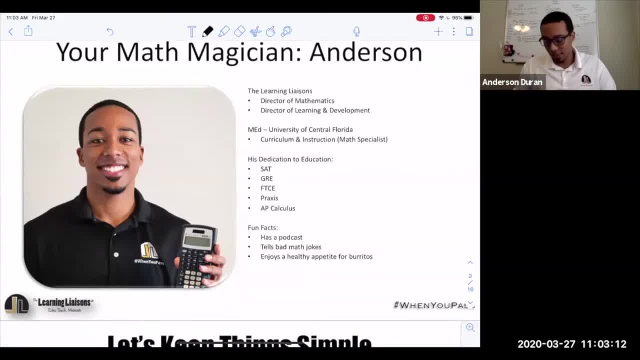 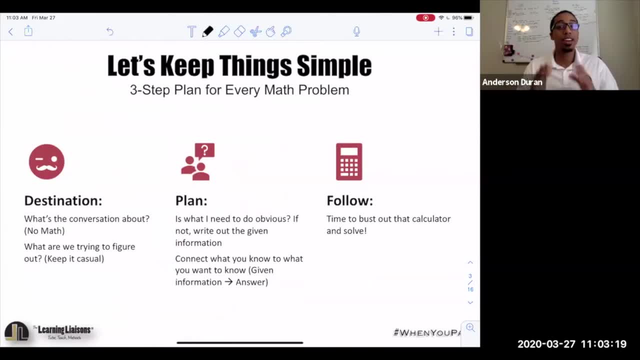 and I'm just here to help that happen. So, with that said, let's go ahead and keep things simple. We're gonna go over this three-step strategy and this strategy is gonna take hold in every single problem. Could be a word problem, could not be a word problem. 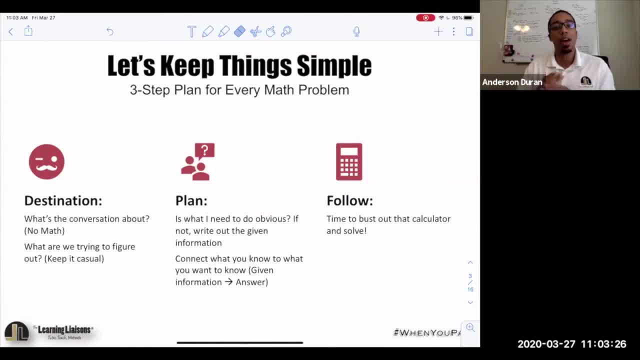 It could be one plus one. We always wanna apply this strategy, no matter what, And so, before I go ahead and talk about it, let me know in the chat box: have you heard me talk about this strategy ever before in your life? Destination plan follow yes or no? 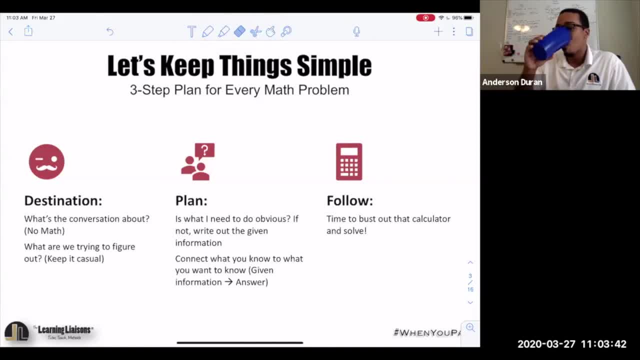 Because, if not, you're in for a treat. today, Nice, quite a few people have a few haven't. All right, so let's just go ahead then and reiterate this, That way we can continue building off of it, getting that knowledge that we need. 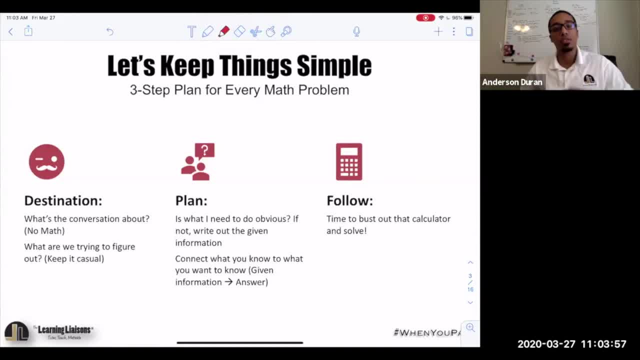 So let's begin. The first step in solving any problem at all is destination. Destination- think about the word It's. oh, where am I ending up? Okay, So destination. there's two things you wanna consider at the beginning of every single math problem. 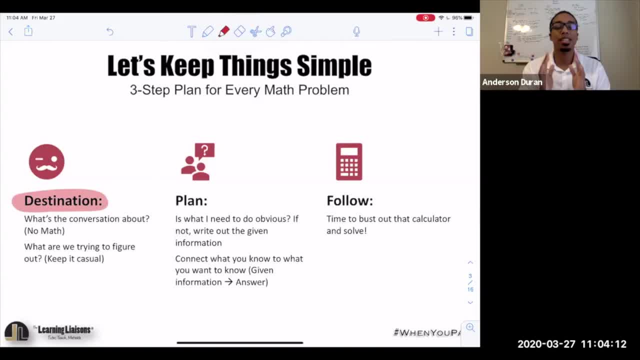 no matter what, And it's about starting simple, keeping things simple. First thing you wanna ask yourself: okay, what did I just read Like? what's the story about? Not the math, not anything complicated. What can I comprehend here? 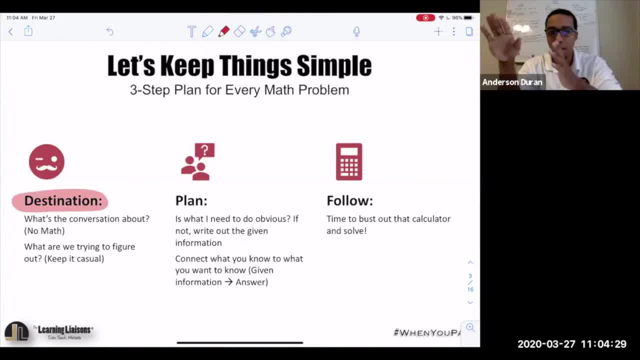 What can I understand? What's the story about? So don't talk about math. Talk about what's going on, the who, what, when, where, why, And then, once you understand the context, you know what's going on. then, okay, what's the question? 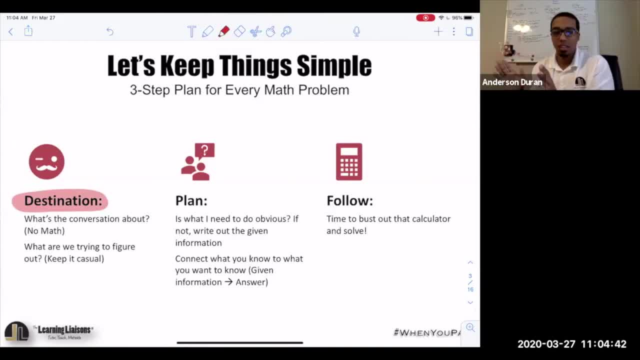 What am I supposed to end up at? What information do I wanna find out? Keep it simple. Try not to use math when you don't need to, But if you do need to sometimes, hey that's okay. But the idea is to only use things. 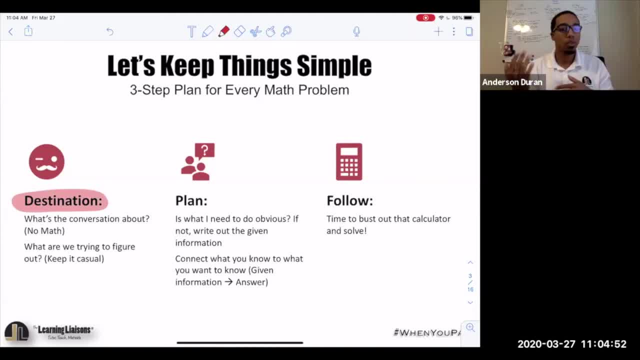 that you can easily recognize, like real everyday words or some of those simple math terms. So again, context and question, that's destination, Because once you understand where you are and where you wanna end up, that's when you start bringing the math in to help you out. 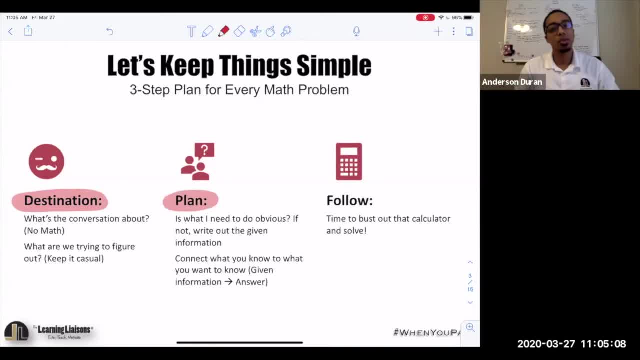 You start making your plan, And so in the planning phase, what you wanna do here is look at your given information or what you have where you need to end up, And you wanna seriously ask yourself: okay, what math ideas or what do I know? logically, 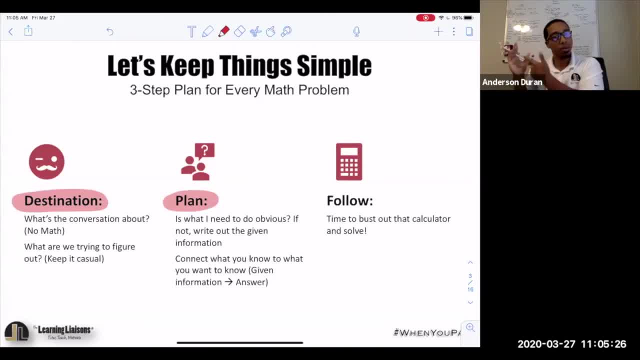 that will connect what I have to what I need to figure out. Or if I wanted to get the answer easily, what information would I need? So, for example, in a problem that asks you: oh, what's you know, this playpen is this. 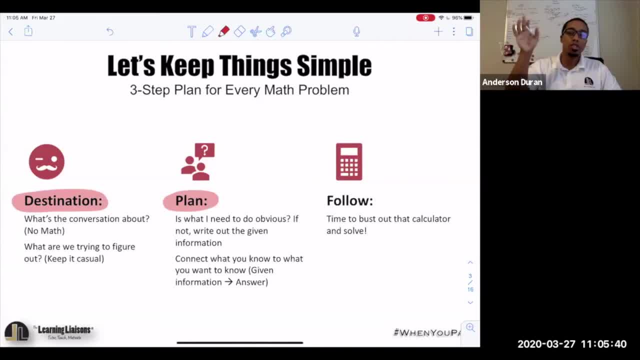 da-da-da-da-da, this many feet tall da-da-da-da. And then the question says: what's the answer? What's the area of the playpen? Okay, so in that question you said: oh, I'm looking for area of the playpen. it's rectangular. 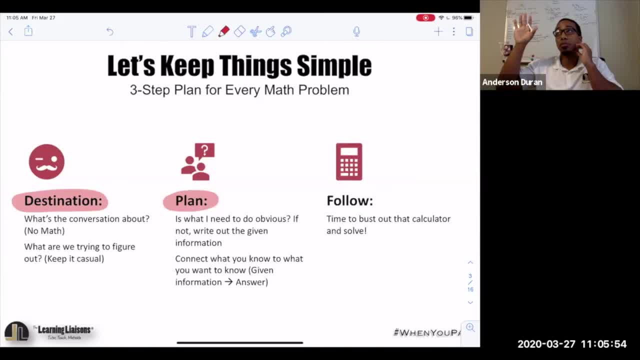 Okay, if I wanted to find the area of a rectangular playpen, what do I need? Oh, yeah, length and width. Oh, do I have that in the problem? Oh, I see one here, gotta find the other one. So do you guys see that in terms of? 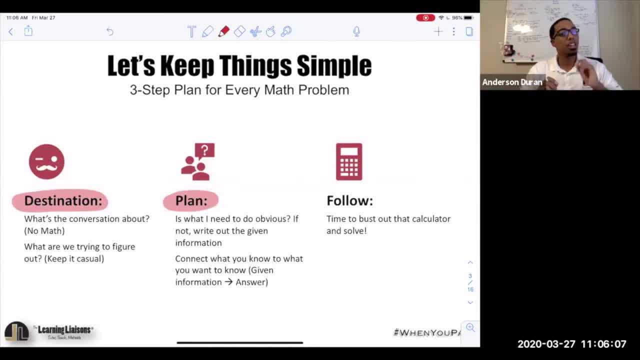 just the structure of solving a problem. Notice how we're not looking at the given information first. we're looking at where we're supposed to end up And we'll see what we need to get there and see if we can find it in the problem. 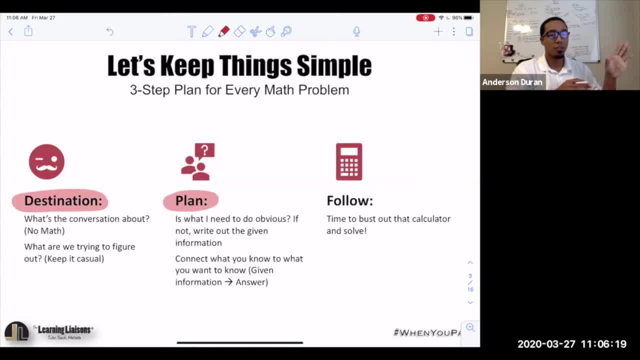 Because it's very complicated and very difficult to just start off by taking all of the information and hoping for the best. There's always extra information in the problem, So try not to use it. So, with that said, again, context in question- then make your math plan. 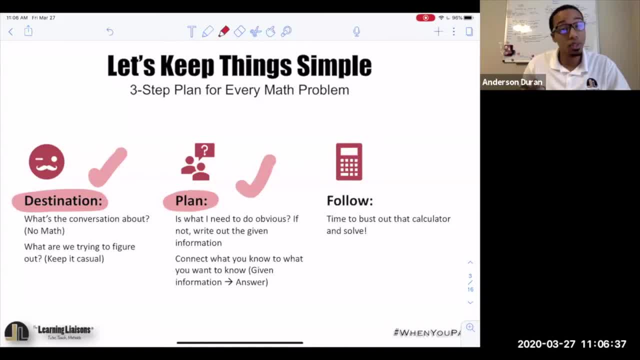 Start from where you are to where you need to go, And then only when you have your plan set up. that's when you're following your plan, That's when you start calculating. So, with that said, that's destination plan follow. 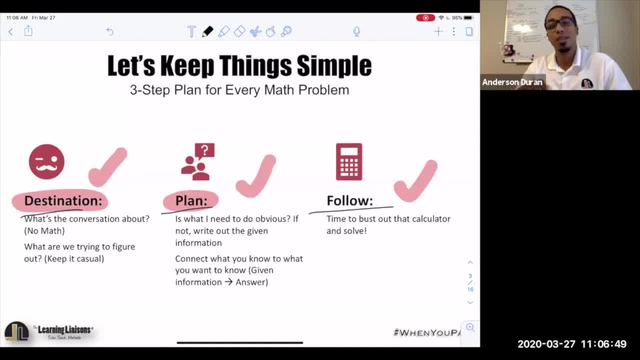 Who's ready to start implementing this plan in every single problem today? Give me a yes if you're ready, Right on, right on. All right, let's go ahead and start this math party, everybody. So here's the theme for today. 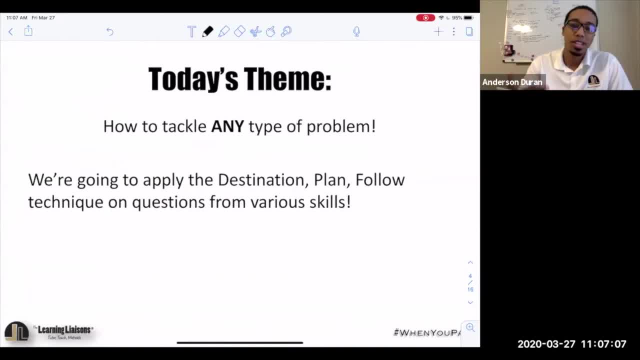 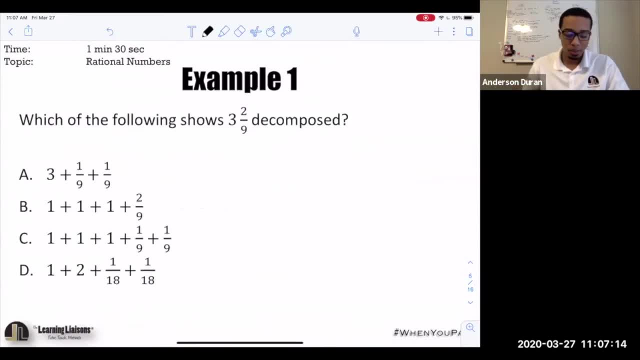 We're trying to tackle any math problem, Let's do it. So we're going to use destination plan follow on every single problem. Question number one: we've got a minute 30 seconds. Which of the following shows three and two ninths decomposed? 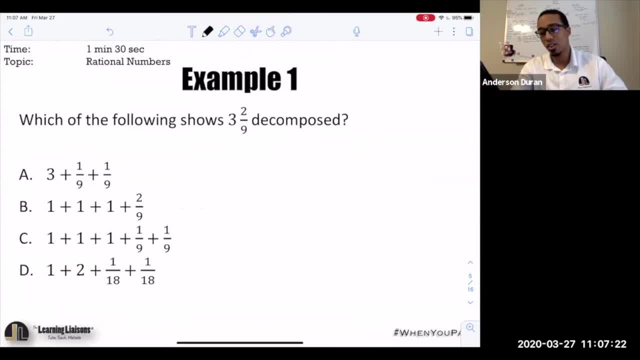 We have a minute 30. Starting the clock go And once you're ready, just type ready in the chat box. Do not, please, please, please, do not type in your answer into the chat box, Just type ready. All right, good job so far, everybody. 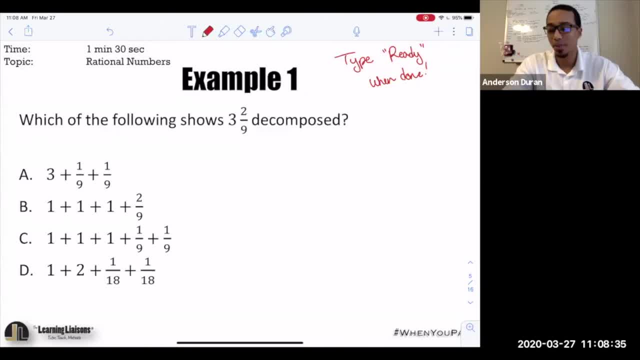 We've got about 20 seconds left, So get ready, We're ready to type your answer in. We still have 20 seconds. All right, five, four, three, two, What do we got Go? All right, so it looks like this question: 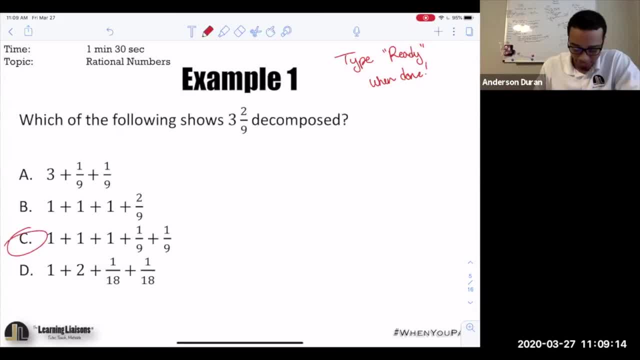 didn't really trick anybody. We all picked C and that is the correct answer. So this is a topic that's going to be both on the FTCE- elementary education math- as well as the praxis elementary math as well. So this is all about how to decompose fractions. 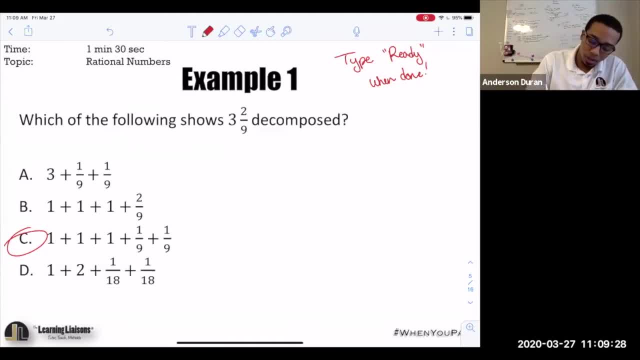 and numbers. So in this question here we have three and two ninths And we want to know. We want to know which one of these shows it decomposed. And when we think about how to decompose a number, especially a mixed number, here's how you do it. 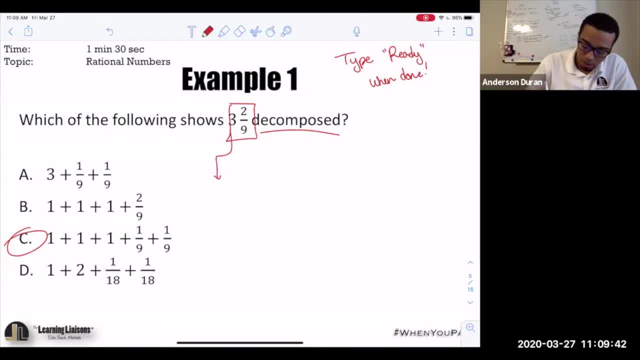 So the number itself. you want to break it down into its unit digits, So 1 plus 1 plus 1.. And with a fraction, you don't want to. you know the way that we would convert it and break it down. 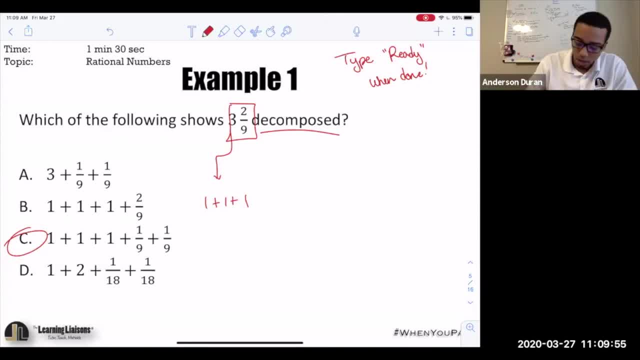 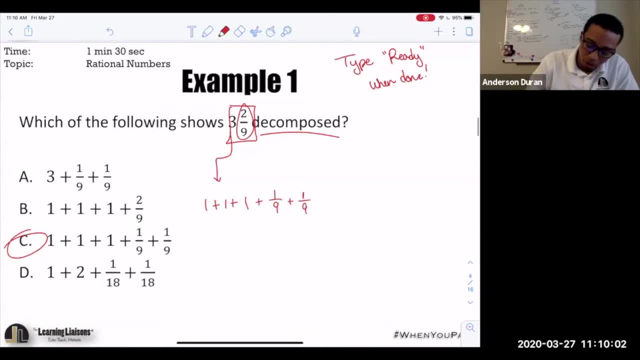 into unit digits. it's just called the unit fractions. So 2 over 9 would just be 1 over 9 and 1 over 9.. It's called the unit fraction and unit digits because it's just units, just ones, right there. 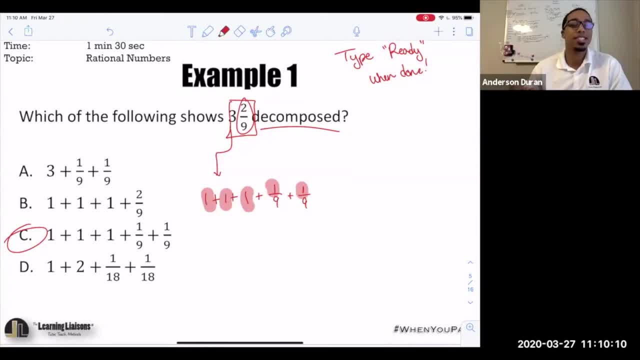 all the way through. So, with that said, that's why C is the answer. Is everybody cool with that one? This is probably the quickest explanation I've ever given in my life. You guys know me. I'm pretty notorious for spending like four or five. 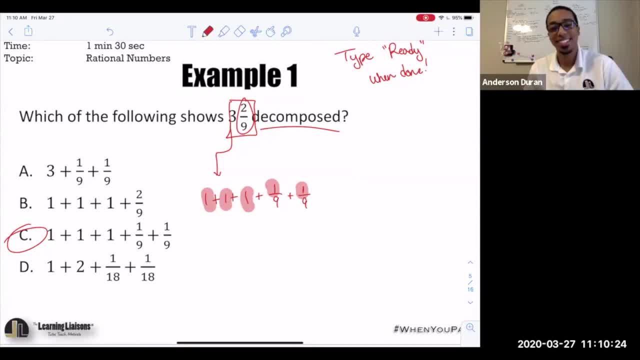 minutes on one problem, But this one's pretty straightforward, And so if you see a question Like this, hey, just look at it and say: thank you, burrito gods, grab it, boom, move on. All right, so we didn't really have. 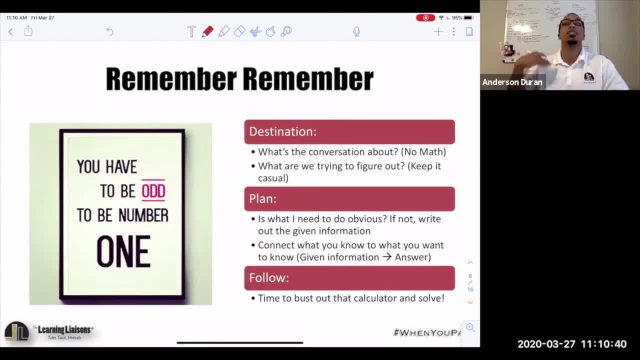 to use destination plan follow there because it was so intuitively obvious that a lot of us were just like: oh, I know what number decomposed means boom, But you actually did it without thinking about it. So we're applying destination plan follow on problems. 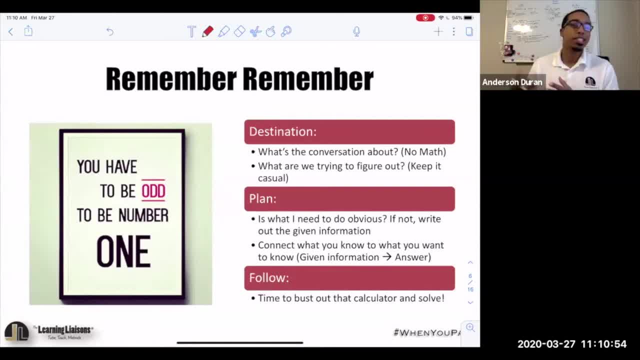 that we truly understand In that one destination was: OK, I see a fraction And I see that they're asking me to decompose it. Boom, my plan breaking down to the unit forms Then: follow that plan and do it. 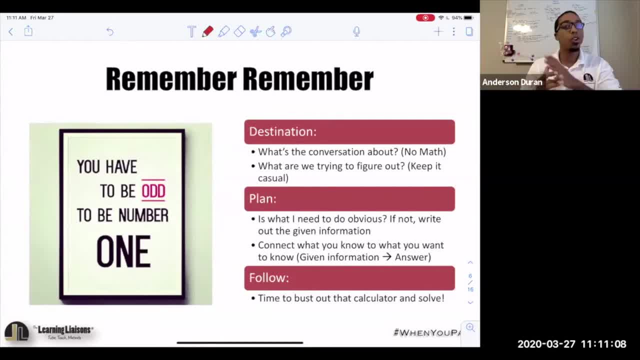 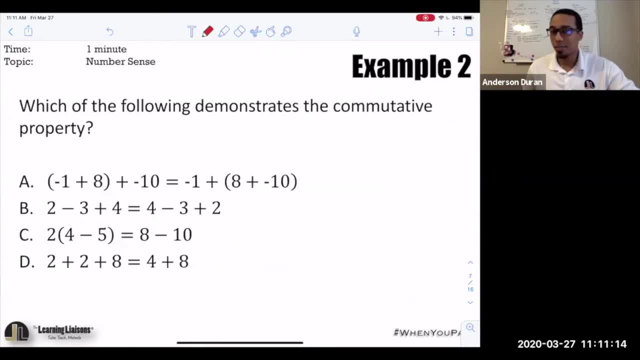 You just didn't think about it in the three steps like that. But the thing is you already did it in that process. So question number two: you got one minute. I know these problems are easy coming up, But get ready for the tougher ones coming on later. 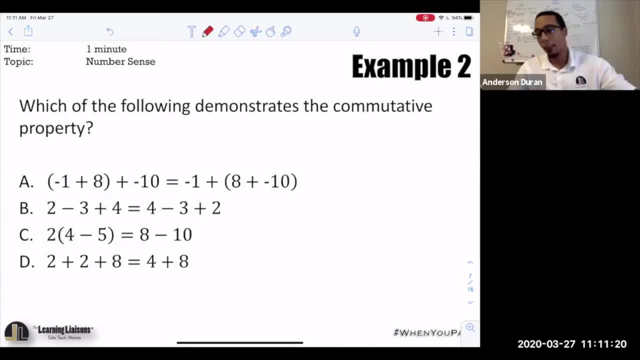 One minute go, All right. so we're going to go ahead and end this today And we have some time for questions. So you guys, are you ready to do this? We're sitting here and we're going to take a moment. 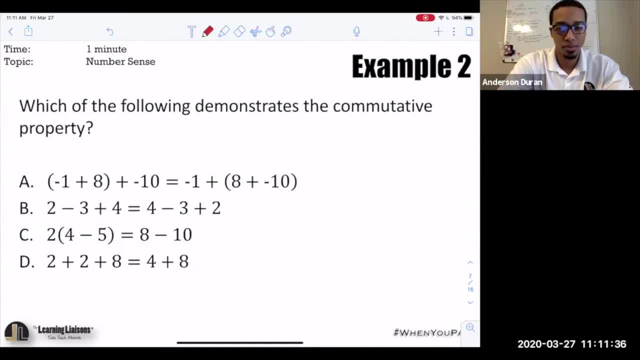 to collect a few questions, So we're going to go ahead and read the ones that we've been received. Let's do the first question. All right, As always, we're reading a question And there's a question on the screen here. 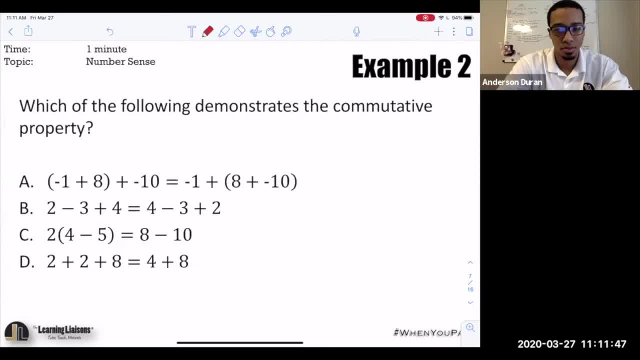 So you guys are going to pick a question One minute to go, OK, so here we go, Here we go, Let's just do this the second time. And continues. Here's the question. Let's start, Let's go. 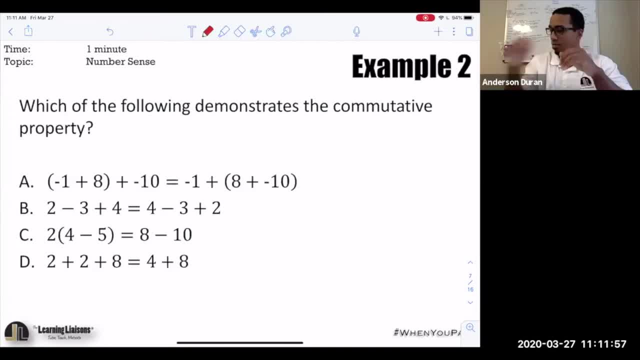 Let's go All right. All right, remember to type in ready when you're ready. and we have about 10 seconds left, but- and i only see about three- four people say that they were ready. oh, i'm gonna give us an extra 20 seconds here. 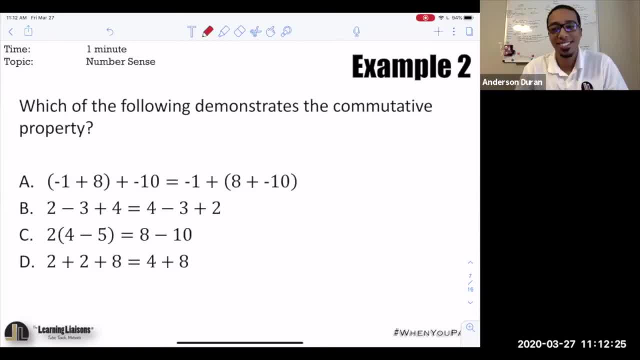 let's see if we can still figure it out. this one should be good. all right, that's 20 seconds. three, two, one. what do we got everybody? oh, we got some difference in opinions here. i got some differences in opinions, got some a's, some c's, some d's, some b's. all right, all right. so it looks like we're split on this one. 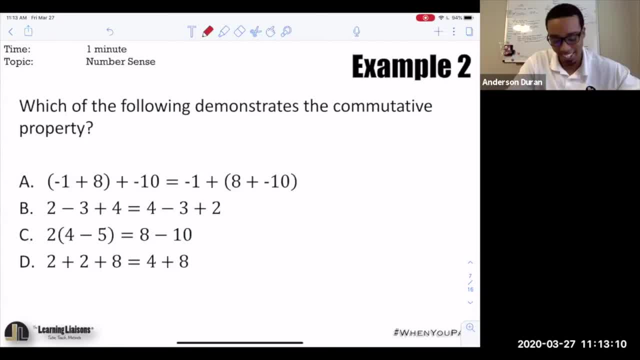 and i love disagreement, so let's go ahead and bring us all together here. so the problem states: which of the following demonstrates the commutative property? all right, so if i'm going by destination, plan follow. so i don't freak out, you know, by all of this math, here i'm reading it, i'm just saying: okay, which of the following? so instantly: 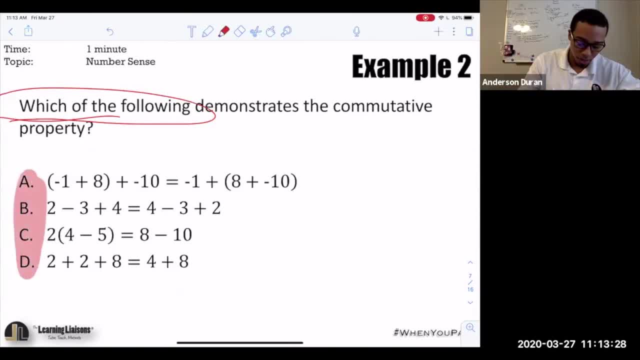 when i read a question like that that says which of the following you know you have to use the answer choices you have to, and then demonstrates the commutative property, all right. so whenever i read a word like commutative property, i always think of the other properties as well. so everybody. 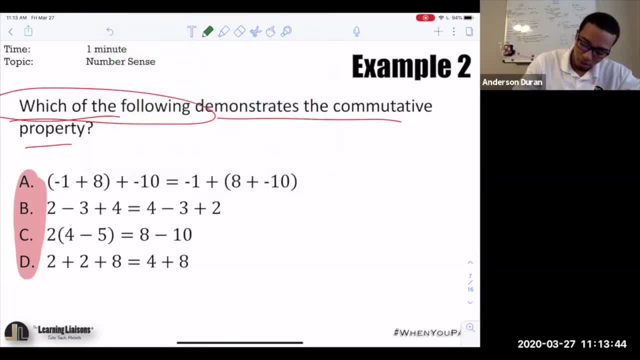 go ahead and help me out. what are all of the properties that we should know? the first one in commutative. what are the other properties? right anicia, distributive- we got one there- associative right, mm-hmm. and those are the three that we really need to know for this test. i saw the 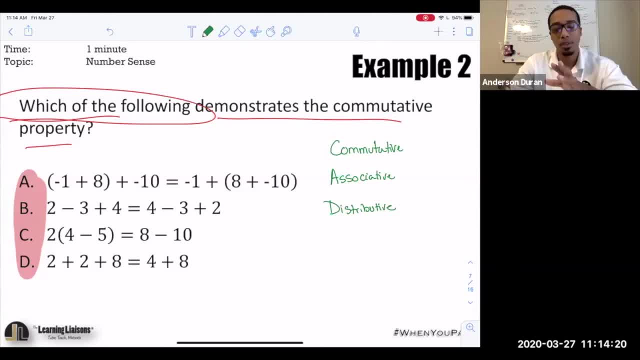 um, the identities. uh, identities are just a set of? uh, facts, not a set of like mechanisms, so it's a little different. um, so let's go ahead and just talk about these three right here, because these are the ones that we want to know. so, commutative property: think of the word communicate, communicate, communicate. 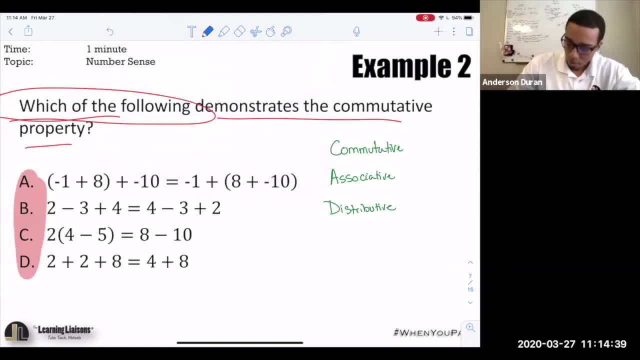 try to think of those in the same way, so i'm going to go ahead and write that here. they can communicate in different ways. associative- think about it like this: well, you can associate in different ways. and then distributive- well, think of the word distribute. very straightforward, very straightforward with these three terms. now, when we look at a, b, c and d, 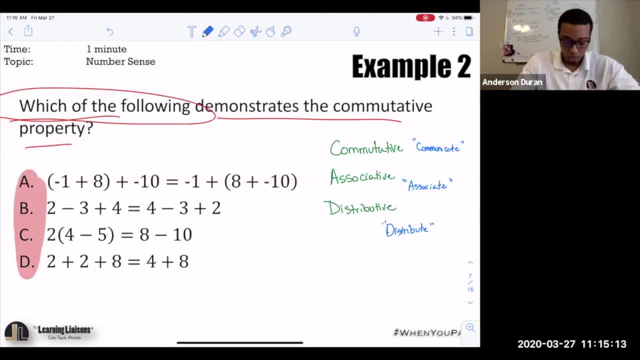 let's go ahead and pick apart which properties these are. so a we have to think about these three. we have in a parentheses, negative one plus eight, and then we're adding a negative 10 beyond it. now, on the right side of the equal sign, what we see? we have the negative one still in the same place, the eight still in the same. 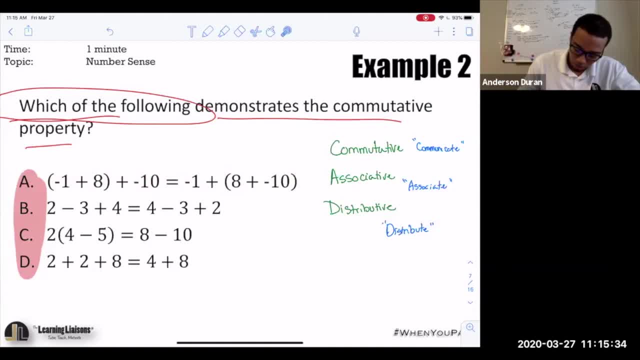 place being second and the negative 10 still being there in the third. the only difference is that the parentheses group the negative one and eight together and then moved to group the eight and negative 10. so essentially, the parentheses are the same place and the negative 10 are the. 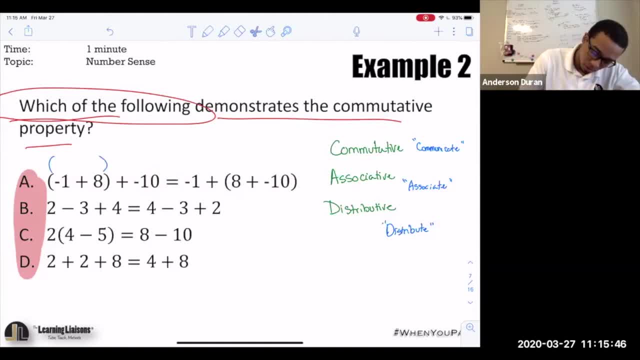 parentheses just moved from the left here to right here. so when that happens, what are we doing here? are we associating two numbers in a different way? are two numbers communicating in different ways? are they distributing something to the numbers? what are we seeing here? and so, to get this down, 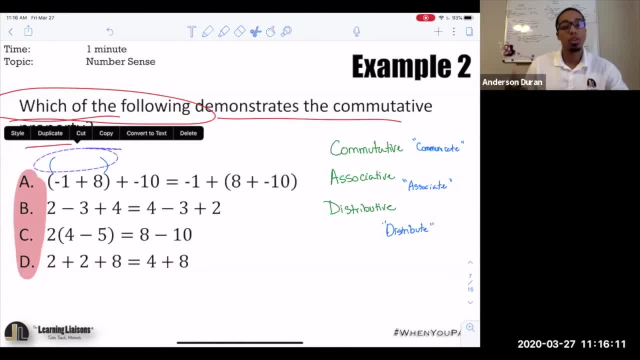 and know this definition like the back of our hands. what's really going on here is that we are associating a parentheses with different numbers. we're associating the parentheses with different numbers. so this is the associative property. does everybody agree with what i just said? all right, awesome. so yeah, that's what's going on if we associate two different. 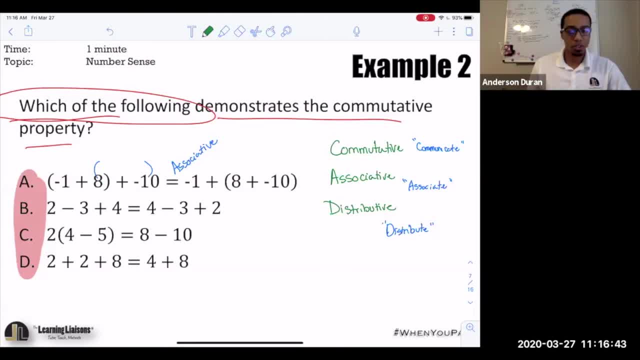 numbers and it doesn't do anything. we're associating two different numbers and we're associating two parentheses and it doesn't change the outcome of the equation or the expression. yep, that's associated, because you can associate the parentheses and still keep the same answer. now, b, again i'm. 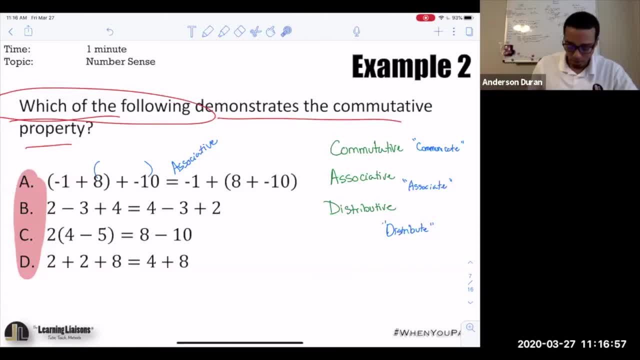 just going to analyze it fairly quickly. i'm going a little slow here to break it all down. but on test a, you want to be quick. here we have 2-3 plus four. what changes? four minus 3 plus two. so it looks like the two and the four were swapped. then negative three or the minus three crosses it in check. 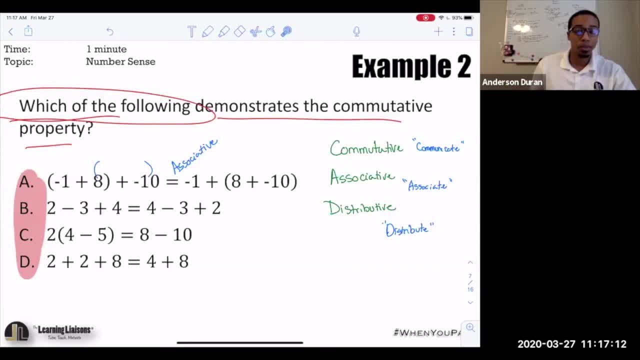 them all down on here and here. Okay, all right, now we're going to work this way. we're gonna ours a little bit too slow. three stays in the middle. So, with that said, it looks like they're saying, hey, it doesn't matter. 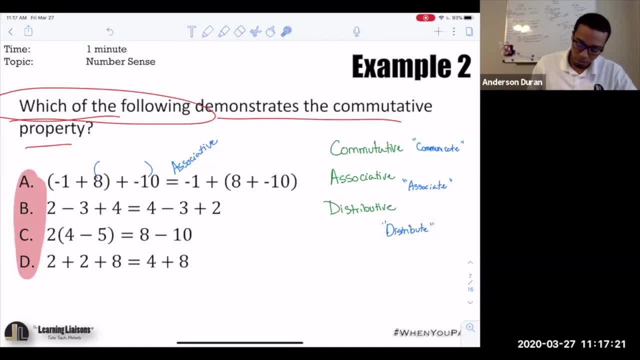 what the order is. We can have two, then minus three, then plus four, or we can communicate it a different way and say four, then minus three, then plus two. They're both going to be the same result. So notice that we can communicate the numbers in different ways and still get the same. 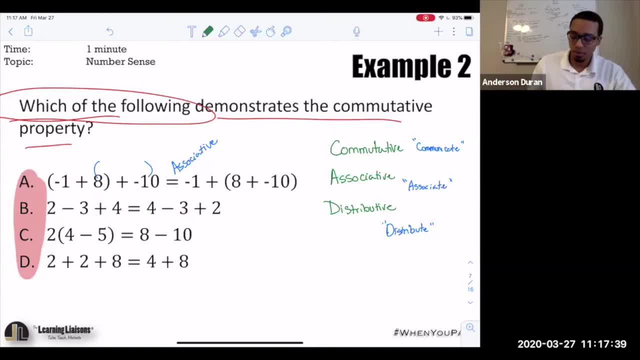 result. So this would be which property? everybody. I want you to type it out because the more you talk about it, the more you type about it. I know it's a little inconvenient to type it all out, but I want you guys to do it because, again, the more you talk about it, the faster. 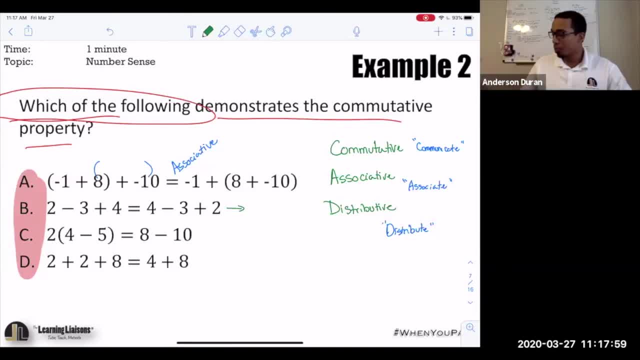 you get better. Seriously, something as simple as repeating it and the definition or typing it out really does help. Yep, it's commutative, Exactly, And that's why B would be the correct answer here. If we look at C, what's happening here? It looks like we go from two multiplied by four minus five. 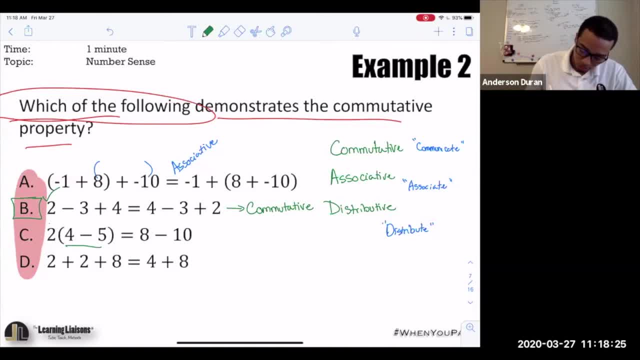 and we ended up with eight minus 10.. What ended up happening here was that the two was distributed through the four and negative five, which gives us the eight minus 10.. And that's the distributive property. So what the distributive property says is that if you have a number being 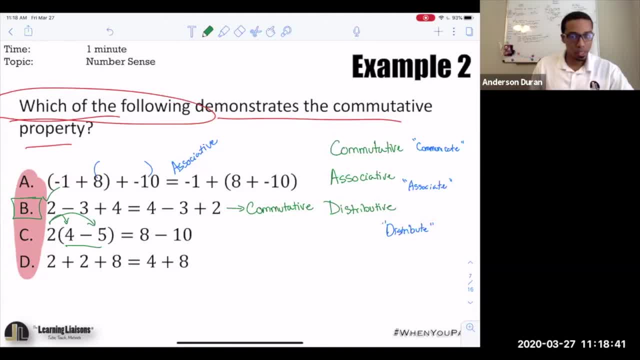 multiplied to a group or parentheses, then you can distribute or multiply that coefficient onto everything inside and still preserve that true statement or still keep the equation true. The last one here we have: two plus two plus eight turns into four plus eight. This is just. 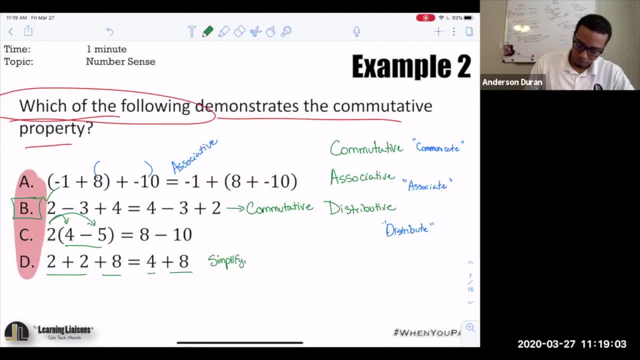 simplifying. All right, This is just simplifying. This is just grabbing your like terms and simplifying your like terms, or adding your like terms or subtracting your like terms. Whichever way you see it, you're just simplifying like terms. That's all it is. So, with that said, how are we feeling about? 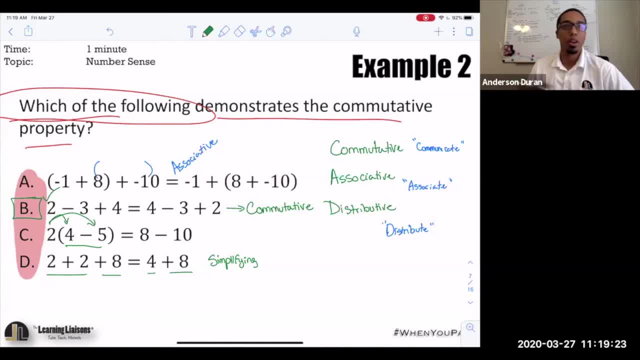 example number two: Where were we before and do we feel better now? or do we still have the same level of understanding as we did before? Sweet, Because I know a lot of us have seen these terms before. It's obvious: We've all been in grade. 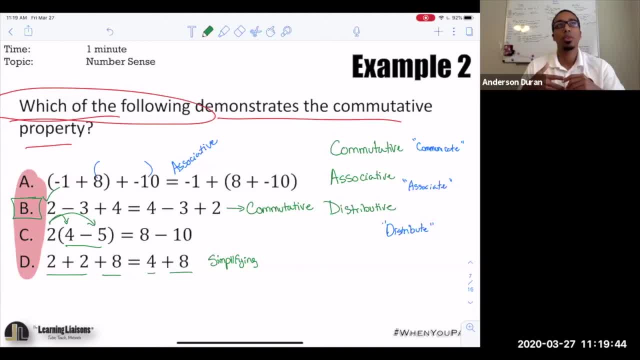 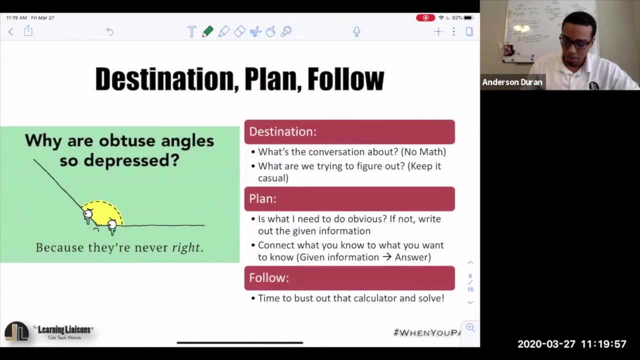 school. But the thing is, the question is not whether we recognize it, It's more so about hey, can you talk about this? Can you explain this well enough to be able to really see any type of problem about it? So let's go ahead and recap again. Destination plan follow. 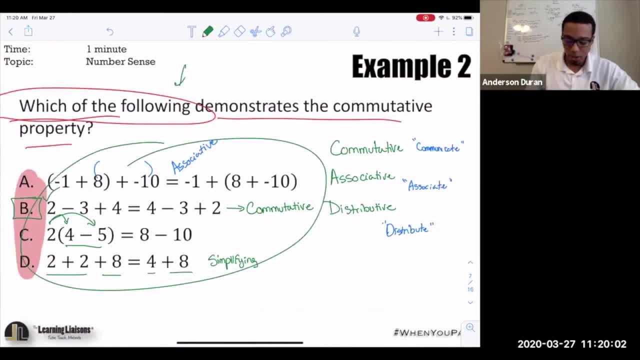 I started off by saying, hey, which of the following Got to use my answer choices? That helps me not freak out, Because if I look at things like this I'm like, oh, what the heck, What's going on. But when I read which of the following, oh, I just have to analyze something. 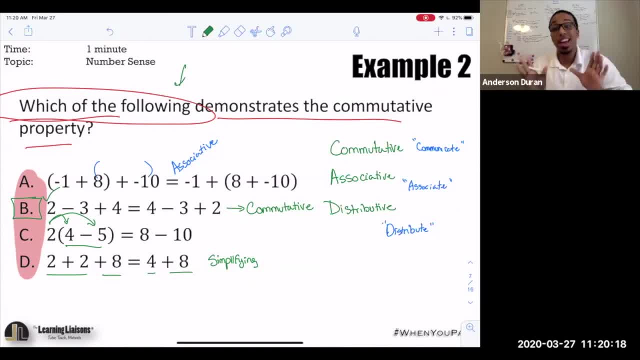 about these problems or these equations, And that helps me stay a lot calmer than I would have if I would have just said: oh God, all of these equations I'm done. And then just read: demonstrates commentative property. So I went through it. 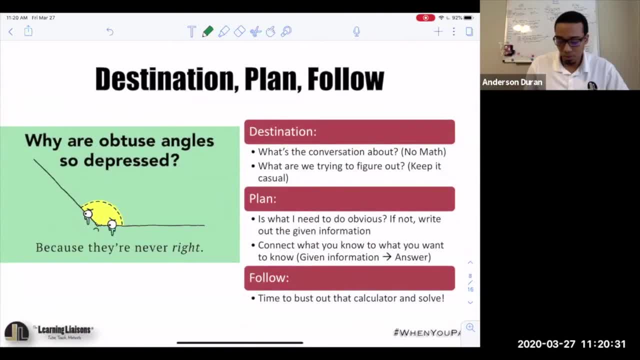 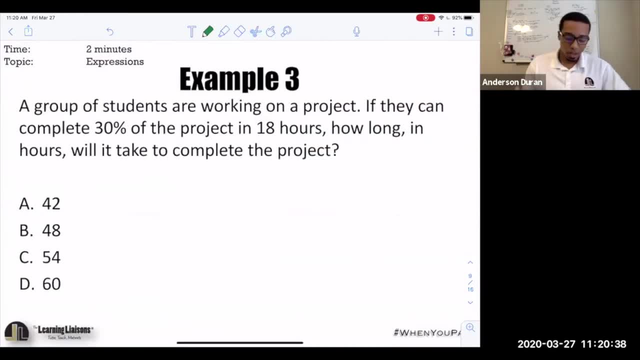 Found which one it was And I'm done. So there it is again. Destination plan. follow Question number three: Diving right in Two minutes here, This is not expression, Sorry about that, This is percent, But here we go, Two minutes. I'm going to go ahead and start the timer right now. Three, two, one and go. 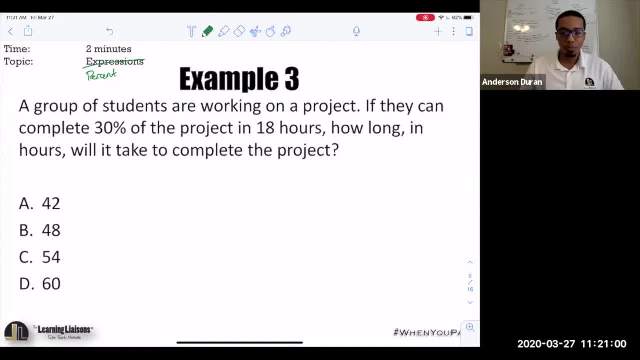 Diving right in Two minutes here: Three, two, one and go And remember everybody. once you have your answer, once you're ready, just type you're ready in the chat box. That way we can make sure no one sees any answers. 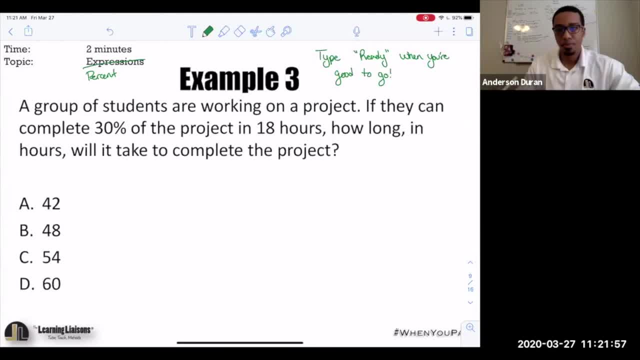 Diving right in Two minutes here: Three, two, one and go. You've got about 40 seconds here, Just about 40 seconds. Diving right in Two minutes here: Three, two, one and go. 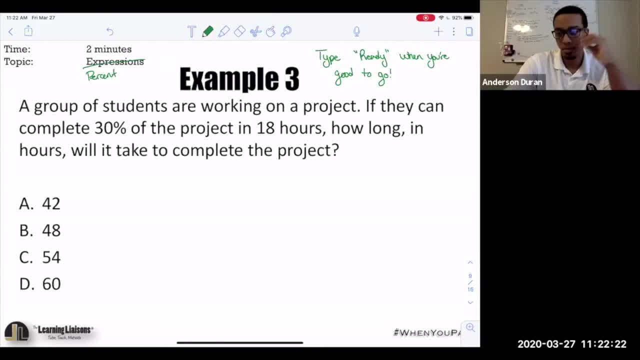 Diving right in: Two minutes here: Three, two, one and go. We have 10 seconds here: Five, four, three, two and one. What do we got? All right, we got some Ds, we got some Cs. 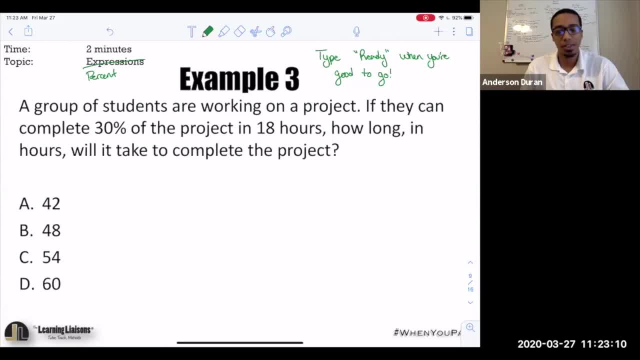 All right. so no As or Bs, strictly Ds and Cs. Okay, Okay, We got an A now. okay, All right, looks like a lot of A's. All right, A lot of folks here. all right, So the majority of us agree that it's either a, C or D, All right. 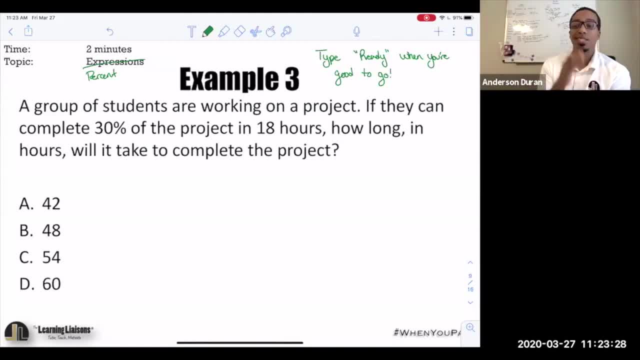 so let's go ahead and go over it. but first and foremost, as always, destination plan follow All right. so let's go ahead and run through it nice and smoothly. So remember when you read the problem the first time, you don't want to focus on the math. 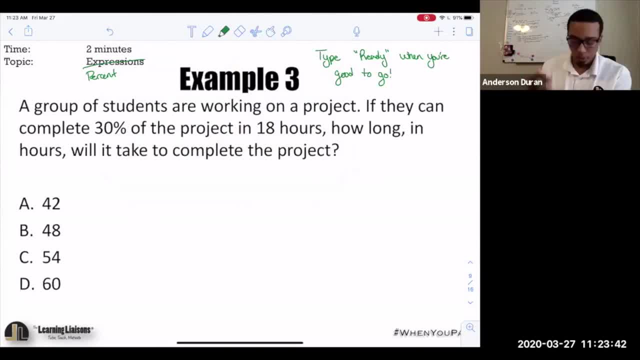 You just want to focus on the story, what you can recognize. So a group of students are working on a project. All right, that's pretty self-explanatory, Cool. So a student's working on a project. If they can complete this much of the project in this much time. 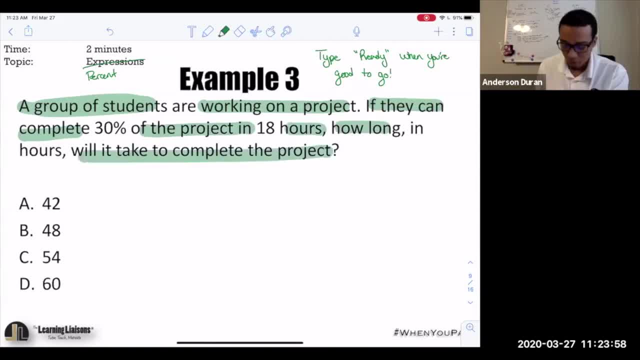 how long will it take them to complete the project? So the story destination again: only focus on what you can immediately recognize and talk about. We're talking about a couple of kids that are working on a project. They've completed some piece of it after a certain amount of time. 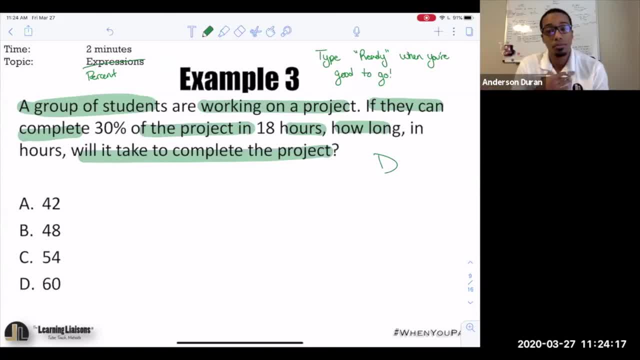 and we just want to know how long it's going to take them to complete the whole thing. So, with that said, we're going to go ahead and get started With that first initial step there with destination. did everybody understand that again? 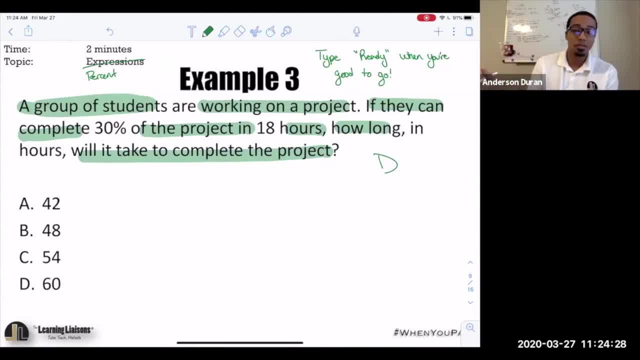 all, we're just talking about a group of kids working on a project. They've completed some of it so far. We just want to know how much time it's going to take them. Sweet, Perfect, That's where we want to start here. 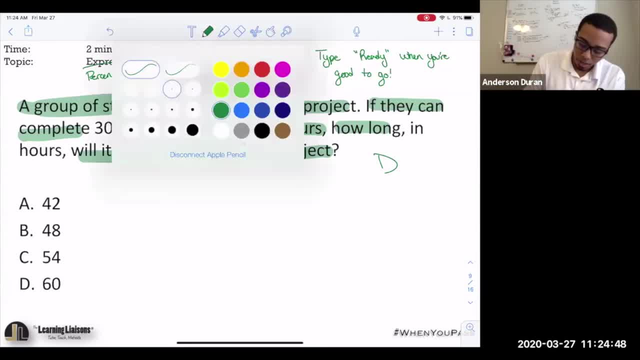 Again, we just want to figure out how long it's going to take them to complete the whole thing. So we're going to go ahead and get started, So we're going to figure out how long it's going to take them to complete that project. 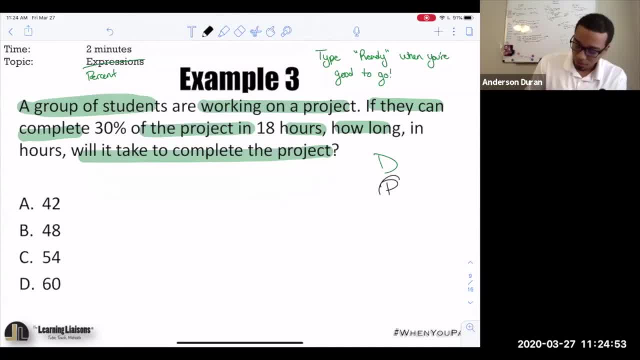 So when I go into the planning step or the planning phase here, the first thing I want to do is write out my answer- Not the exact number, obviously, but the units or whatever we're discussing. So if they're saying, how long will it take to complete the project? 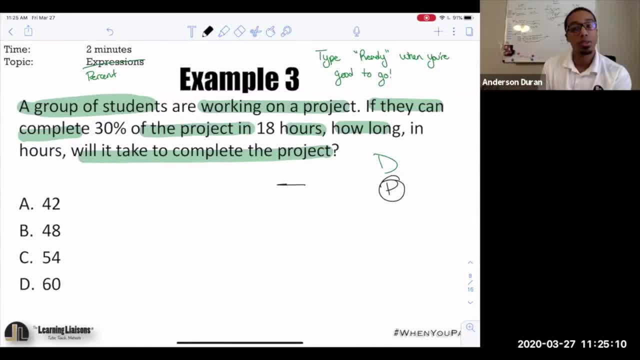 I'll say blank what? What are the units that we're using, for how long it's going to take? Okay, What are my units here? So if I'm writing my answer blank what? Because here it would be 42 blank, 48 blank, 54 blank, 60 blank. 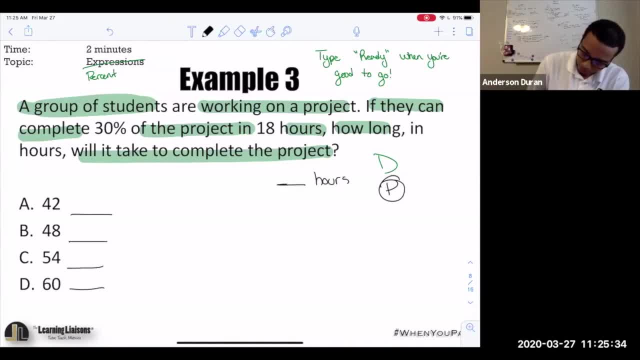 Yep, exactly Blank hours, Exactly Blank hours. And if we really wanted to fill in that blank, here's my recommendation: When you write variables from now moving forward, here's what I recommend you do: Only use letters that pertain to what you're solving for. 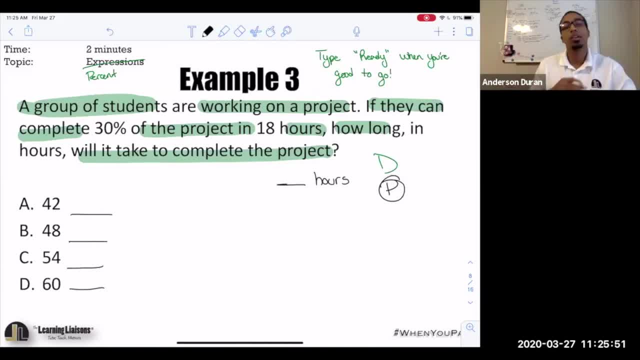 Don't always use X. I know everybody has a really bad habit of always using X. The thing is sure, you're perfectly allowed to do that, but the thing is you want to build a further connection with the problem that really shows that you understand. 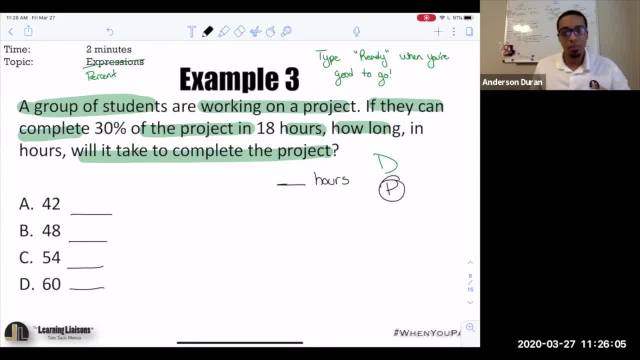 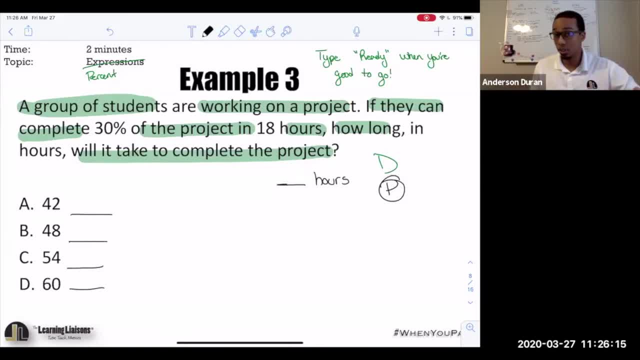 So, just like learning any other language, the more you try it intentionally, the better you get and the faster you get at it. So that has something to do with it. So we're looking for H hours Now in our plan. let's go ahead and start writing some of the given information. 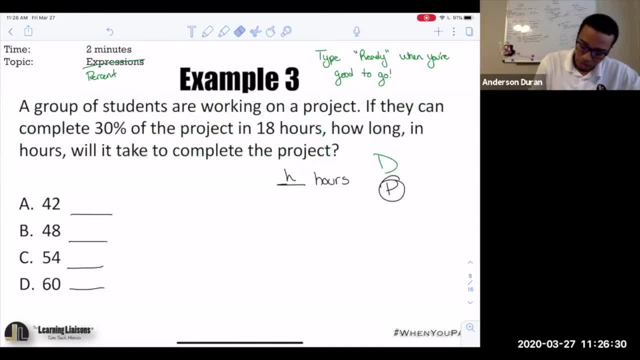 So let me erase what I wrote here, And now let's go ahead. boom, 30% of the project in 18 hours. That's a pretty important piece of information, Also how long in hours, which I already have here. 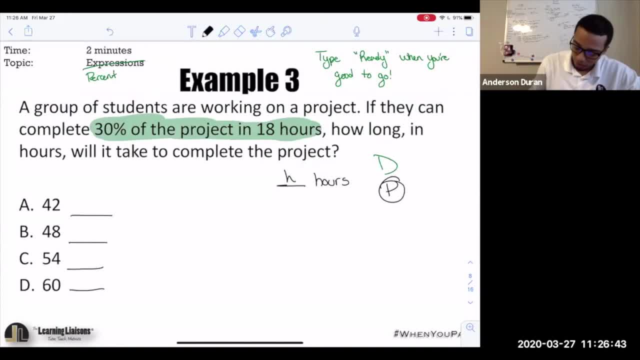 So that's good. That's really what I have. All I have is 30% complete in 18 hours, All right. So for those of us who believe that we got it right, go ahead, type out the equation that you probably maybe set up to solve this. 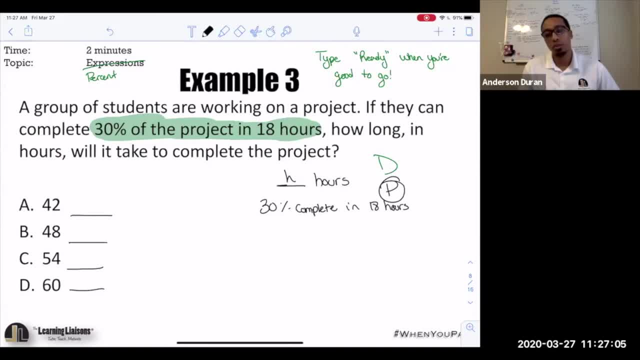 Or if you didn't set up an equation, you know what calculation did you do to get it done, So I'll give us a second. Give us a second to type that out. So how did we go about it in our way? 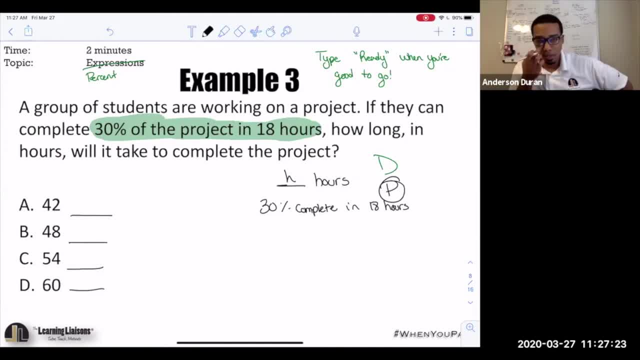 18 divided by 30,, 0.3 times 18, percent of is 100, cross, multiply and divide. Ah, okay, okay, okay, I like this. now I like this. So a lot of us use a couple of different ways, but what I did recognize is that a couple 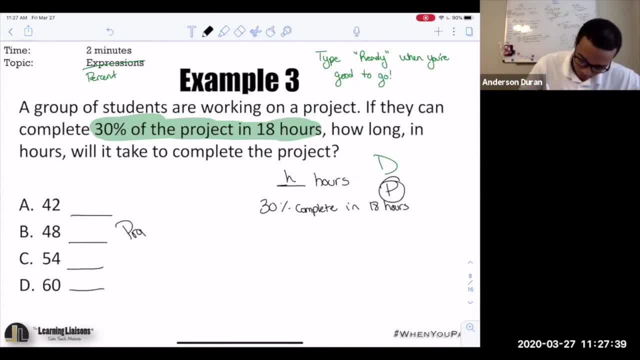 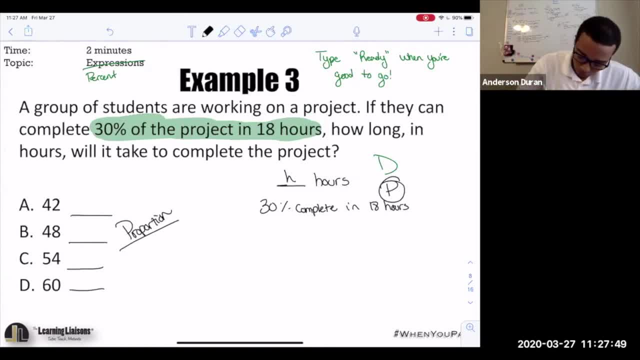 compared in the same ways. So again, a proportion where the same things are being compared in the same ways. So if we have 30% complete in 18 hours, we're going to have 100% complete in how many hours, guys? 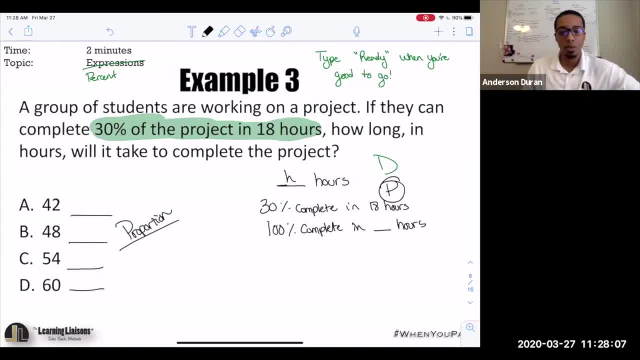 What's that? what should I fill in the blank with? That's right, Sedaria, thank you. thank you with H hours I'm talking about, like with what we know so far, not the answer, guys. So 30% complete in 18 hours. no worries, you're good. 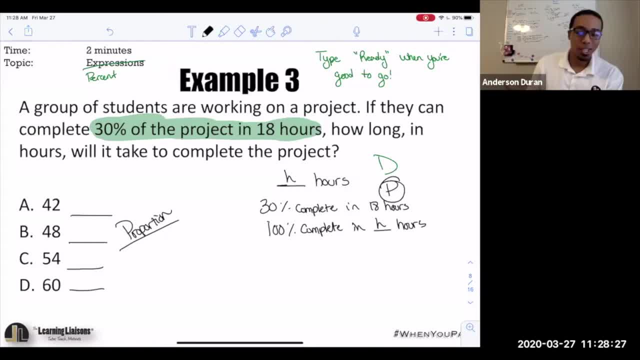 30% complete in 18 hours. 100% complete in H hours. So there we are, And what we want to do here is set up a proportion. So again, we want to compare the same items in the same way So we can set it up as 30% out of 100% equals 18 hours out of H hours. 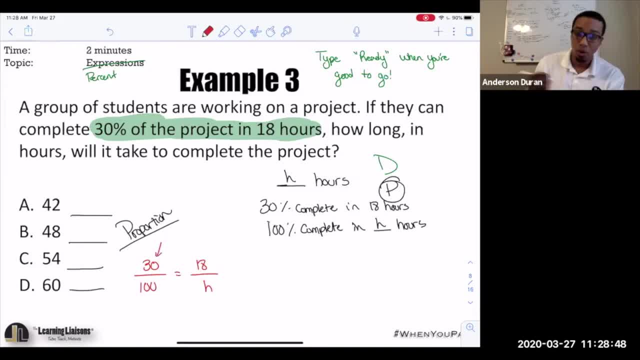 The reason this is okay is because 30 represents 30% of the work and 18 represents 30% of the work just in the form of hours. 100 is the percent of the total work. This is the hours of total work. 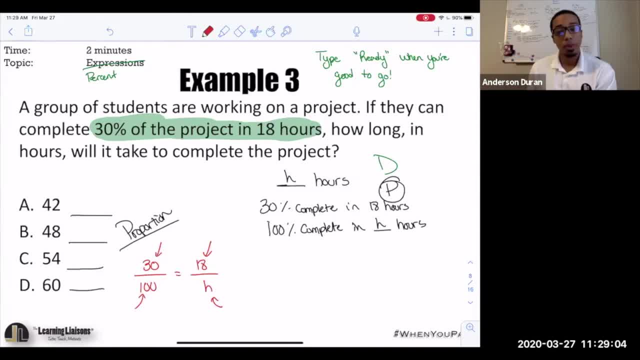 So notice, on the left side We're just comparing percents. on the right side, we're comparing hours. but they're being compared in the same way, And that's good. That's all we need. Others may have set it up in the following way, and this is still correct as well. 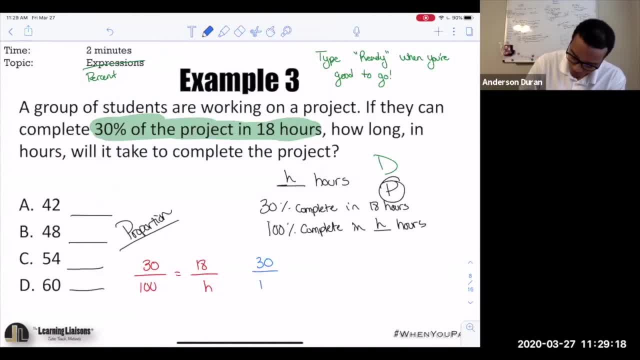 Some of us may have set it up as 30 over 18 equals, 100 over H. Another way could have been: Okay, We could have done H over 100 equals and then we could have said 18 over 30. That's another way to do it. 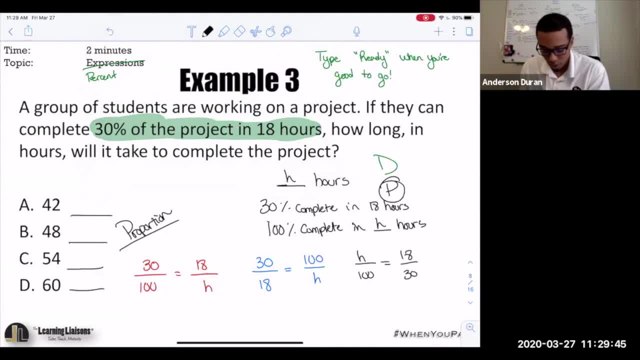 So those are three of the more common ways. I think there's one more that we can do, but I'm going to leave it right there. But the thing is, these are all correct. All you have to do is compare the same items in the same way. 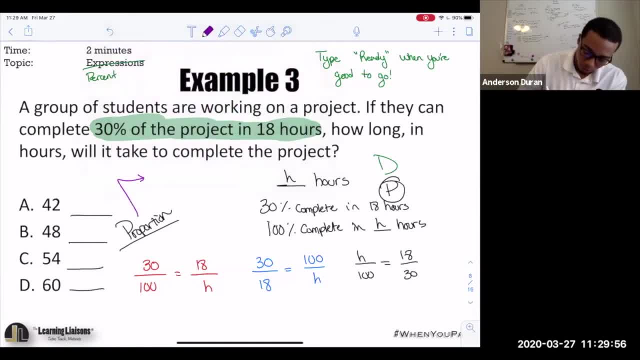 So I'm going to write this down for everybody, or anybody who has a struggle with proportions. So compare The same items in the same way And you're good to go. So again: percent, percent, total, hours, hours, total, all good. 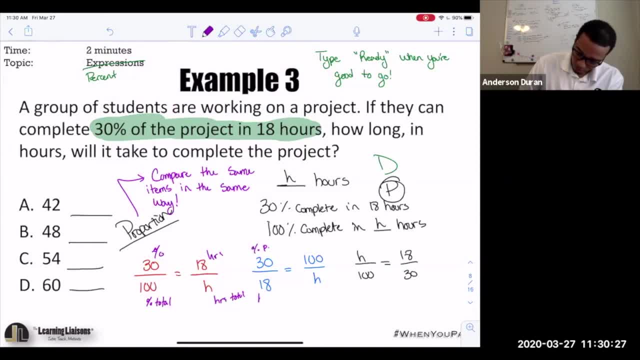 Percent Part Hours, Part Hours Hours. Part Hours, Part Hours, Part. Now we have percent total, Hours total. So again, just compare the same items in the same way and you're good. So, with that said, who's ready to just knock this out right now? 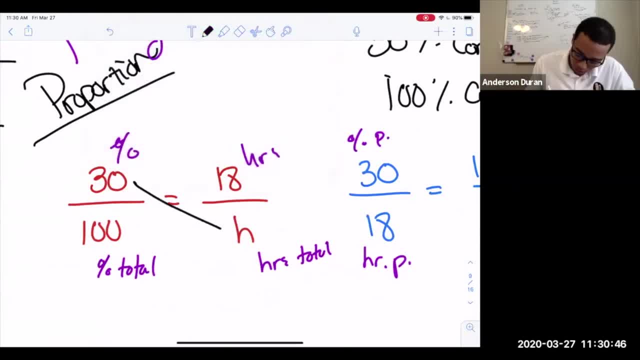 What do we get when we get the 30 and H together when we cross multiply? But what do we get when we have 100 multiplied by 18? What do we get everybody? Help me out, All right, Correct 1,800.. 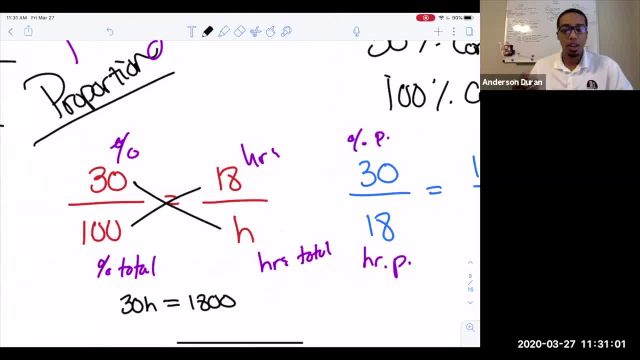 Yep, From here. the only thing we have to do now is just divide both sides by 30 and we're set. Because what's going to happen on my left side? 30 is canceled out, leaving us with h equals 60.. 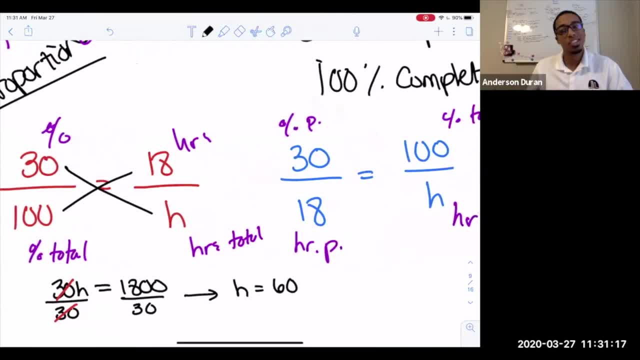 Remember to answer it in the context of the question. Sixty what everybody Make the connection with the problem. Sixty what Boom First goes to Kamawari, Perfect Boom, Sixty hours. Sixty hours is again. 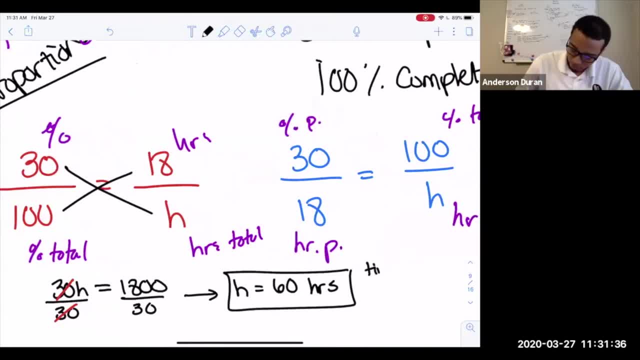 how long it'll take to complete the project. Again, it's super important that, once we're done that, when we're practicing, especially that we're not just: oh, there's the number, plug it in, that's my choice and move on. 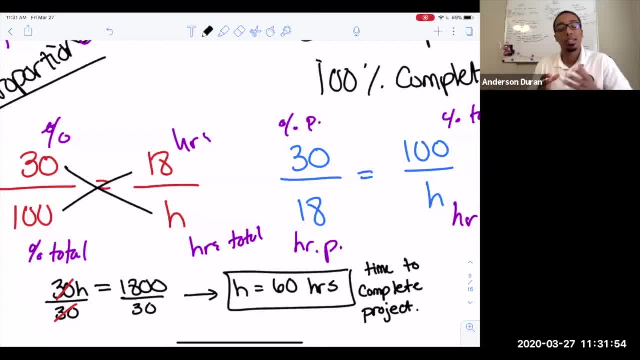 We don't want to do that. What we really want to do is again solve the problem, get the number and then relay the number back to yourself. I got 60. I was trying to find the number of hours it'll take to complete this total project. 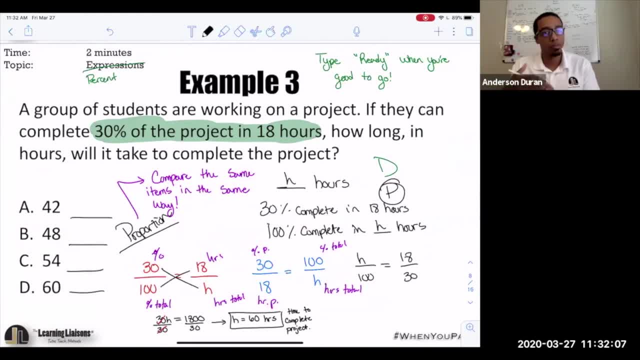 Sixty represents 60 hours to complete it all, with all the group of students working together. Boom, You've tied it all back together along with the story and you've made a more meaningful connection with the problem, and it's more than just circling the right answer, moving on. 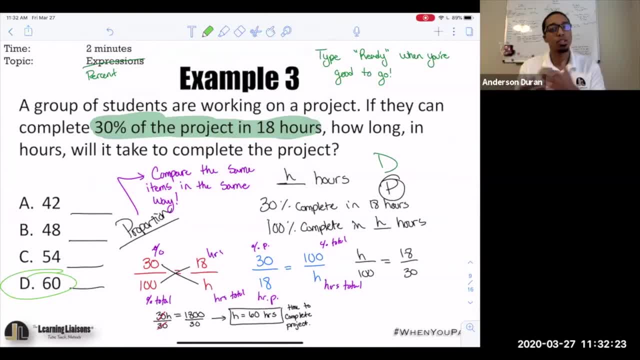 Because you reflected on it. you see what you did right. you see how you can apply it to the next problem and, with more problems under your belt, you'll start doing it automatically, as opposed to having to really give that effort every single time. 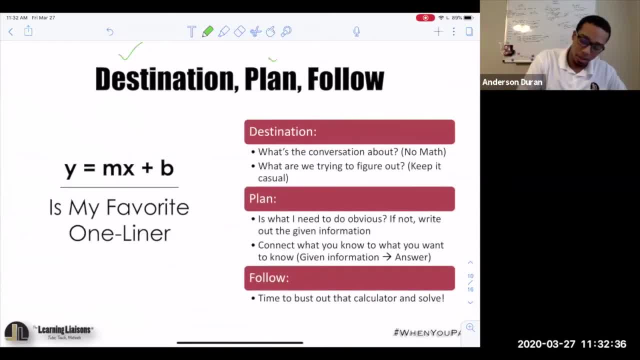 With that said, who's liking destination plan follows so far, Because, notice, we're not calculating at all until the very end. Who likes this strategy so far? Is it helping anybody? If so, how is it helping you Now? what were you doing before that made you struggle? 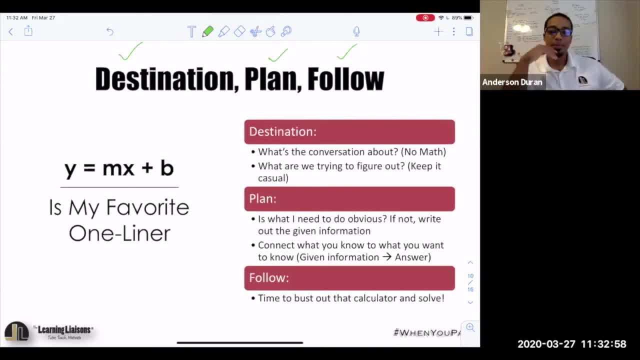 I want some real answers here. I just realized we're live on Facebook too, so I'll be relaying some of these answers to the folks. I'm not going to say any names though. so you're good, But what were we doing before learning destination plan follow. 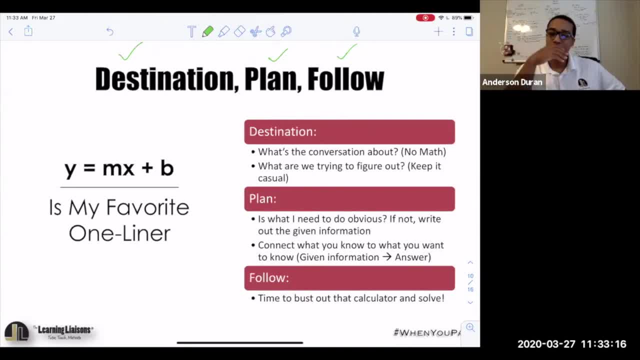 and how does this strategy help you? now That's my question Starting to take root with a few more problems. you're going to grasp it. I love that Helpful with organizing the problem clearly and not making common mistakes. That's exactly why we do it. 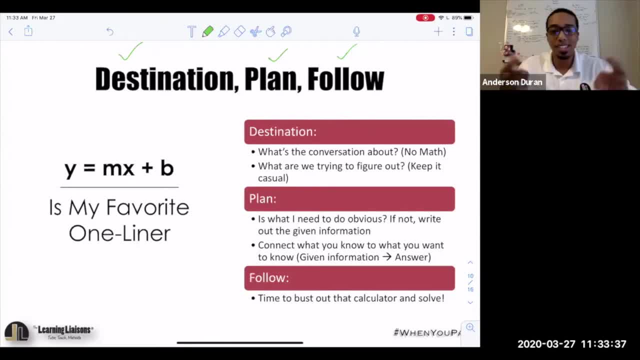 Determining when to use proportions or other math concepts exactly. It's a good visual. It helps you slow down a bit and understand what you're doing. I was just jumping to the math and going and my answer. it didn't always make sense. 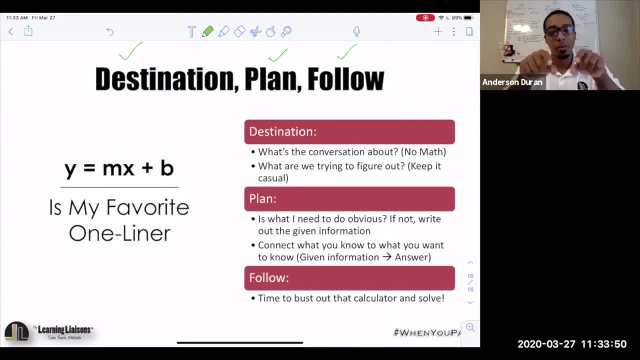 Girl, that is exactly what I'm talking about, Because the thing is again: how many of us have started a word problem and the first thing we did was to start grabbing our calculator, mash some buttons together and really just hope for the best? 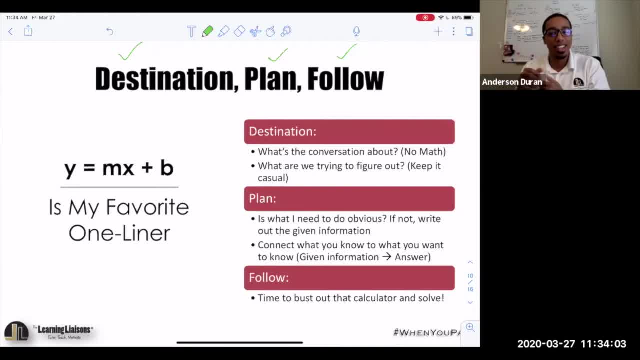 Prank the burrito gods or singing Hail Mary or something like that. Then if you see a number that shows up in your calculator, great. But the thing is, there's no methodology behind that, There's no confirmation behind that, There's no confidence behind that. 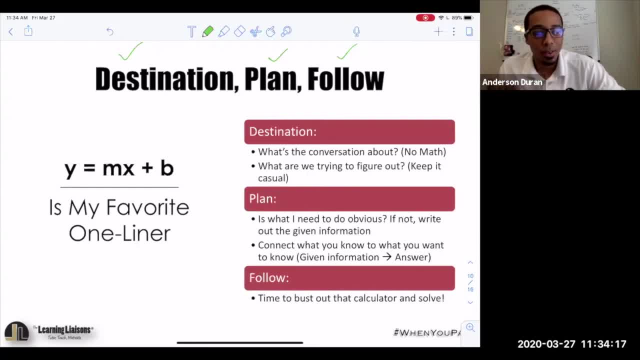 There's no teaching How to be confident, So some more. It's a new strategy to me and is making the process easier to understand by piecemealing. I love it. I personally was just ready and trying my best to answer questions. 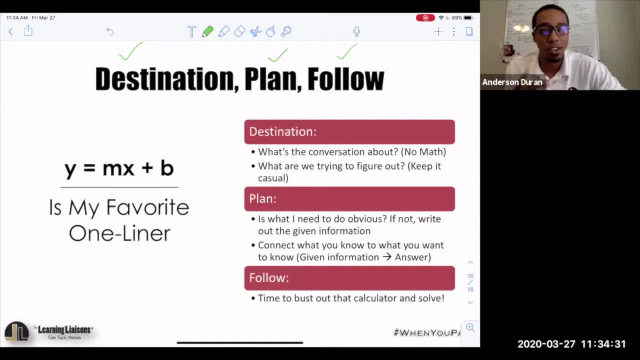 Now I'm really trying to not read too much into it. Exactly Keeping it simple, Starting simple. I can see the whole picture now. Before I used to freak out when, and then it cuts off when I see all the numbers. Right. 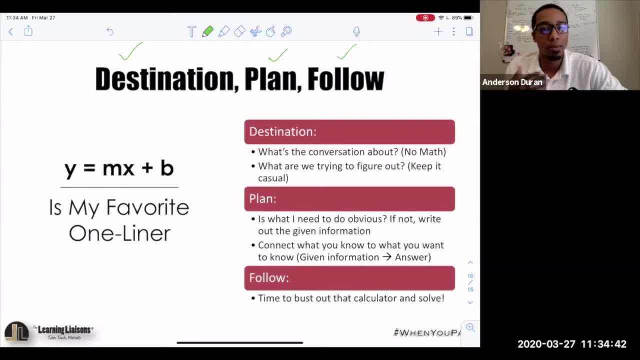 Setting up the problem is my issue. Therefore, helpful Learning how to set up the problem. There we go On the fence. to be honest, when I looked at the FTCE bootcamp, the instructor told me to look at the answers first and remove outliers. 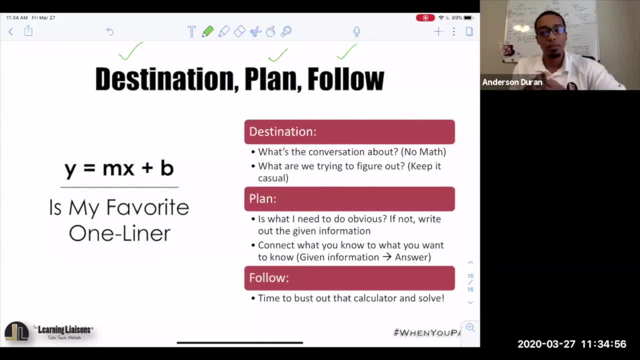 Removing outliers is definitely a great strategy to use With the math. here's the thing. When it comes to the reading writing essay, you can learn the strategies- the simple strategies behind it and apply those only and still pass. But when it comes to the math, the majority of this test is going to bank on your ability. 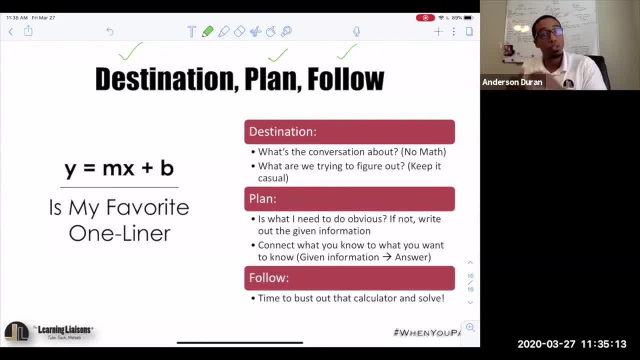 Bank on your ability to understand the math itself. So that strategy still works. but you want to apply that strategy when this first strategy does not work, So when you don't know the math and when you don't know how to break the problem down. 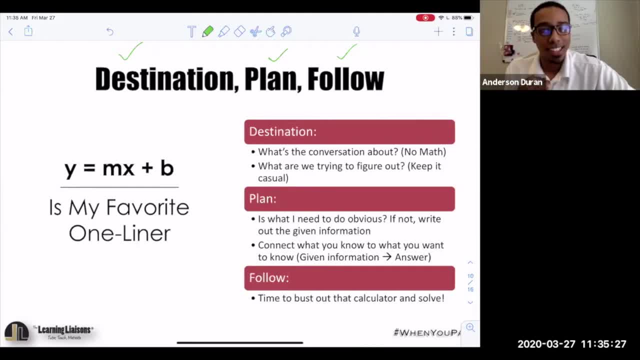 It helps me really understand what the problem is asking. I love it. It helps you think first before the strategy. just look for the numbers. It's helping me map out the problem all the way to start to finish. I love it. Mental math and elimination. 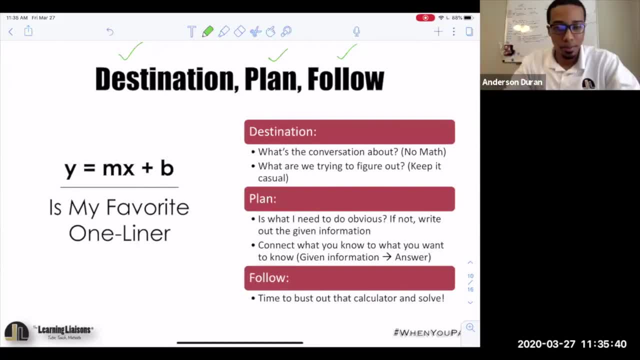 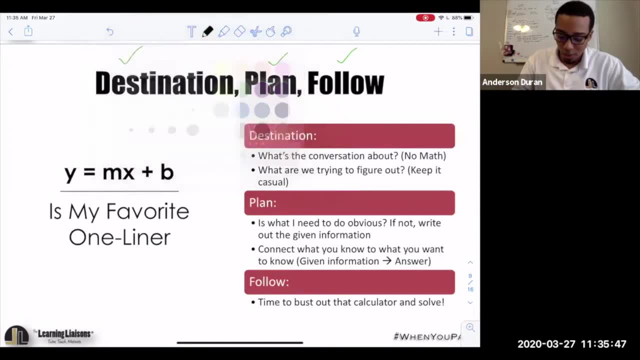 But no formula for change. Okay, Let's go ahead and check some balances, Trying to analyze all parts of the questions. This is great. So we're all growing in some way shape or form here, So let's go ahead and dive right in. 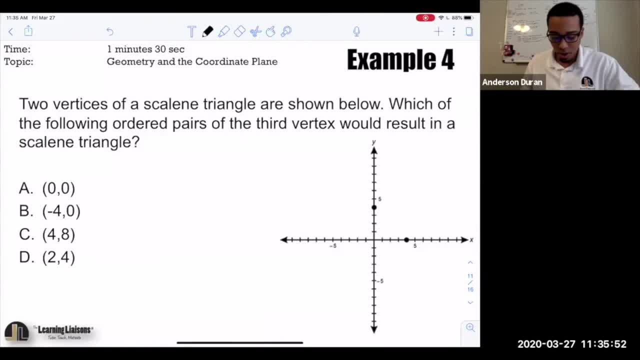 Question number four: a minute 30 seconds. this one's on geometry, starting the timer in three, two, one go. Okay, So you did that. Okay, You can do it. Okay, So you'll be doing this. 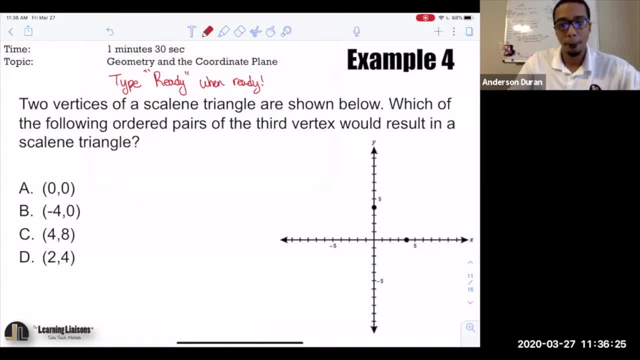 You'll be doing this. You're going to do this Now. we're going to do two more. We're going to do two more. One is this: Now, we're going to do this. Okay, I want you to do this. 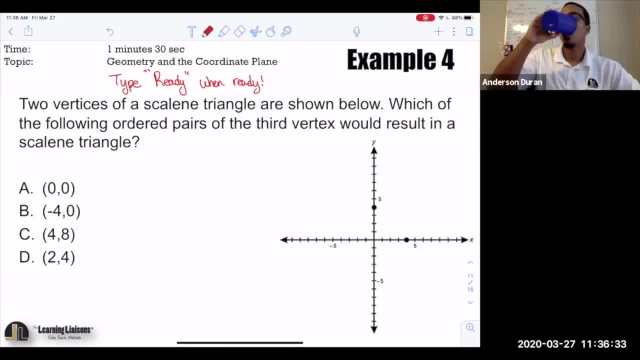 So this is your score. Now let's do your score. Okay, Three, two, one go. Okay, Excellent, Ooh, All right, halfway done here. We got 45 seconds left, 45 left. All right, here we go. 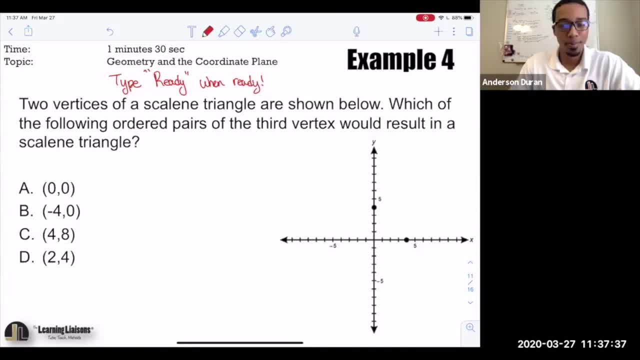 Three, two, one answer. What do we got? I just realized I was muted. I was like no one's posting their answers. Everybody's pretty nervous about this one. All right, got some Bs, got some Cs, got some As, got some No's. 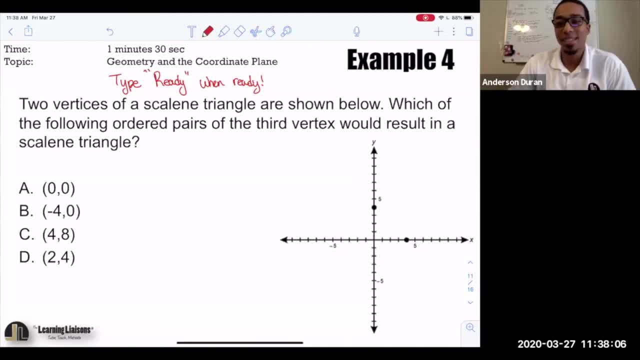 Got some clues, All right, so I love this question. Looks like I stumped a couple of us here And again. this problem is going to be on both the elementary math and practice elementary math. Both of these problems could be on there. 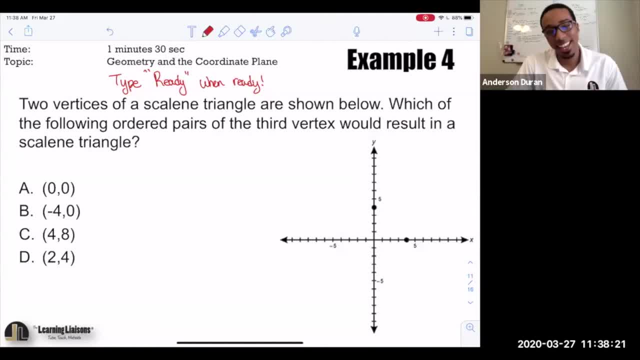 God, take the wheel, Not yet. Let's go ahead and let's reserve that. Don't know yet. Scalene deals with different links, I believe. Oh, there we go. There we go, Fred. So let's go ahead and talk about this. 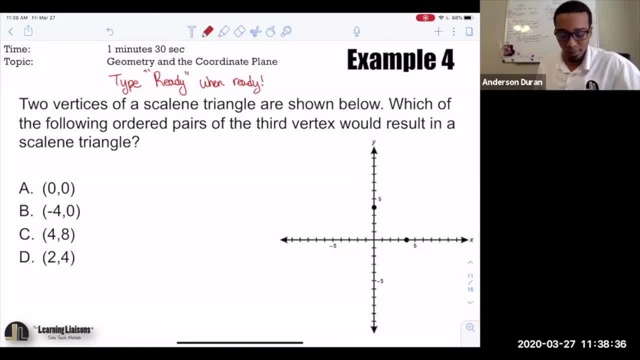 So two vertices of a scalene triangle are shown below. All right, so again, only talk about what you can easily recognize. If it's something that is like a definitive vocabulary word that maybe you got to think about for a second, just go ahead and highlight it or underline it. 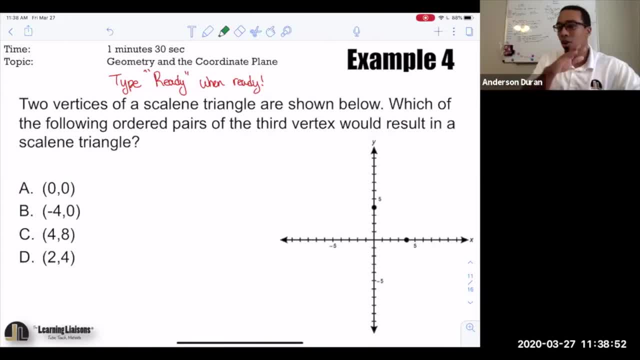 And if we're taking a computer-based screen, then just go over the word. All right, just take note of it and be like, hmm, don't know that word, but whatever, Don't get hung up on the complicated things, Not yet at least. 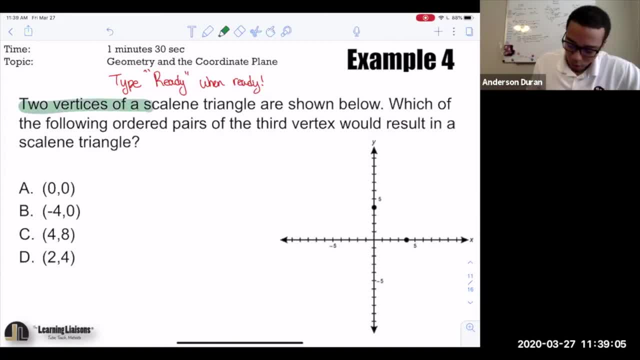 So again, two vertices of a scalene triangle are shown below. All right, I'm going to skip that because that's a lot of math stuff. But the question says which of the following- and remember what I said- which of the following means I need to analyze these answer choices? 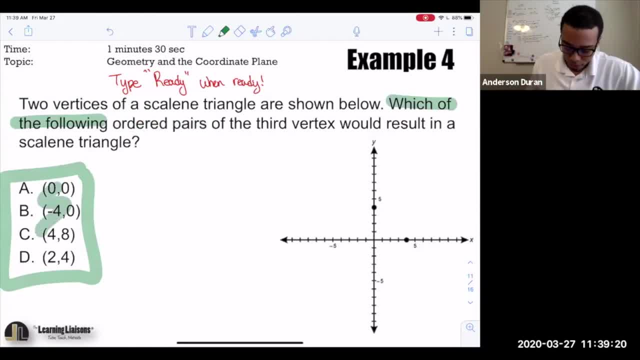 Boom. So which of the following ordered pairs- yes, these are ordered pairs- of the third vertex. okay, third vertex I'm going to highlight that would result in a scalene triangle. Okay, so I'm not going to, you know, try to think too far into this. 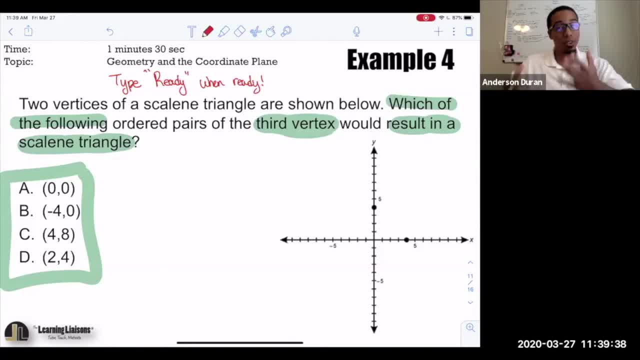 I'm just going to try to break that question down because this is almost a pure math question, But what I did understand was which of the following? so analyze these choices or maybe plug them in ordered pairs. again, those are ordered pairs. 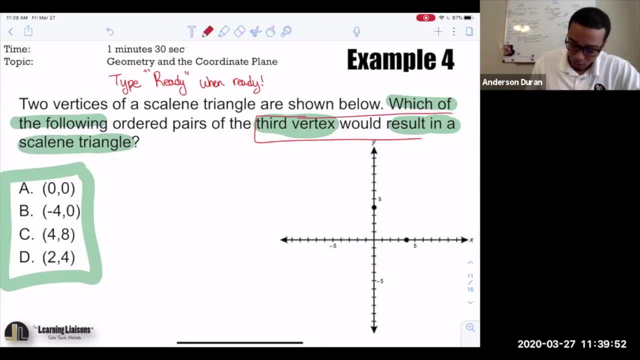 would be the third vertex, resulting in a scalene triangle. Okay, so we want the third vertex To form a scalene triangle. We're going to break that down in one moment. So we need an x and a y, We need a coordinate. 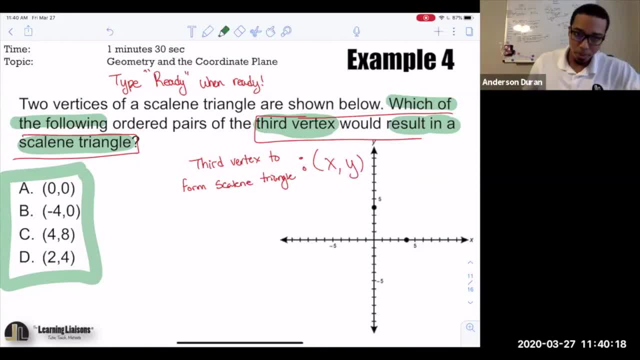 Now let's go ahead and break that down. Third vertex: Well, third vertex in what? Well, we're talking about a triangle, And how many vertices Or how many points do triangles have? everybody Right, we're going to start with the standard information that we can work off of. 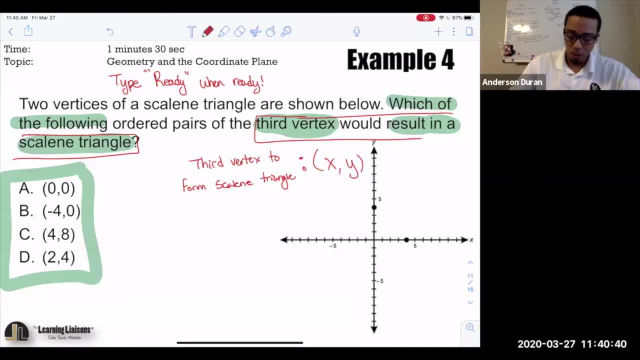 So we know that triangles have three vertices And we're here in this problem. it states that we're looking for that third vertex. So, with that said, well, my first question is: do they give us the first two at all, Like, do they give us the first two vertices? 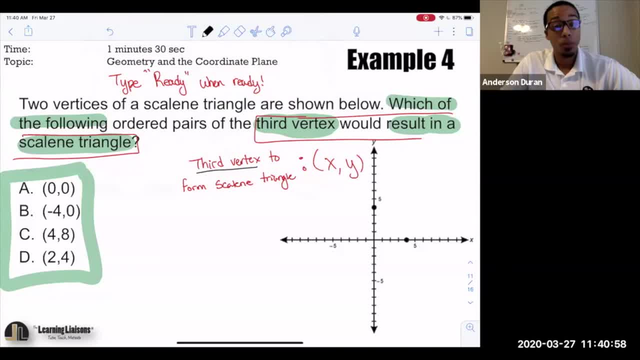 Right, they absolutely do. When we check out the first part of the problem, it states: two vertices of the scalene triangle are shown below. They're shown here and shown here, And there's a word that I've seen twice now: scalene. 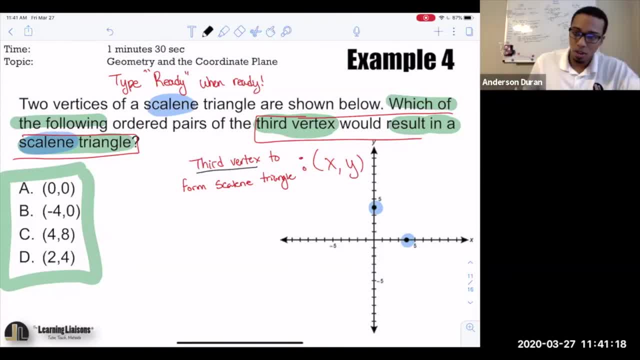 So we need third vertex to form a scalene triangle. So goal: scalene triangle. what does it mean for a triangle to be scalene everybody? So let's be specific, not equal. in what way? Let's go ahead and say it so that everybody can rally behind that thought. 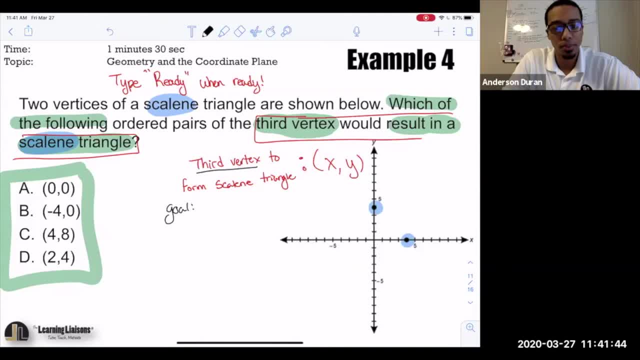 Scalene triangle. what is a scalene triangle? Two, not quite. Way to see who can get it spot on. Boom Fred, you got it Exactly exactly. Yep, we both got it. So again, for a scalene triangle, none of the sides are equal in length. 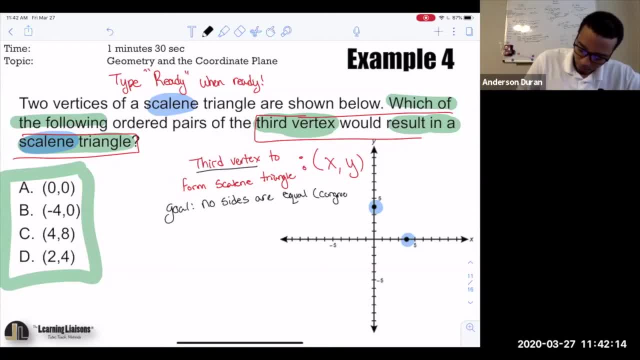 I'll say equal, but the correct term is congruent. All right, So our goal is to find that, you know which of these will give us no sides being congruent for a triangle. And now, what do we have so far? 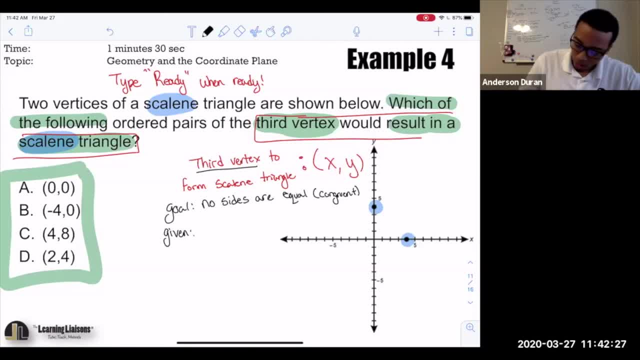 What's my given information? Well, I'm told that the two vertices are here and here, So let's go ahead and name these coordinates. What's this first one down here? What's the name of this first one? How do I name it? 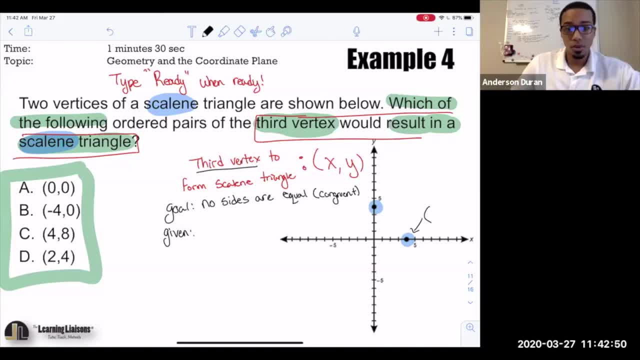 Well, no, we just want to name the coordinate. So some of us have a lot of time. Some of us are saying 0, 4.. Others are saying 4, 0. So let me go ahead and clear up that confusion for one moment. 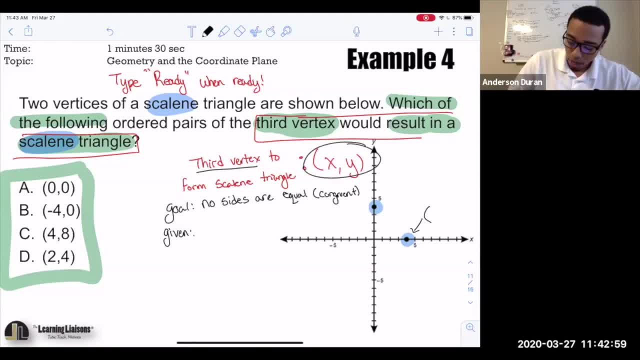 When we name vertices or coordinates, we are going with the x-coordinate first and then the y-coordinate. It goes in alphabetical order: x, then y, And so the x is here and that's 4.. The y, or how far up and down it is, is 0, because going up would be positive, down would be negative, but on the line is 0.. 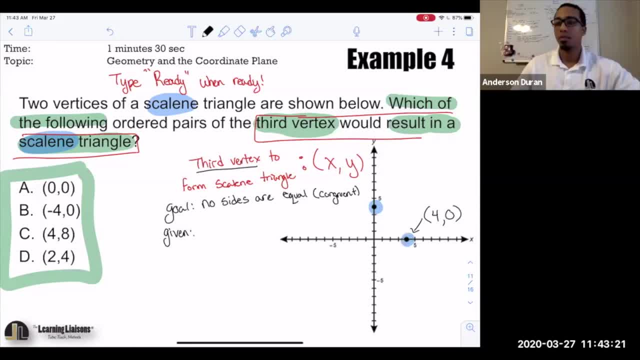 So this is 4, 0.. So we have x- 0.. No worries, I'm glad that I could just clear up that confusion. And then here, same deal. we're the x naming first. Again, it's positive over here and negative over there. 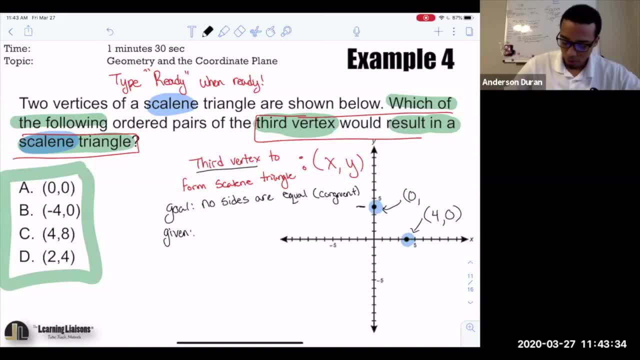 So it's 0 right now, And the height is all we're looking at, which is 4.. So we have 0, 4 and 4, 0.. Let me separate these a little bit. That way it's not too confusing. 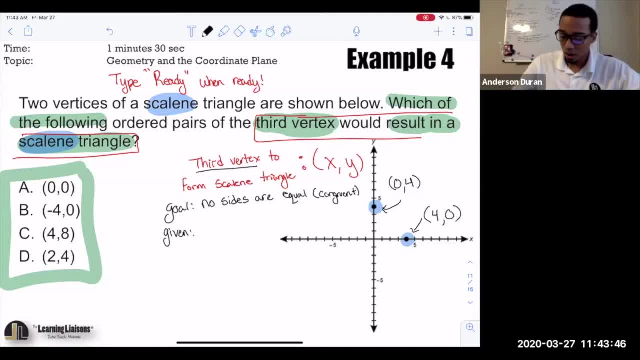 So, with that said, now what we're going to look at are the third vertices. that are our options here, because the thing is, we're given the coordinates and we want to know which one of these can we plug in to make it scalene. so let's go ahead and start off with zero, zero. 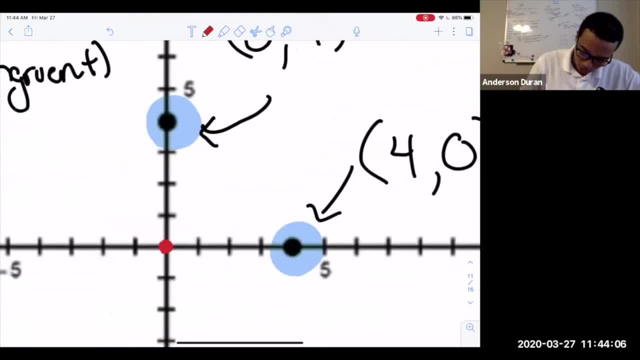 if i were to go ahead and plug in zero, zero right here and made a triangle, what kind of a triangle would this be? everybody, would it be scalene? okay, so we see that it's a right triangle, but is that really important in this problem, though? because a right triangle can be scalene, so let's go ahead and only use 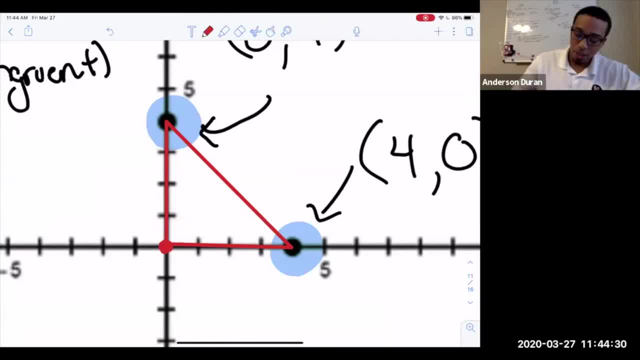 the information that we really need to think about and the three types of triangles that we can have. remember: they are scalene, they are isosceles and the last one is equal, uh, equilateral. these are the three types of triangles that we can have, so in this case, we would definitely not. 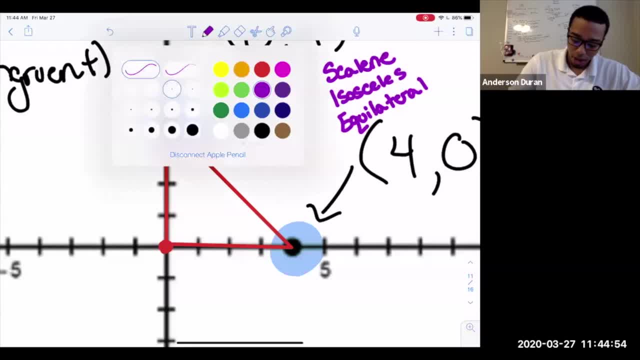 have a scalene triangle, simply because this would be a length of four and that would be a length of four. so everybody, before i continue, give me a yes, if you understand that a is not the answer, because the coordinate zero, zero would create an isosceles triangle. 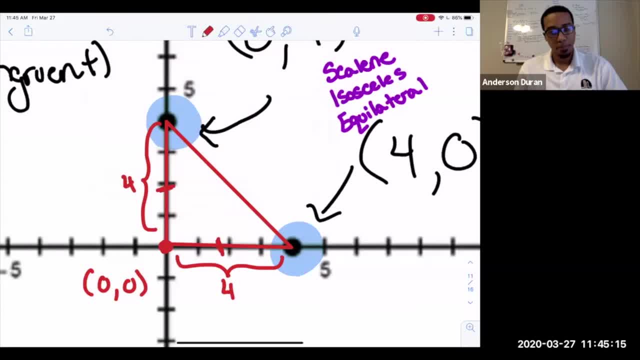 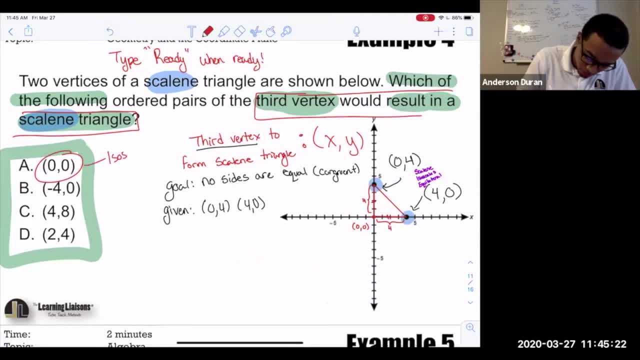 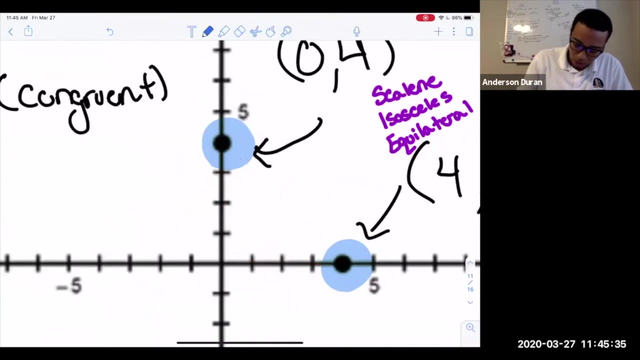 so i'm going to go ahead and go back, and again, this is an isosceles, so that can't work. now i'll move up to use blue here for this one negative four comma zero. so going back, let's erase what we've got. bye, bye everything. and i'll go to negative four comma zero again. the x is first, then the y. 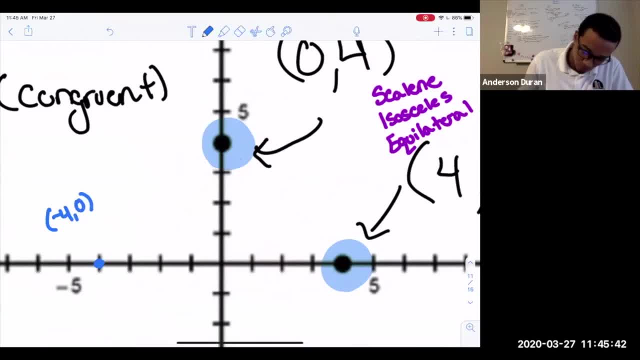 so negative four comma zero, and i'll go to negative four comma zero is right there. now i can go ahead and draw this out. what kind of a triangle would this one be? or is there anything that we know about this, that, even if we don't know what the exact lengths are? 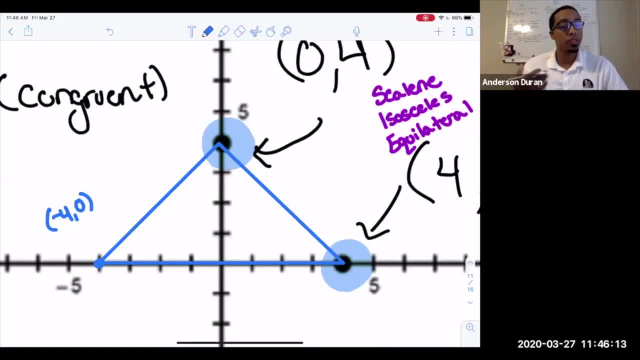 so not equalized, etc. but i just want you to remember that the plus and minus están here, and so these dosis are usually right there and beside here. these are like these, sorry, like this side, sorry that cs and dei structural, this one actually, at the very least via isosceles. here's why we're going from this coordinate right here. we're going from right there and it's going the same distance. it's going down four over four to get over here and it's going down for an over four to get over there. so it's perfectly reasonable for us to say than these two sides are equal or congruent. so this one is isosceles. 치�ialize in me now what would be the answer here is to one or two �ruktur. 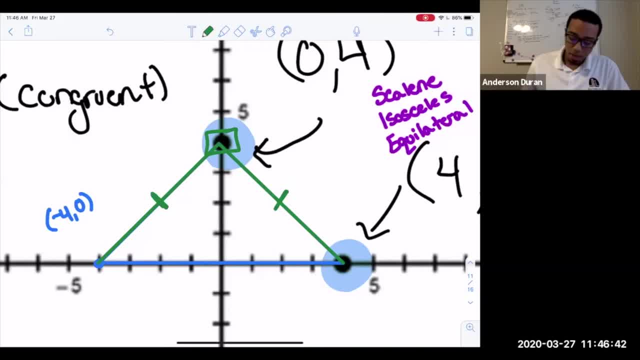 one is isosceles, no matter what, um, it is not going to be equilateral, because this is actually way, um longer. that would actually be. i believe that would be a red isosceles. i believe, yeah, it is actually right: isosceles, because this is 45 degrees and that's 45 degrees. 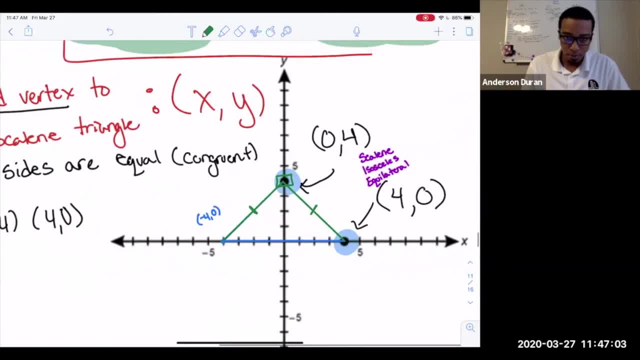 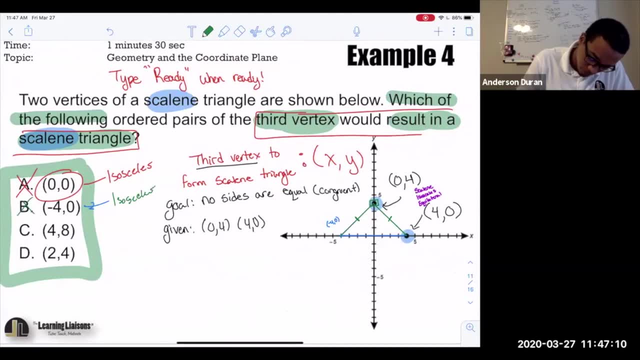 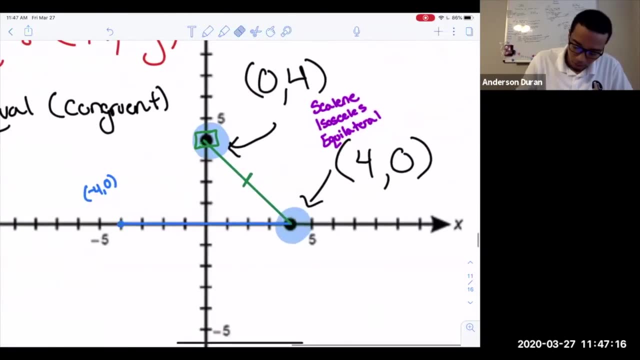 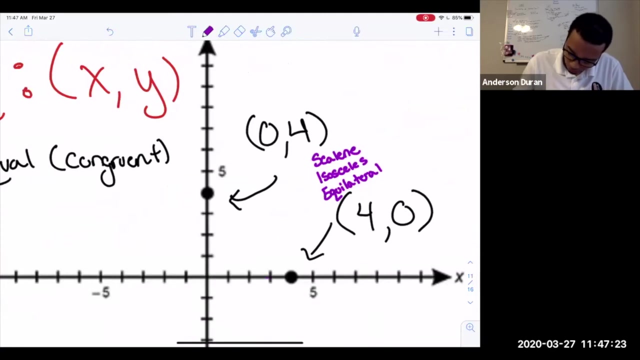 so this is a right isosceles triangle. so boom. so, with that said, this is again isosceles. what didn't work? next c, four comma eight. so let's take everything down again and write in four comma eight. so here's four, six, seven, eight, so i can connect the dots right here. 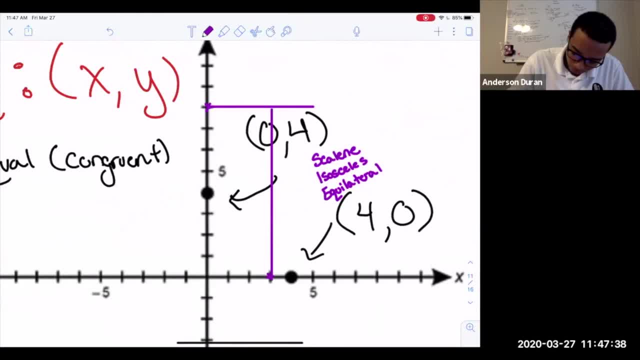 boom. so there's my dot that i'm going to connect. all right. so if i go ahead and work this out, what do i see? oh whoops, i made a huge mistake. oh man, i need to go up from here. boom. so when we take a look here, 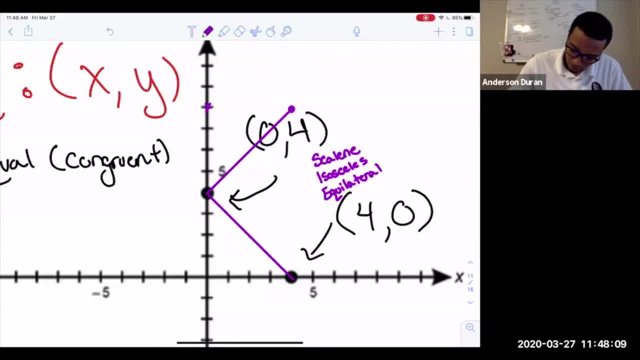 here's what we got: straight line there, straight line there and then up, and this is the same situation. what we're going to have here is, well, this side and this side are the same because, again, for this point, to go to this point, what we see is going over four and up four to get to eight. this one is going over four and down four, so again, 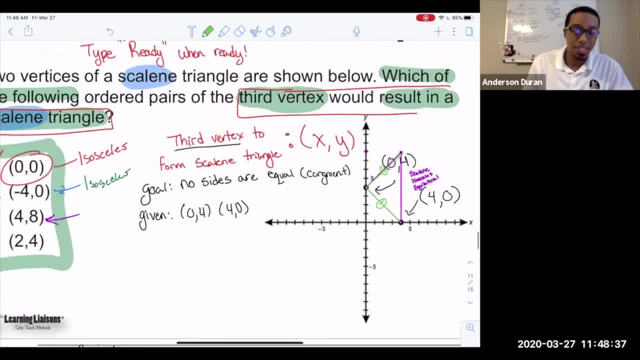 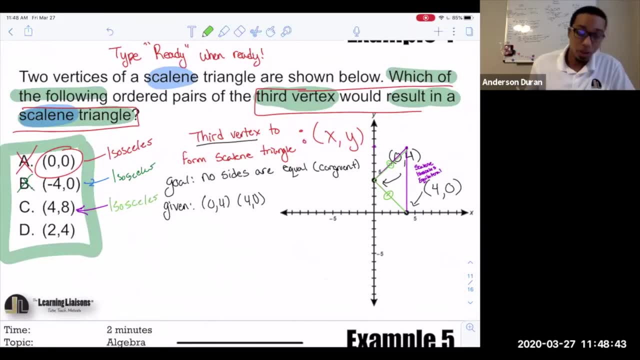 so the sides are equal. that would be isosceles yet again. so far are we all good in understanding why all three of the first options are isosceles. yes or no? all right, perfect. so then by default, you know, we can say that d is the answer. so by default we can say, yeah, d24 is the answer. but i 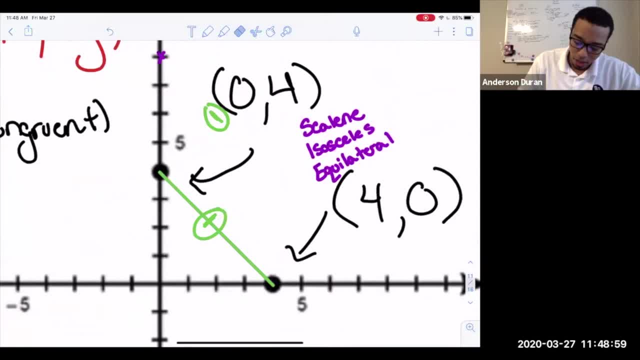 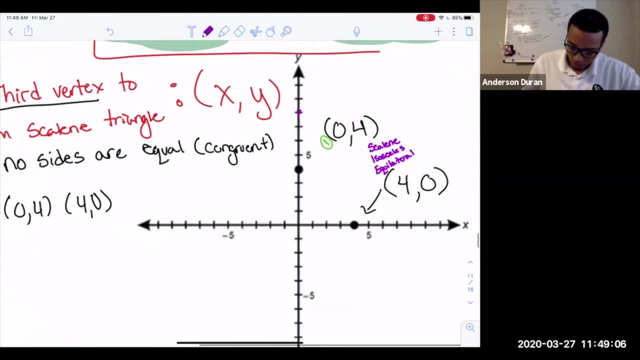 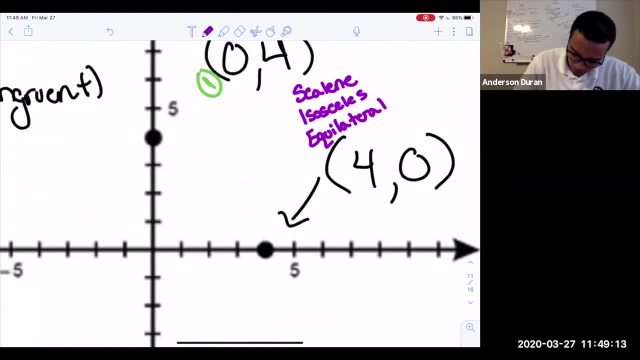 don't want to cheap shot you guys. i want you to see everything that is being, that's necessary to see. so 24 was the coordinate right, 24, perfect. so what i'm going to do is i'm going to graph two, four, four. right here, sorry, right there. 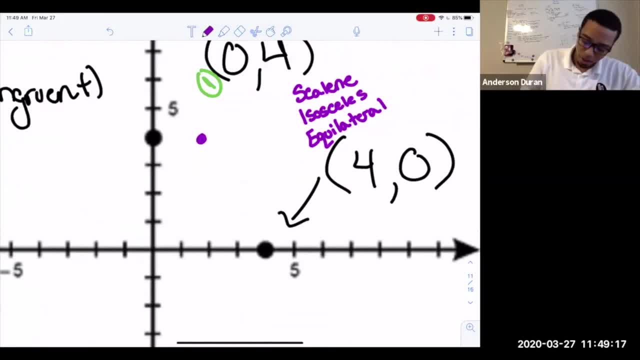 and when you think about it, all right, cool, here's what we're going to see, and there it is, so, so, so that would definitely be a scaling triangle. so, with that said, scaling again, no equal sides. so, taking a look here, yeah, this would be a distance of two right here. 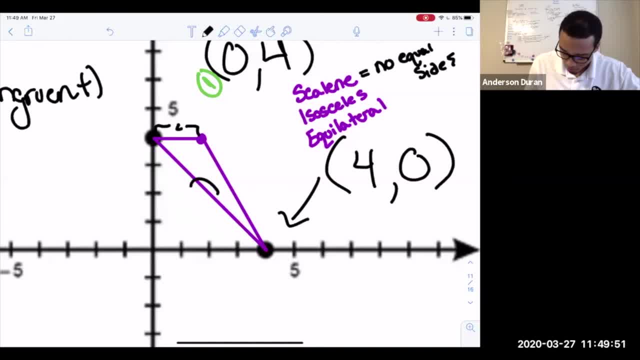 uh, you can actually use the pythagorean theorem to find this one out. but we know for a fact that this angle is the biggest one, so this is the biggest side, and then this angle, or this side here has the smaller angle. so it would be, you know, slightly bigger than this side, but not bigger than this one. so we know. 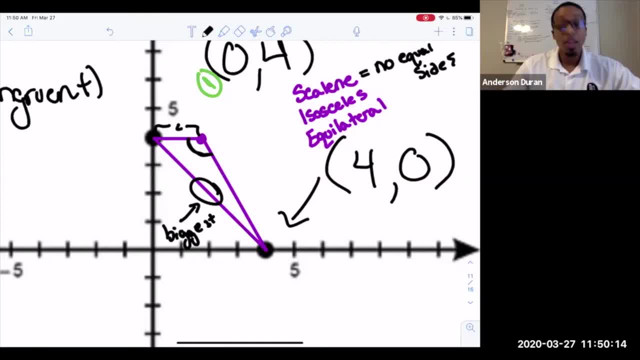 there's a hierarchy here. we're goal. equilateral is when all the sides are the same. all three sides are the same. that would make it equilateral. so, um, if we had a triangle, let's say it's the same for all three sides to be the same again. we would just need to see something along. 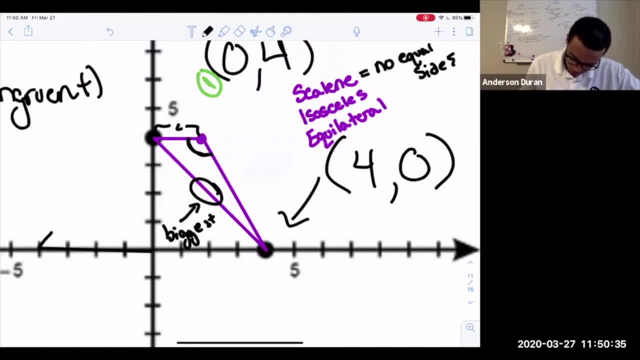 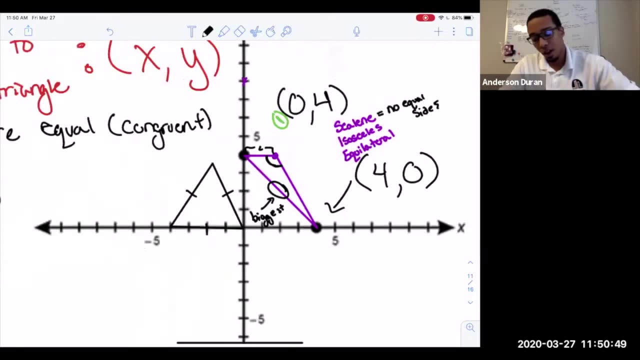 these lines something like this: it equalizes means all three sides are the same. that's all it means, and so we need to see all three sides being the same, or be able to measure that to do it. but in this problem, we were only looking for what would make it scalene, and so we just went through. 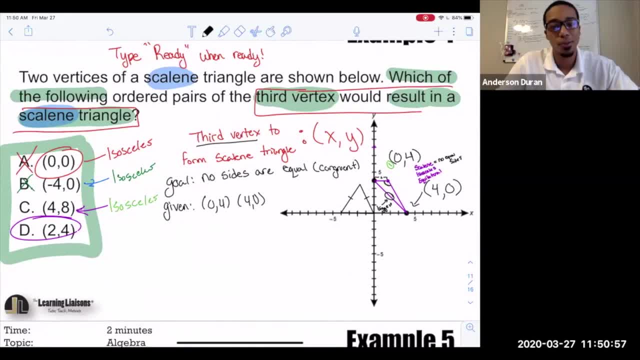 all four choices found that the last one is the one that works, and so we haveutted all four of these to the孩, not the original value. so the right answer is the right answer. the left answer is the right particular number. the right answer is the value of h and the right answer is the value of Martha. 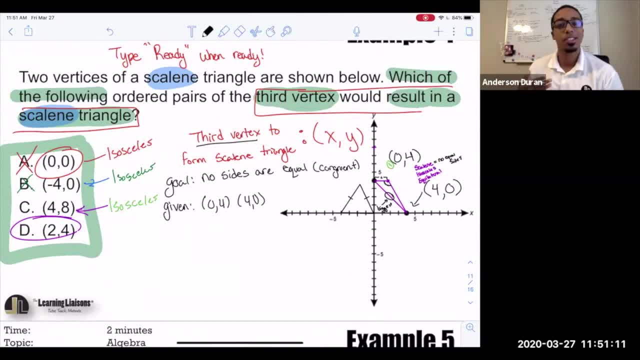 okay, so we're done with one of the questions and I hope you learned anything about it. let me make sure, when we get to this big question, what we can do at this point, we can look back at some of the choices we had. so we'll look at nine of our options. 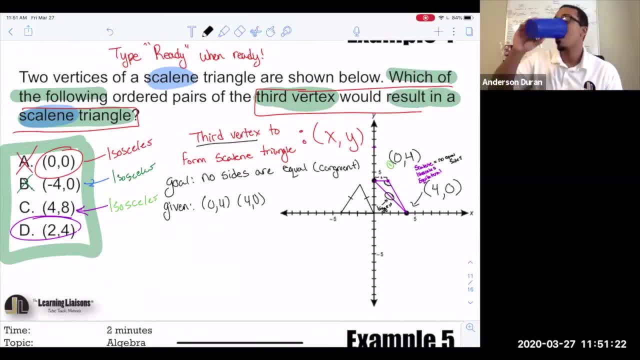 find out, okay, what, what works, for which answer? everybody says we need one, and then find out who's right, what doesn't, and if you want to do that, we can do four up, All right. so let's go ahead then. reflect or not reflect, but dive right into the next one here. 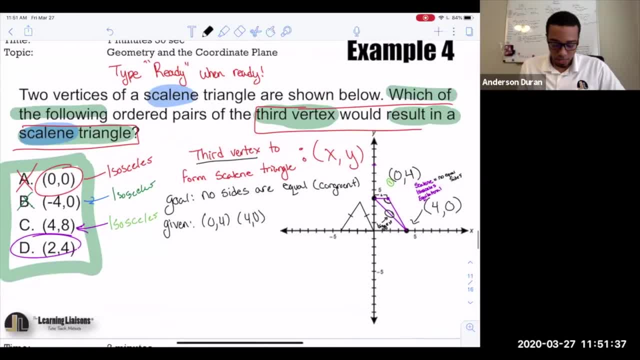 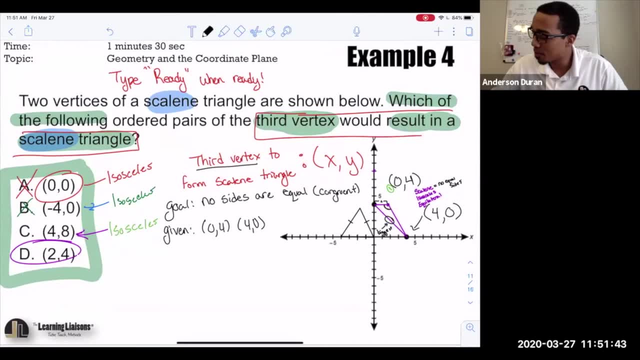 That's right, we got some coffee, All right. so number five coming up. We're gonna have two minutes to get this one done again, So let me get and set my timer. All right, we're getting started in five, four, three. 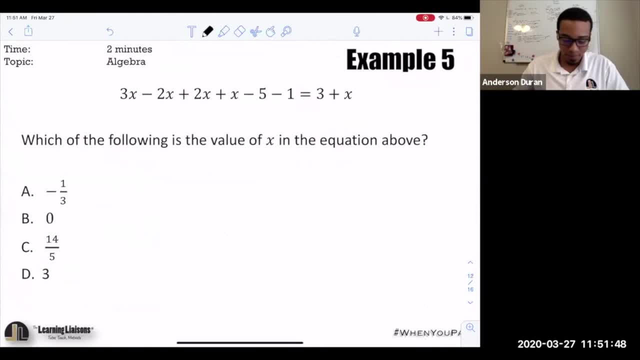 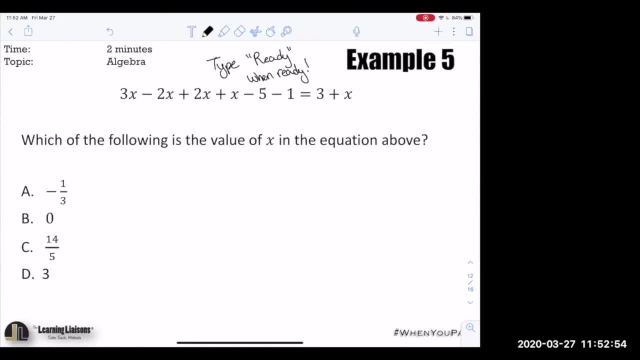 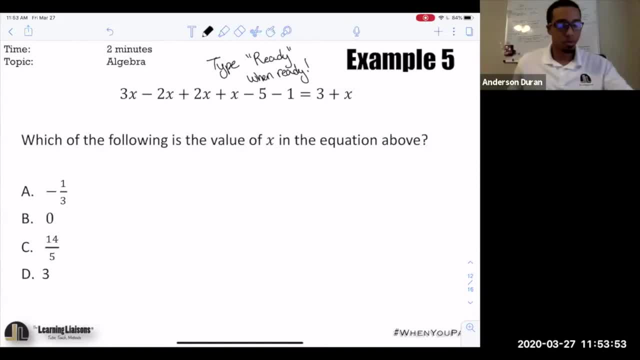 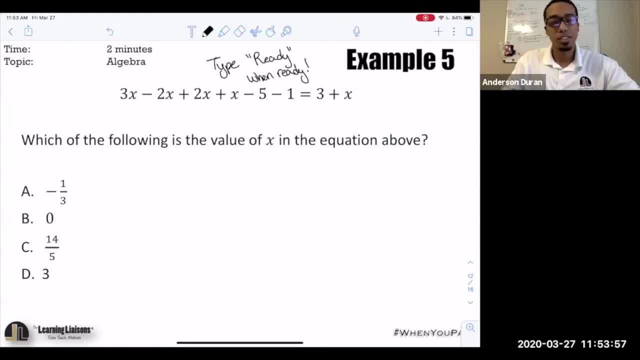 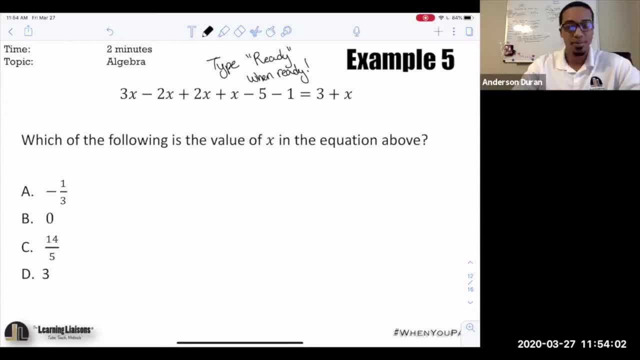 two, one go, All right. we're getting started in five: four: three, two, one go, All right. we're getting started in five: four, three, two, one go, All right. that's not good. C D A. C B D A. 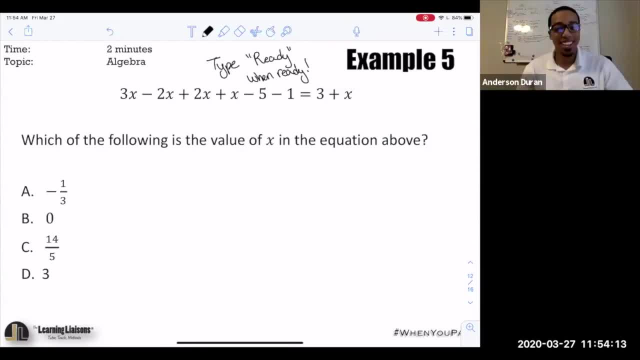 Okay, it looks like we're all disagreeing right now. It looks like it may have taken us a little more than two minutes to get something like this done, But let's see what the rest of the answers are. More Ds: you got a C in there. 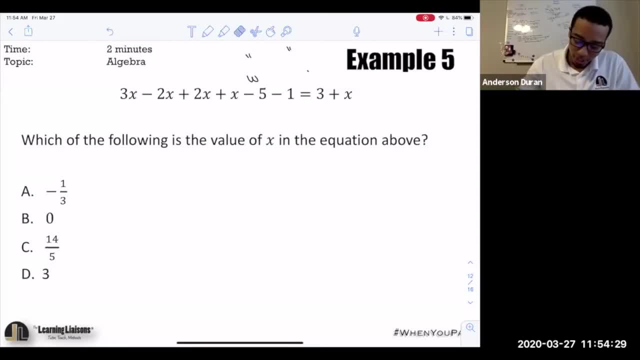 All right, so let's go ahead and review it, then Let's review it, So let's review it, let's review, let's review Destination plan followed. So, even though it's an equation, again, destination plan follow always applies. 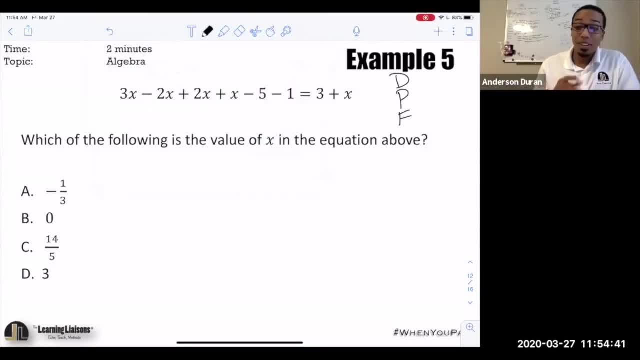 So begin by again not addressing the complicated stuff. So if I'm reading this problem, I am not gonna spend or waste my time going three X minus, two X plus, two X plus X minus. no, No need to read all that. 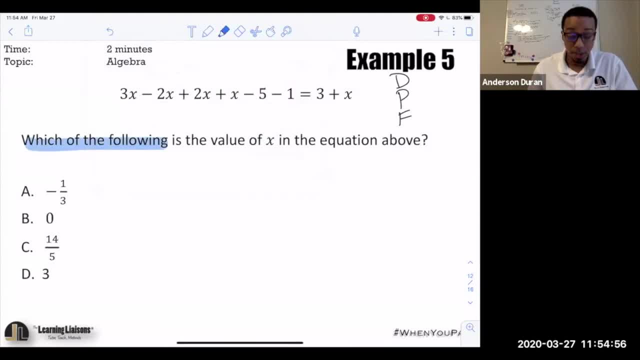 Just go straight to the question. Which of the following? Okay in my head, if I have an equation up here and I got numbers here, we're looking at what the answer is to this. But let's see what the question says. 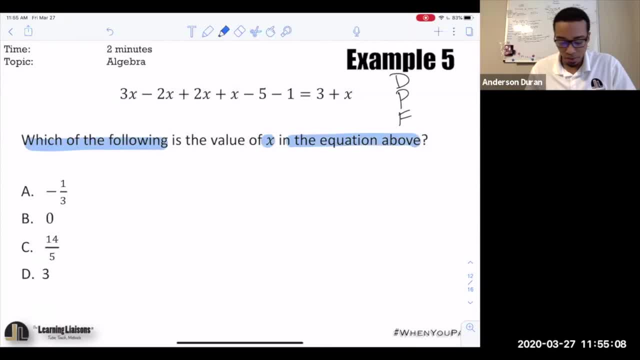 Which of the following is the value of X in the equation above All? right, we've seen problems like this before, So boom, check it off, Solve the equation, get X sweet. So what I'm gonna do first is I'm gonna see: 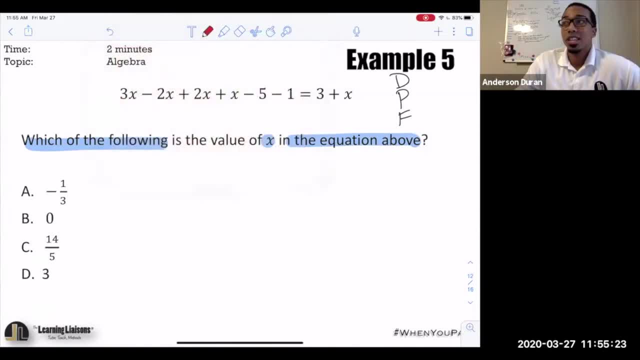 look, in solving equations, there's usually something everybody does: Get the Xs on one side, get the numbers on the other and then divide. That's usually the goal. Now they're gonna present these problems to you guys in different ways. 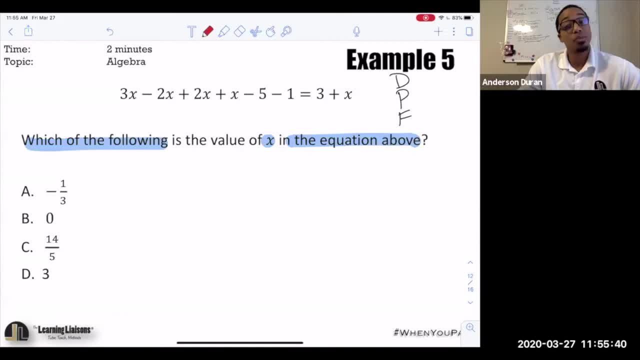 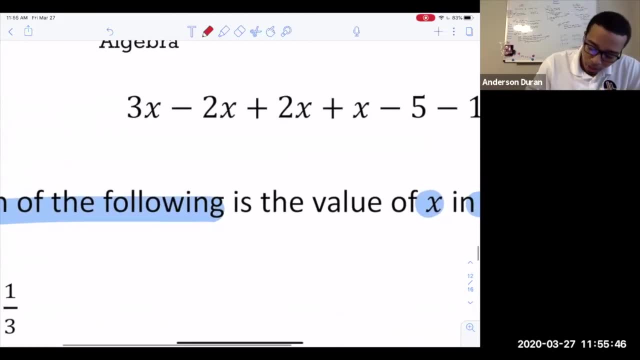 Ways. that would make sense if you looked at some nice simplification steps before you began. So, for example, some of us may be inclined to start the problem like this: Oh, let's start off by doing three X minus two X to get X. 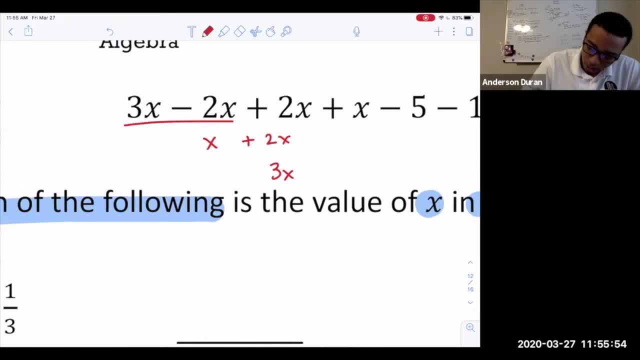 Then I'm gonna add two X and that's gonna be three X. Then I'm gonna add X here and I'm gonna make that four X. Now notice how we're going. We're going line by line and we're kind of spending some time doing that. 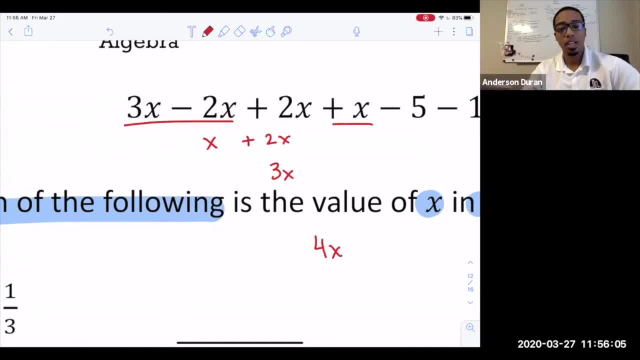 Here's something that I would really suggest that you do: moving forward Instead of going straight, left and right, simplifying. try this out instead. I noticed that we have a negative two X and a positive two X, So if those were to combine, what would happen? everybody? 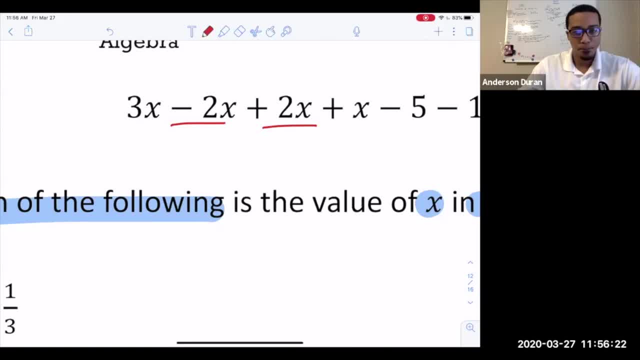 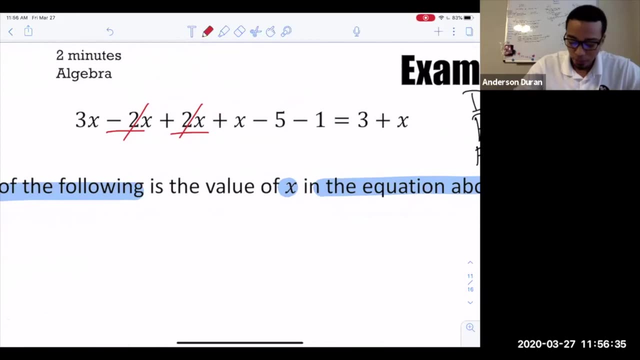 They would what? Absolutely They'd zero out, they would cancel, they go gone, they go bye-bye. exactly So two X negative, two X cancel each other out. Next I'm taking a look again: If- and this is a little more technical now- 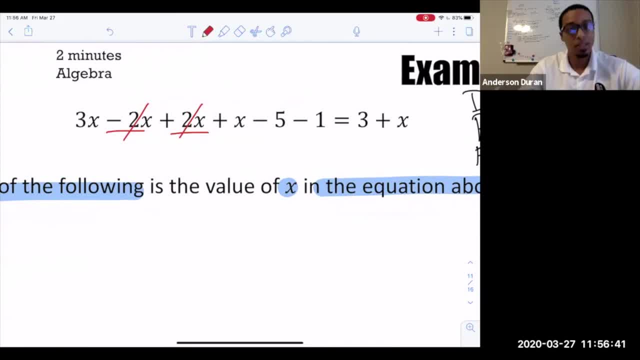 So you know how if you have a negative and positive on the same side, they can cancel out. Here's something that's also true: If you have the same sign on the same term on each side of the equation, those also cancel out. 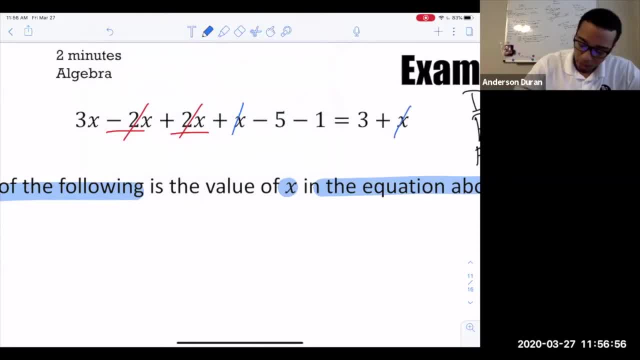 Here's what I'm referring to. I'm referring to the X negative two X, negative two X. I'm referring to the X and the X here. You wanna know why? Here's why, If I have the X here and the X here, 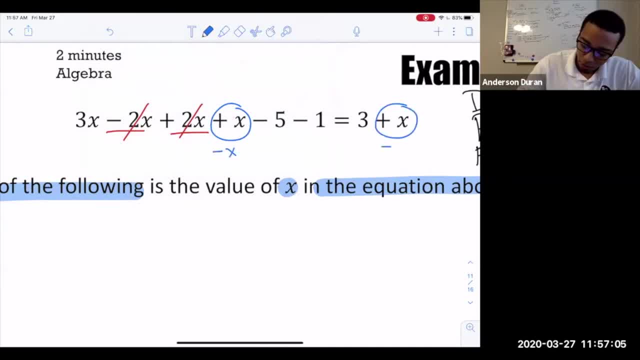 they're gonna cancel, because I can subtract X from both sides and cancel on both sides. That's why, if you have the same term with the same sign on each side, you don't have to do the work. You can simply cancel them out automatically. 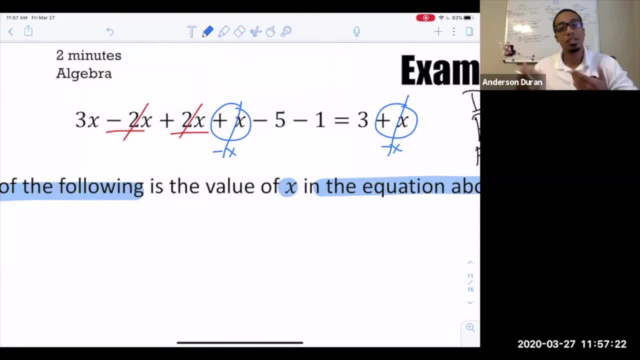 Because, again, the premise, the idea is that you can subtract on both sides And since they're the same term, they both are gone. So does that make sense? everybody Wanna make sure that I'm teaching you how to conserve your time on this test. 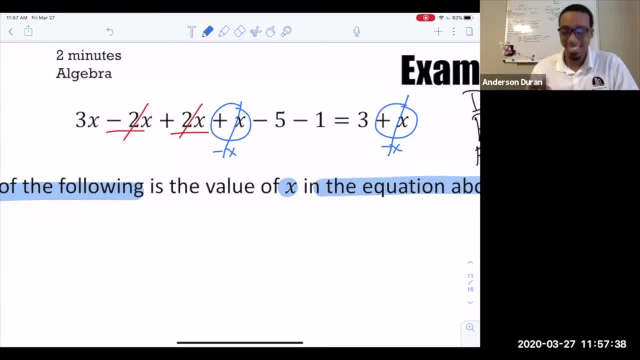 Sweet, right on, right on. Hey, I'm glad that you guys are really excited about that. All right, so there it is. I don't have to write that out, I can just say: all right, X and X on both sides are gone. 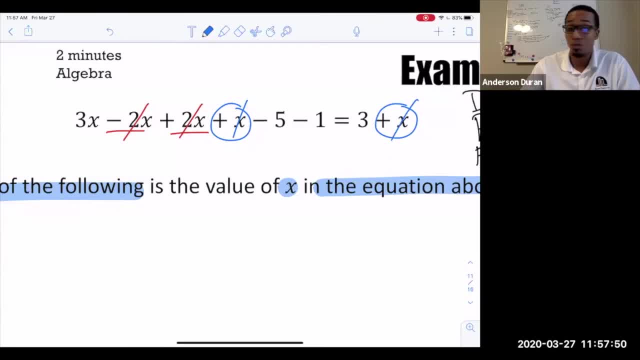 So, really, this simplifies my problem a great bit right off the bat, Because what I have now is three, X and negative five minus one, which would be negative six, And that equals three. So look at that, This is the essence of destination plan follow. 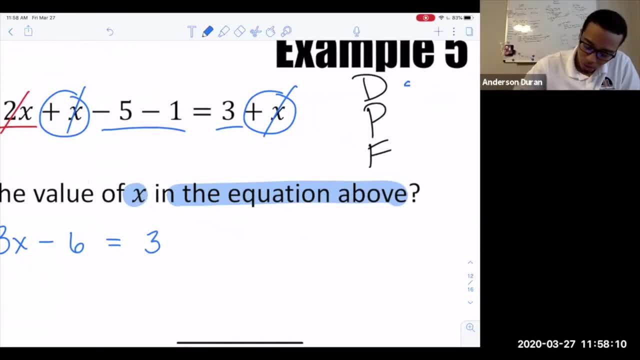 Our destination solved for X, So X equals what. That's what the destination was. The plan was well, analyze first, because you wanna simplify easily, then you wanna solve. You wanna analyze first, then simplify, then solve. If you simply go in there and try to solve, 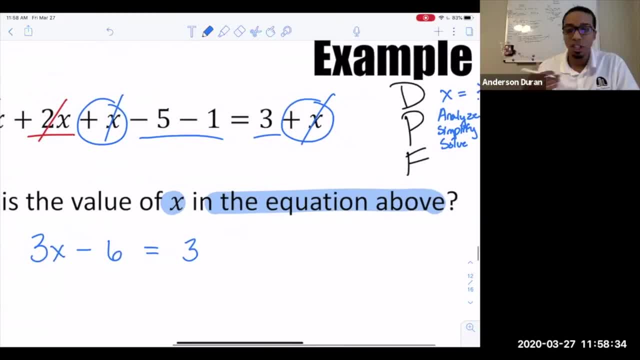 again going step by step. it's gonna be a bunch of lines And chances are you might make a mistake if you're writing a bunch on this test. So remember the whole thing of working smarter, not harder. this is what it's all about here. 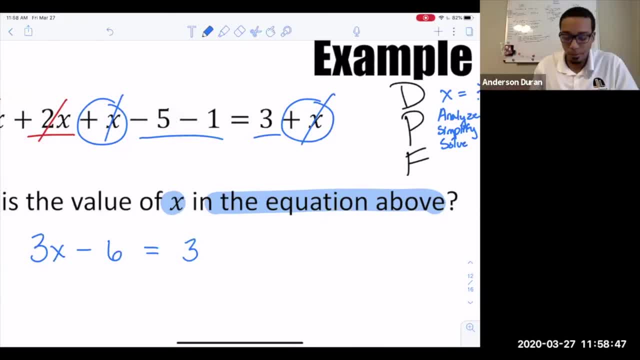 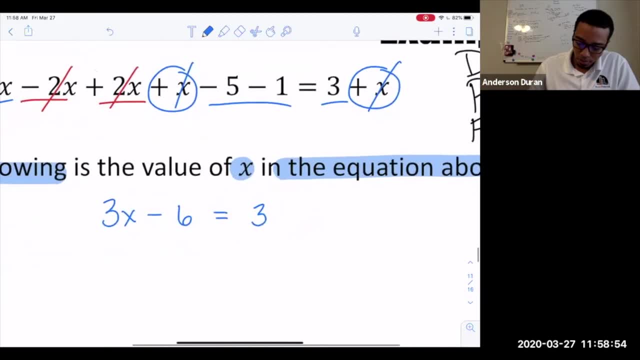 Knowing these concepts well enough to be able to apply some shortcuts. And so the four X's. So the following is: just follow this. So we analyzed boom, we simplified boom. Now let's go ahead and go through the regular process. 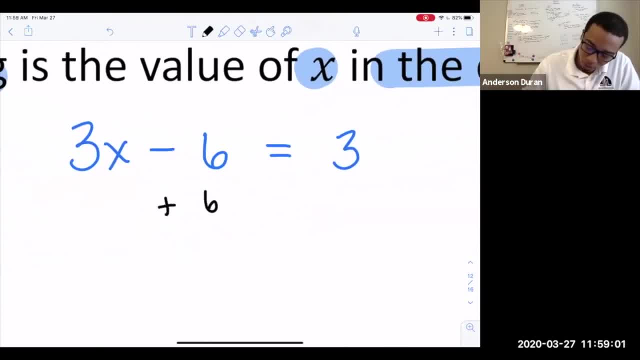 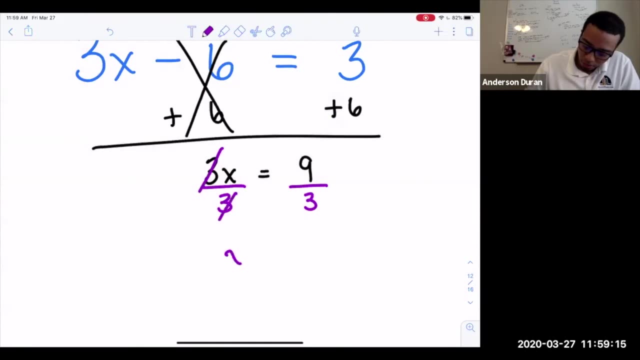 of solving an equation. Get the x by itself. so I'll add six to both sides. Goodbye on the left side, leaving me with three. x equals nine. From there I'll move to divide three on both sides. Cancels on the left, leaving me with x equals three. 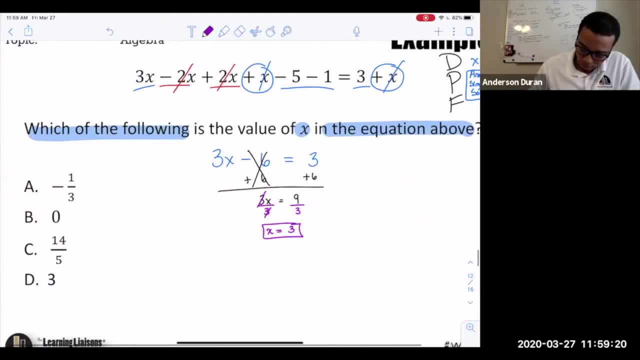 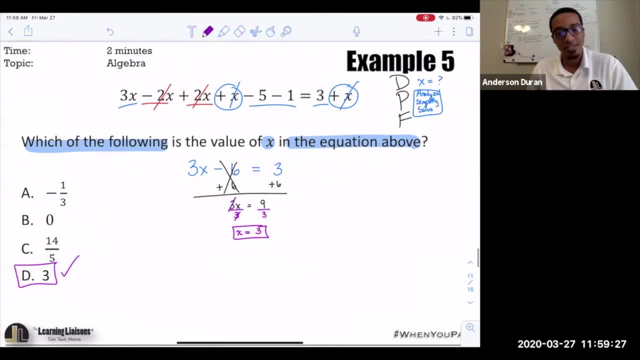 And boom from there. my answer choice here is D. So how do we feel about question number five? Diana will slay this test. I love it. I love your name there, Feeling good, great and better. Hey, that's what we're here for, guys. 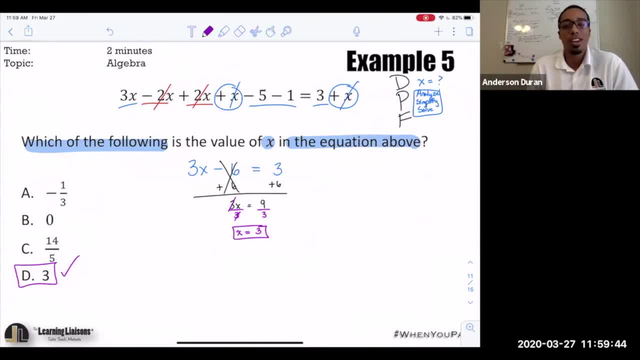 Again, there's so many different types of problems that you'll see, and I'm just trying to help you see it in different ways. So, Ashley, so what I'm? yeah, exactly what I'm referring to here. so you're saying you know you solved this. 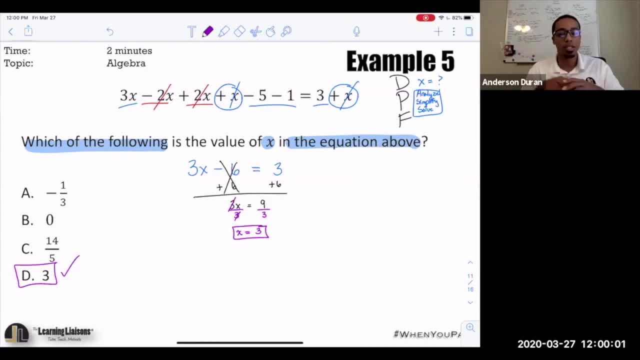 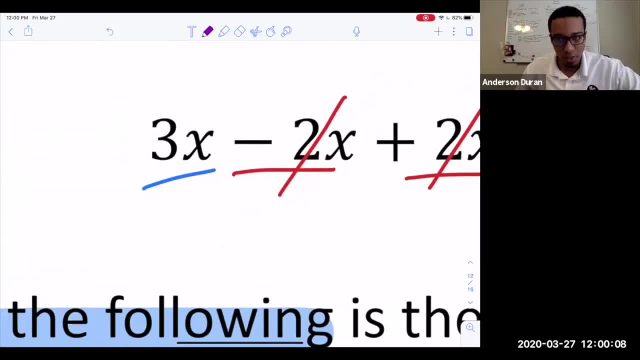 in a completely different way than you were trying to, and this makes more sense. And I believe that the reason that this may make more sense is because we're not zooming all the way into the first things that we see and then going left and right. 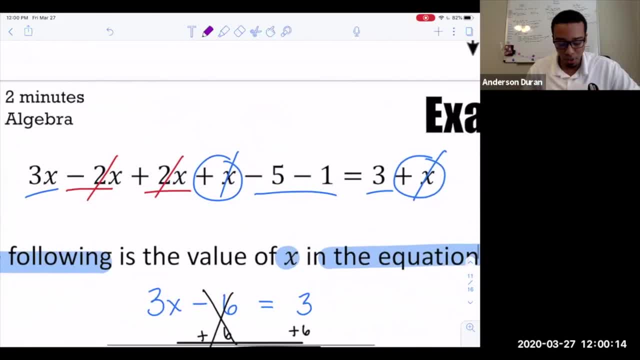 No, what we're doing here instead is: hey, let's take a look at the whole picture. Okay, Okay, Let's take a look at the whole picture And what ideas do I know or that I can recognize? Okay, negatives and positives together cancel out. 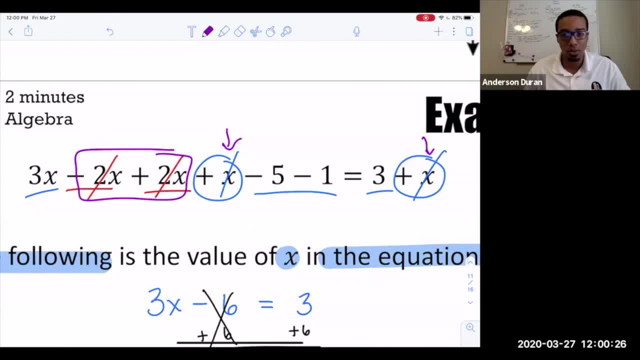 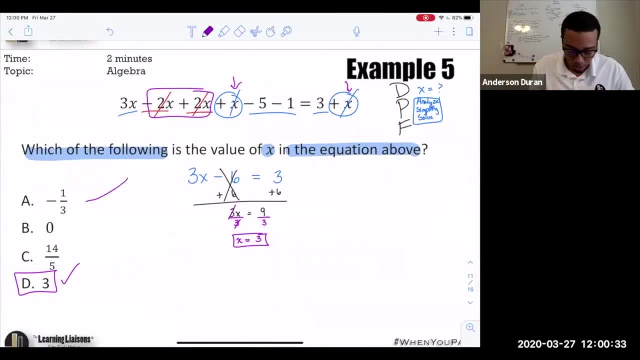 And if I have the same term on each side, those cancel out as well. So I did that, and then I went down the road. Another method that some of us may use is plug and shove, where we plug in numbers into everything. 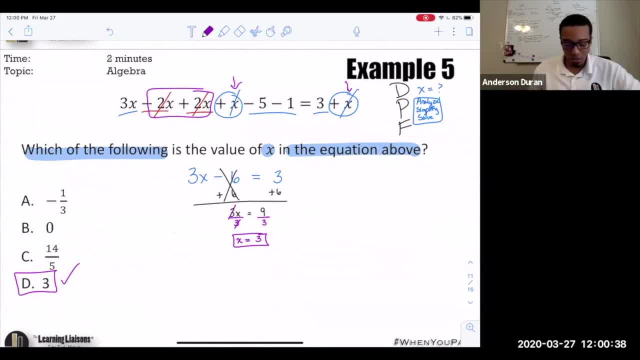 Now plugging in can still work, but I would recommend simplifying this first, because you don't wanna plug in the same number three, four, five different times. I wouldn't wanna do that. So, with that said, if you do, plug and shove. 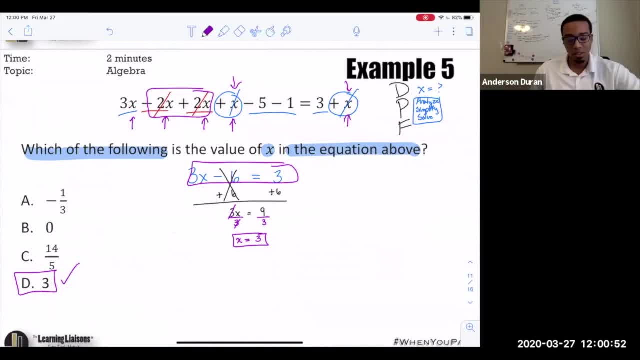 try to simplify it first into something like the three X minus six and then plug in. So I like that you take your time explaining, because my kids are driving me crazy and I'm trying to focus and keep up and this makes it easy. No reason, I'm glad that I can help out. 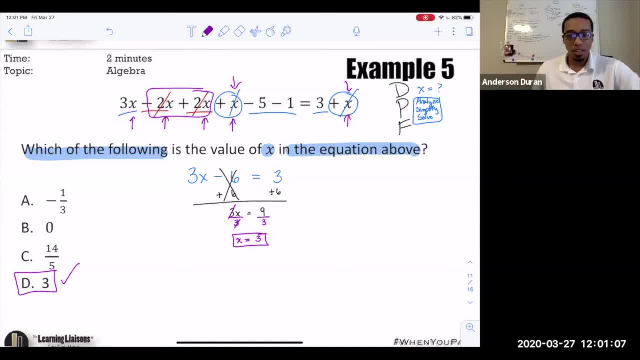 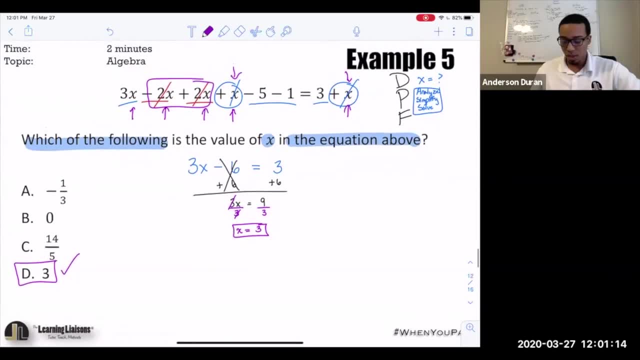 Again, this is an hour and a half, so it helps all of us out. All right, perfect, Thanks, Kamar. All right guys. so let's go ahead and look at question number six. Six, three, two, one go. 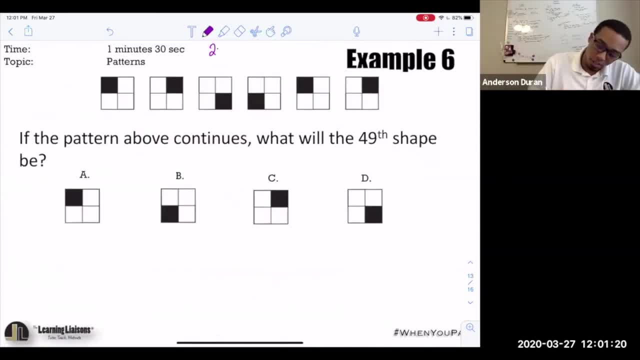 Last one of the day. I'm gonna give us a full- actually two minutes and 30 seconds- here. I wanna make sure that everybody has a chance to answer this. So two minutes and 30 seconds, starting in three, two, one and go. 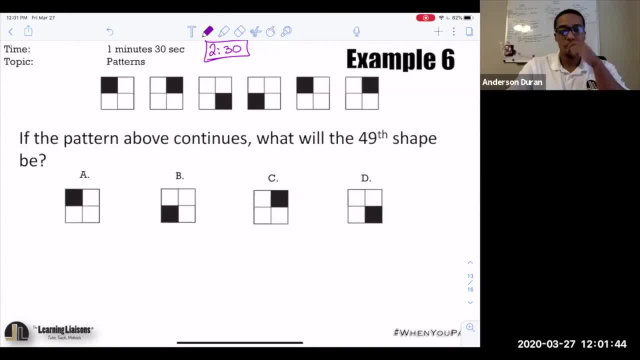 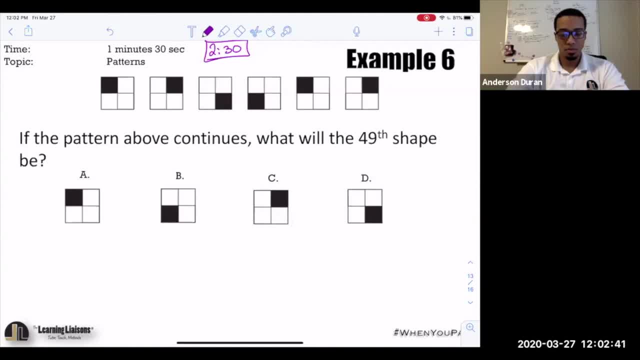 Thank you. All right, we're looking at one minute left. One minute left. You're good, Dania, It's all good. Five, four, three, two, one One Answers: D, B, A, B, D, A D. 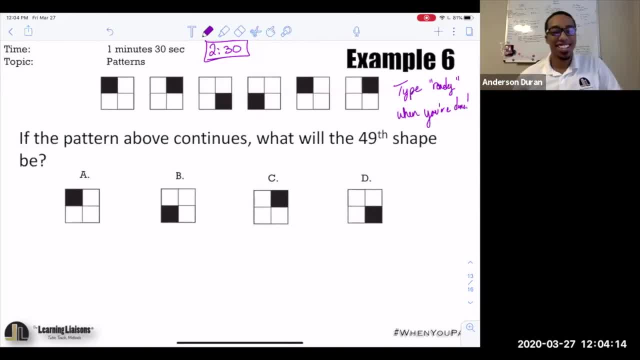 Oh gosh, Oh gosh. All right, so it happened again. Looks like we're all not on the same page here, But this is a good thing, because this is a really good question to ask. This is about pattern recognition. 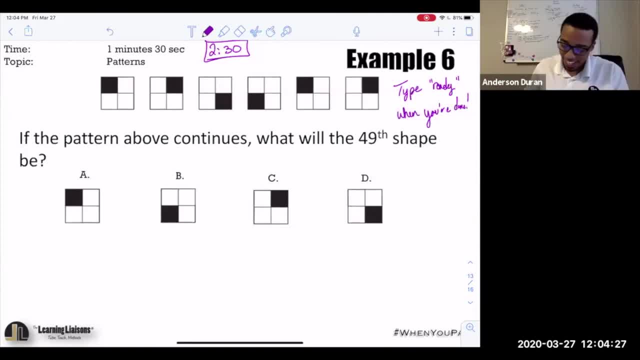 And I'm excited to do this one. I'm excited, I'm excited, I'm excited. So, if the pattern above continues, what will the 49th shape? what will the 49th shape be All right, so, no matter what, guys. 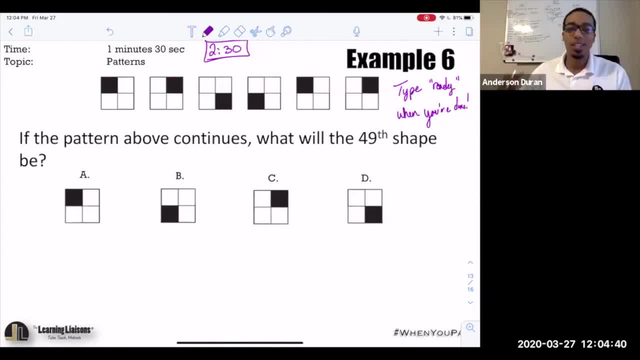 even if you see a problem that you again don't immediately recognize, you get nervous or whatever it is, destination plan follow. If it helps, you write that out every single time. you do a problem. do it Seriously, do it. 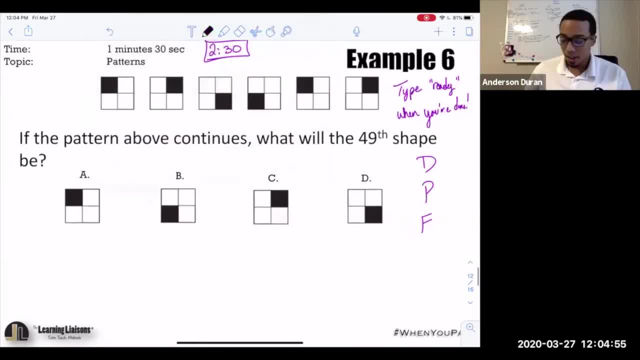 So destination, let's start here: Destination. Okay, what am I looking at and what is the question? I'm looking at what looks to be a pattern. So if I'm thinking about it, okay, top, top, left, wait. 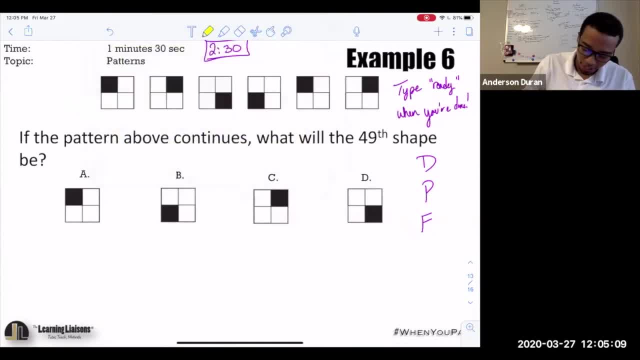 let me try to get a yellow here So it actually sticks to the screen. Top left, top right, bottom right, bottom left. Oh, then top left, top. Oh, okay, So there might be some pattern here that I'm looking at. 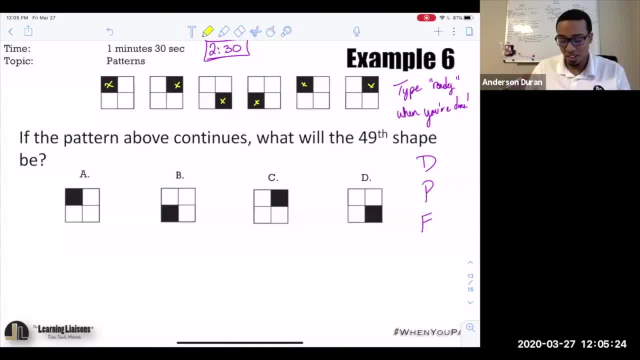 Hmm, I see a pattern here, but let's see if that even is going to help me. So it says: what will the 49th shape be? Oh, if that pattern continues? Okay, Yes, we're talking about this. 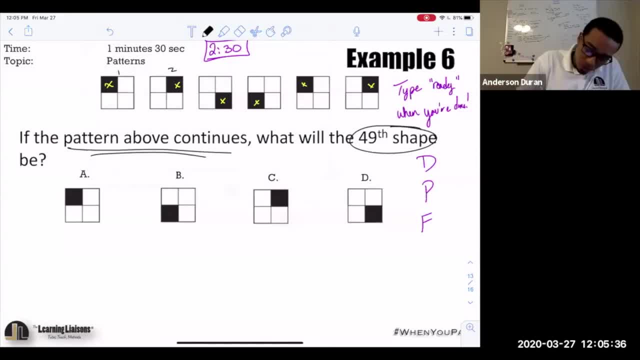 So this is number 1,, 2,, 3,, 4,, 5,, 6, and it continues. My question is: how many of us and type yes, if you did it, how many of us drew squares all the way through the 49th one? 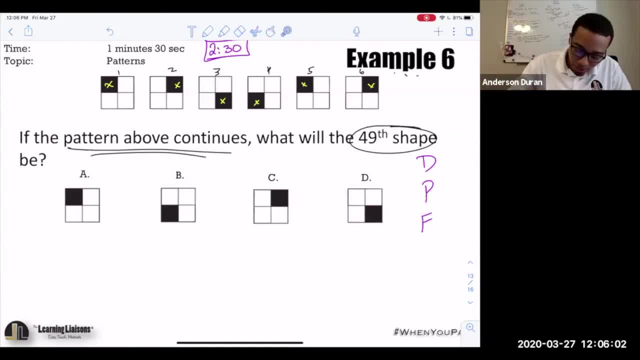 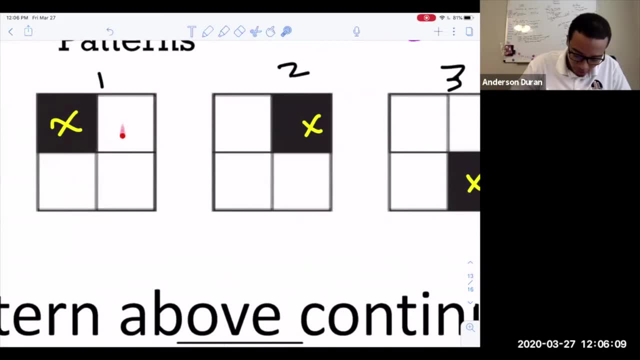 You know what I'm saying is: did anybody go? you know, go, okay, I want to see which one the 49th one is. So 1,, 2,, 3,, 4,, 5,, 6,, 7,, 8,, 9,, 10,, 11,, 12,, 13,, 14,, 15,, 16,, 17,, 18,, 19,, 20,, 21,, 22,, 23,, 24,, 25,, 26,, 27,, 28,, 29,, 30,, 31,, 32,, 33,, 34,, 35,, 36,, 37,, 38,, 39,, 40,, 41,, 42,, 43,, 44,, 45,, 46,, 47,, 48,, 49. 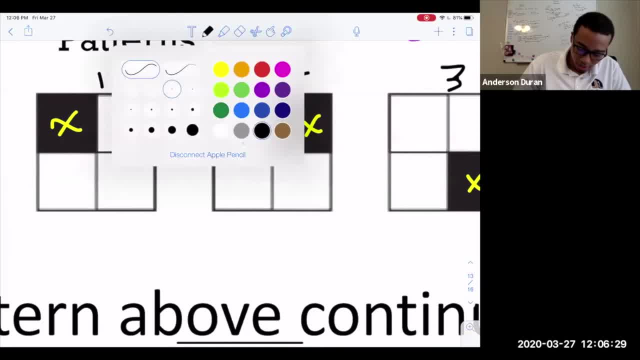 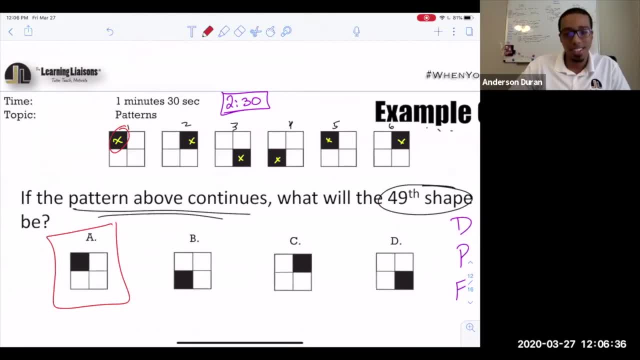 Okay, Did anybody do that? Did anybody do that? All right, So we have some people that said yes, some people that said no, Some people said that they used the pattern and multiplied. So I'm going to go ahead and be very honest with you guys. 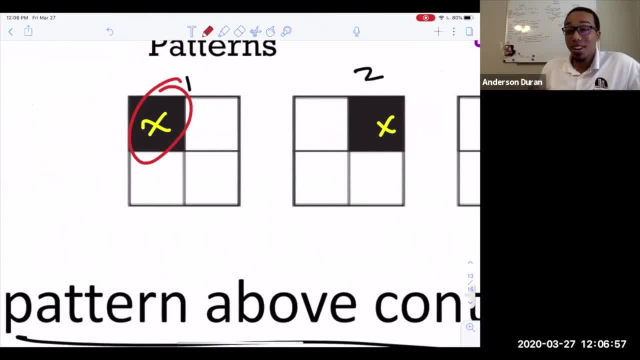 If it's test time or, sorry, if we're practicing, we can feel pretty confident that we can do that. you know going 1,, 2,, 3,, 4,, 5, you know all the way around. 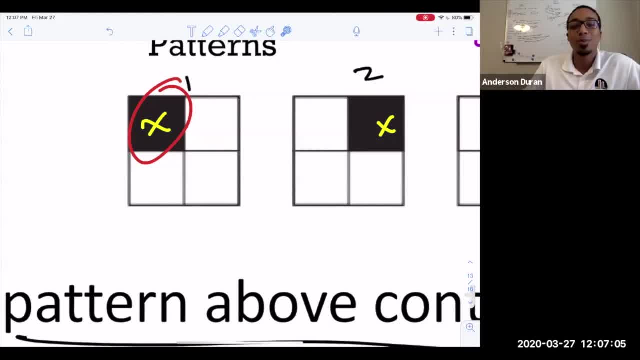 But on test day, I can bet you right now, your anxiety is going to be through the freaking roof. You're going to be like 1,, 2,, 3,, 4,, 5,, 6, and you're going to get to 25, and you're going to be like: wait, crap, which one was I on? 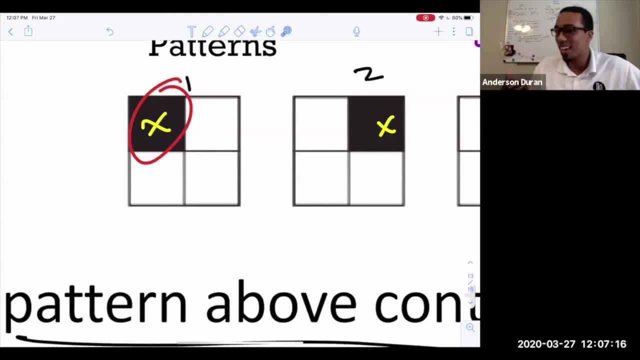 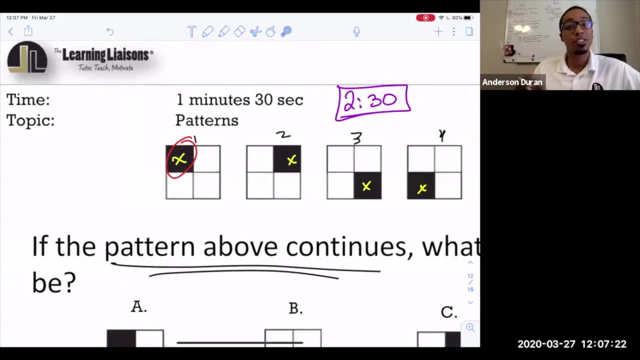 And you're going to start again, And then you might guess- you know, second guess- yourself. It's going to be annoying, But if it works for you, it works for you. So let me show you an alternate way that's going to guarantee that you know which one it is. 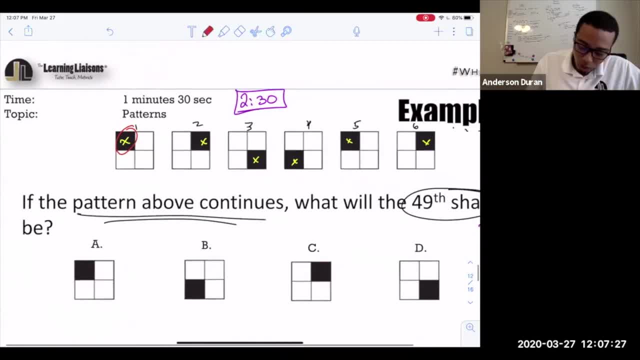 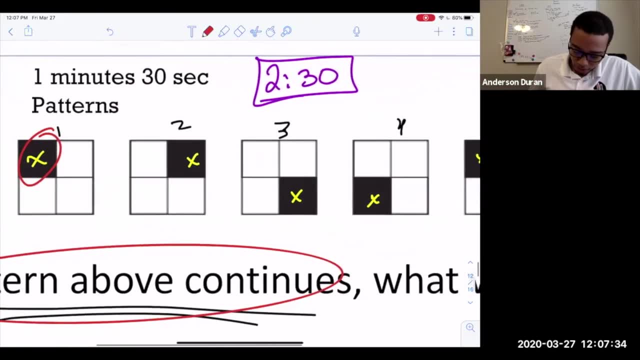 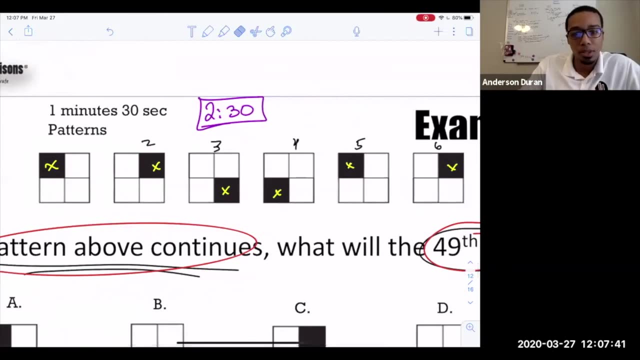 without counting yourself. So we want the pattern to continue, We want shape number 49.. Okay, So, with what we have here, everybody, what's the pattern that we notice? What's the pattern that we notice In English? 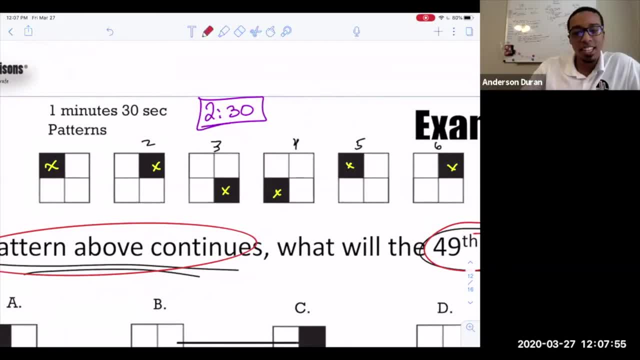 In English. What do we notice? the pattern is in English, Okay, So it repeats. So, Diana, how often does it repeat? What do you mean by that? Let's be more specific. That's a good start, but let's be more specific. 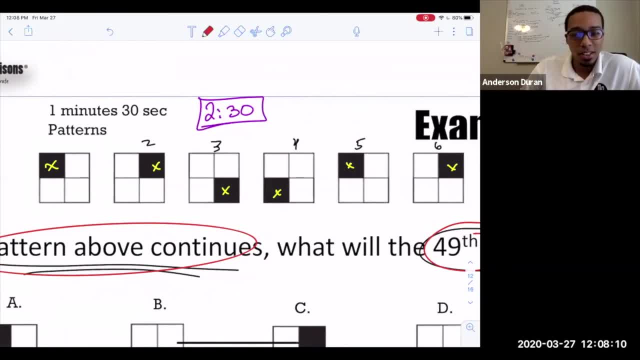 Squares are moving in an order. exactly. It's going clockwise, same pattern. after four. There we go, Christina, That's what I was looking for. After every four, it's the same pattern When you look at 1,, 2,, 3, and 4, check it out. 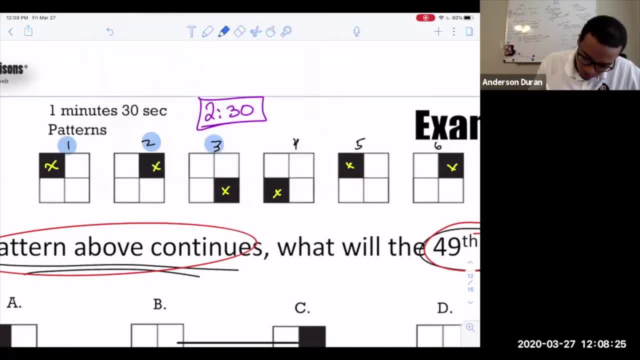 What we see are again 1,, 2,, 3, 4.. But then after 4, number 5 is the same thing as number 1.. Number 2 is the same thing as number 6.. So we see that it's going to continue on in that pattern. 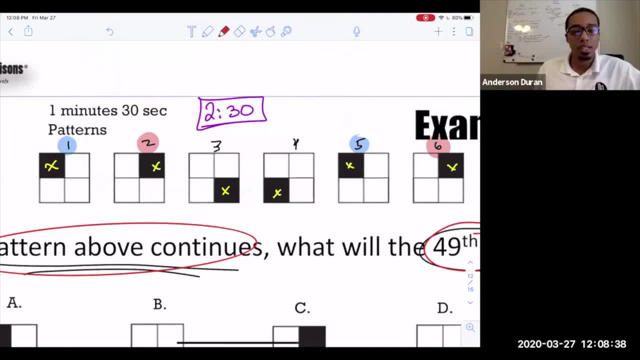 That's the suggestion that we're seeing right here. So, with that said, the pattern that we see is that it repeats after every four, So again repeats After every four, After every four, So again repeats After every four. 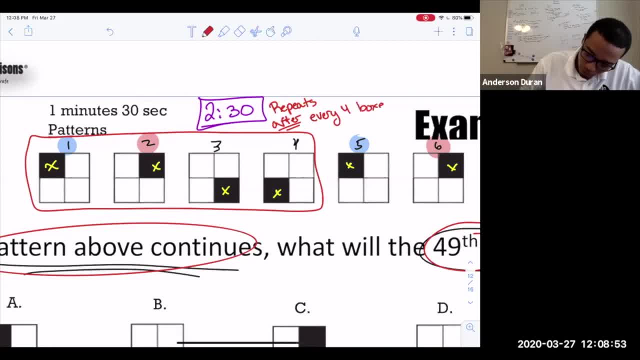 So again, repeats After every four. So again, repeats After every four, Every four boxes. That's the pattern that we see. You're good, Dan, It's all good. So again, the pattern that we see is that it repeats after every four boxes. 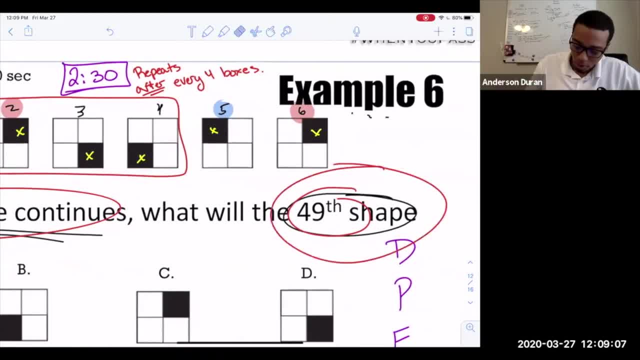 If we're looking for the 49th shape. let's talk about that for a moment, Because if we're looking for the 49th shape, then what this tells me is that, well, if it repeats after every four, well, how many times does 4 fit inside of 49?? 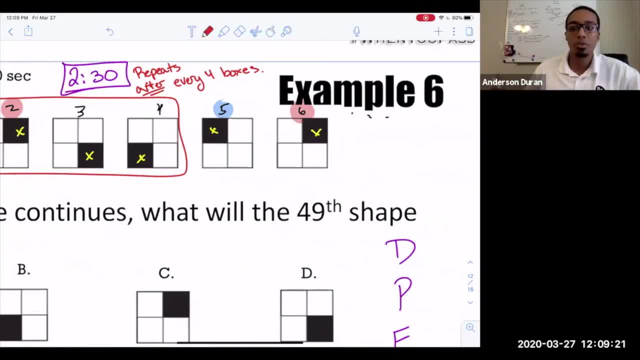 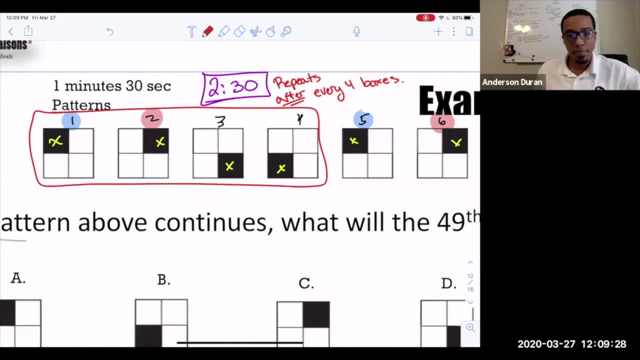 So everybody ask yourself that: How many groups of four can fit into 49?? Or how many cycles of four will we see in 49?? Exactly, We'll see 12 complete cycles. So here's what I mean by that. 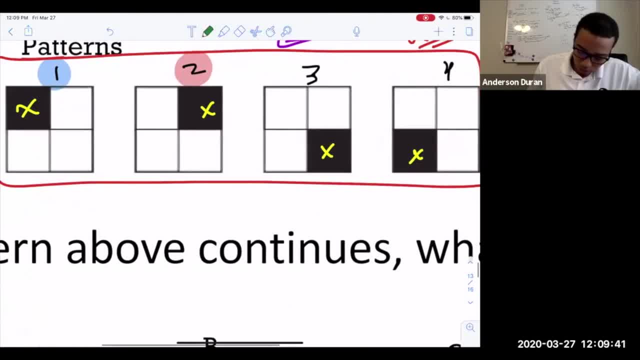 And I'm going to use green and zoom in only on the four here. So we see that this is going to be 1,, 2,, 3, and 4.. This will be 5,, 6,, 7,, 8.. 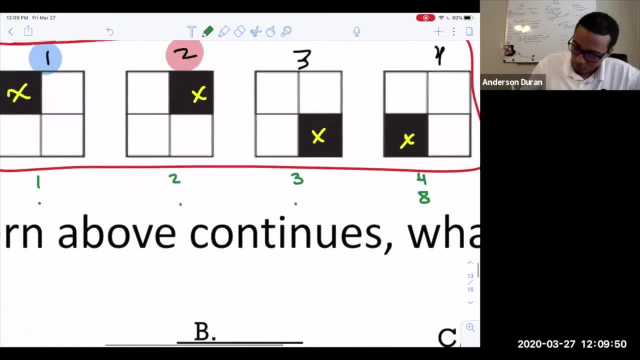 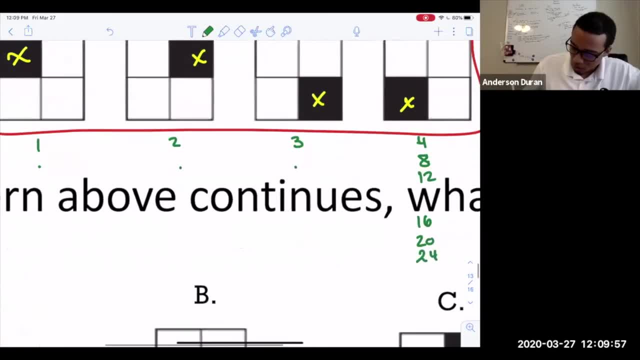 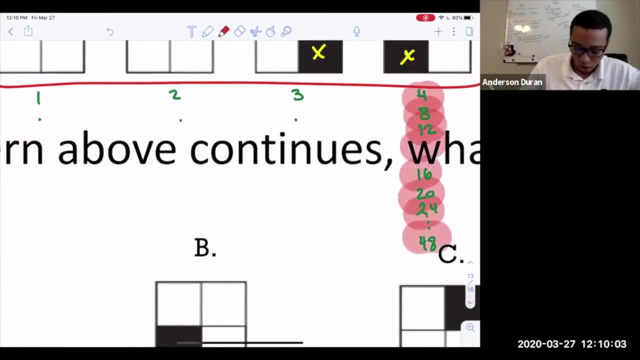 And we would have then 12,, then 16,, then 20,, then 24.. And it would continue on, and continue on, all the way down to 48. Because these are all of the multiples of 4.. These are all of the multiples of 4.. 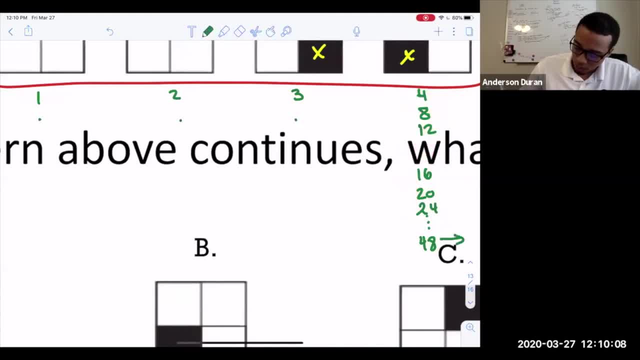 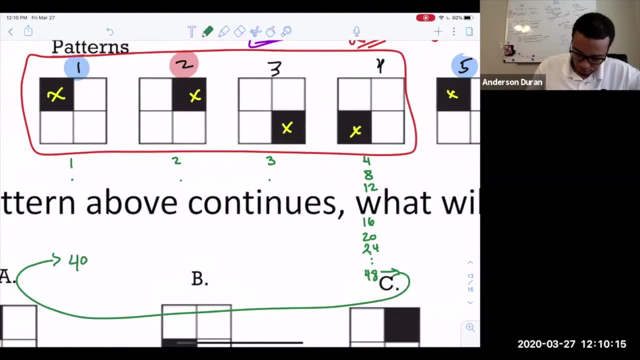 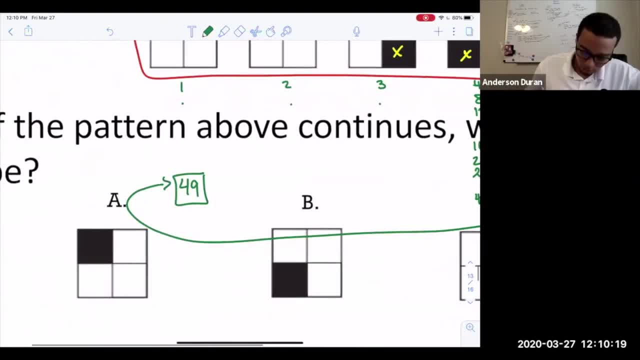 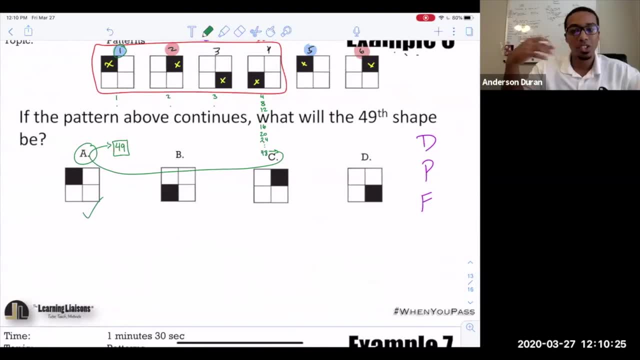 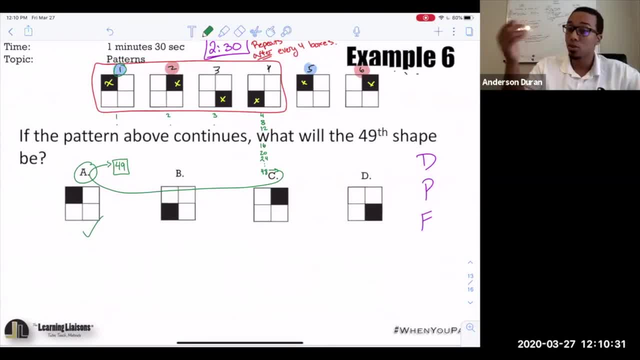 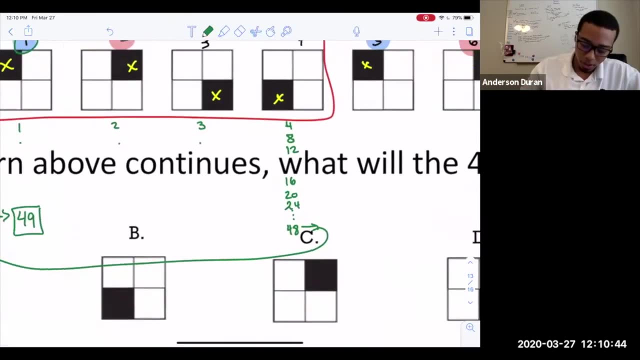 Again. one, we can just count it all the way around, Or two, we can use the pattern to get it done in a less stressful manner. So I'm going to go over that again Because I want us to really grasp that. 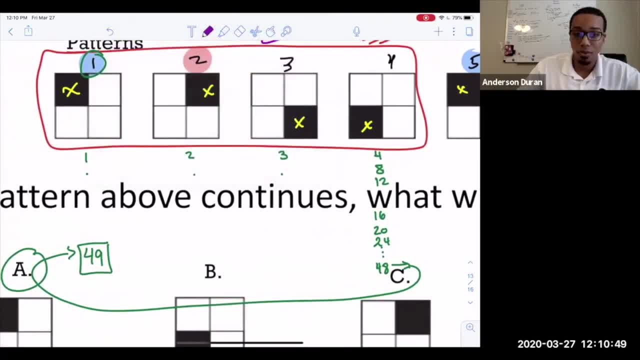 So, again, what we have here is that it repeats after every 4.. So the 4th box will be this, So will the 8th box, So will the 12th, Because it's going to repeat again every 4.. 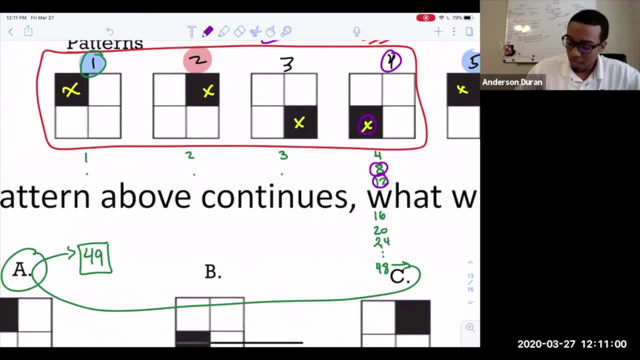 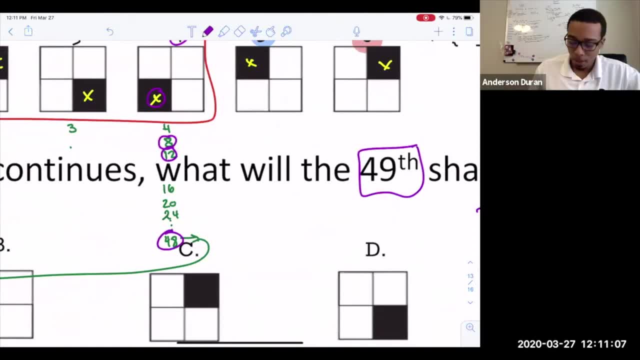 So just keep adding 4 and keep adding 4.. We can get as close to 49 as possible with 48 if we keep adding the 4s. But the thing is we want the 49th shape And we know that it's going to repeat after this one. 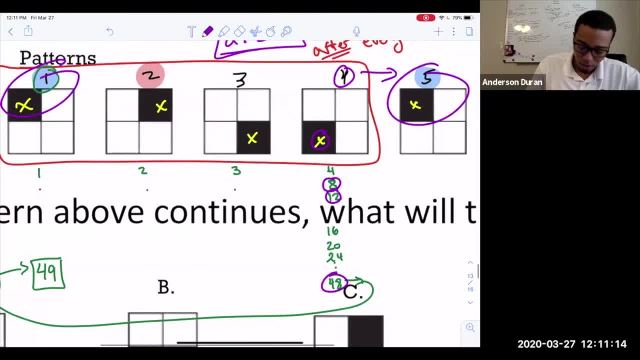 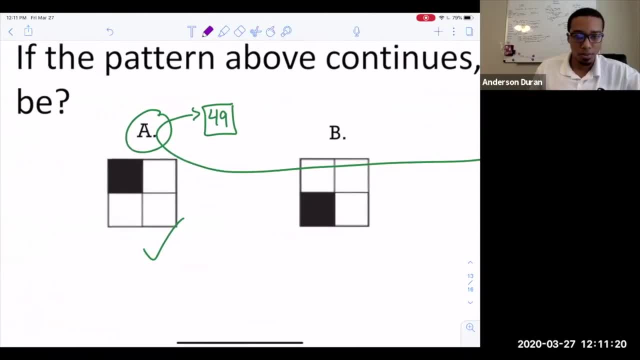 The same way that you see here. So we're going to go over that. You see here and here. So with that said, boom, that's how we get there, We're all good. The reason that it's not 49 divided by 6.. 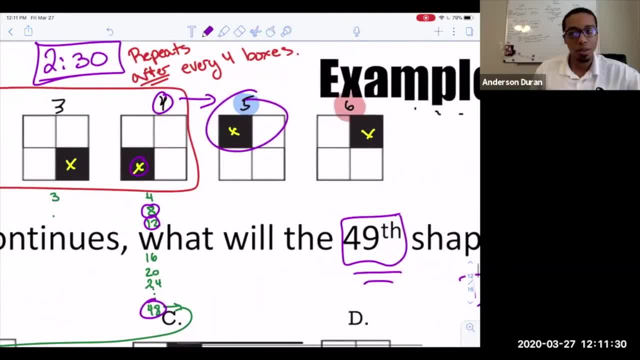 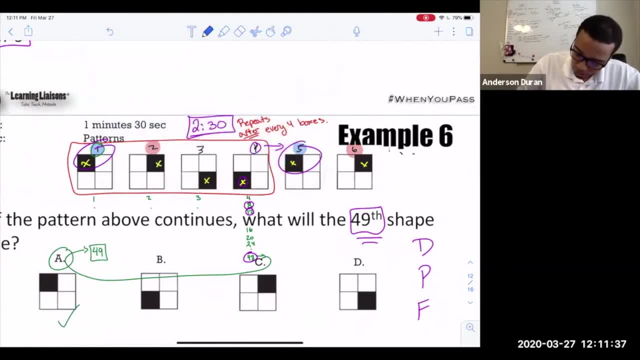 So if it still gave you the same answer, it looks like we may have gotten lucky, or it may have been just a coincidence, Because there's no logical way that it would repeat after every 6.. Because what this is suggesting is that the 7th one will be a box where this one is covered. 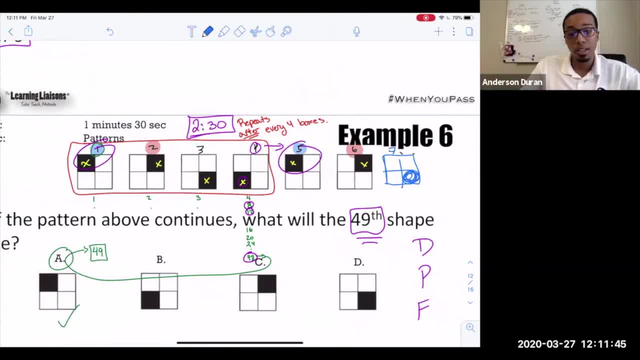 And that goes back to number 3, not number 1.. So be careful about that. Yeah, we may have gotten lucky and gotten it right this time, But just be careful about applying logic that hasn't been proven moving forward. So 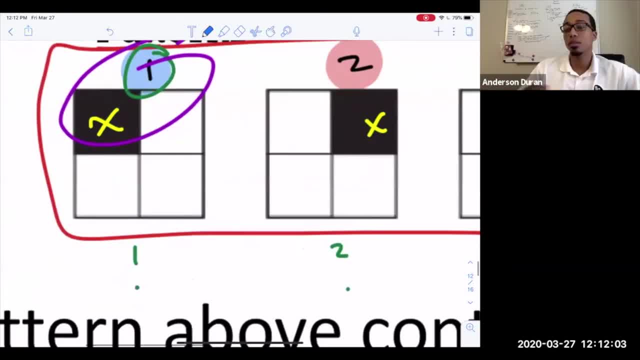 The solution here. there's 2 methods, again One, like I said before, the first way, 1,, 2,, 3,, 4,, 5,, 6, and just keep going all the way around, And then the better way would be 8.. 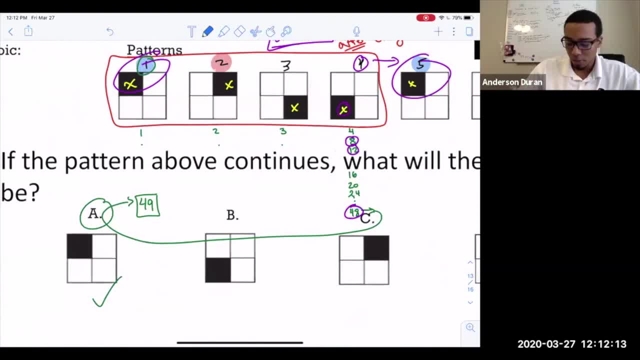 would be to use the pattern recognition and just simply say: okay, it repeats after every four. I know that four times 12 is 48, and so one more is 49, so I'll move one shape over 49 and boom. so those are the two different methods that we can use. both work out just fine. 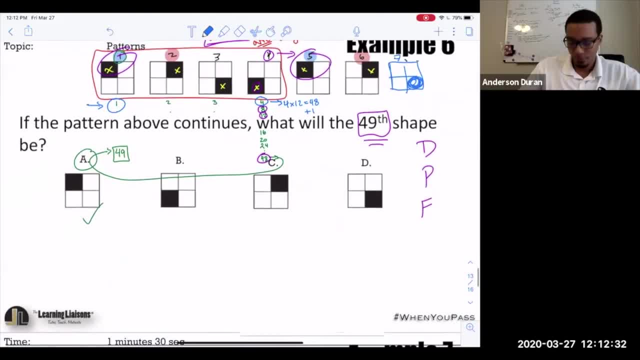 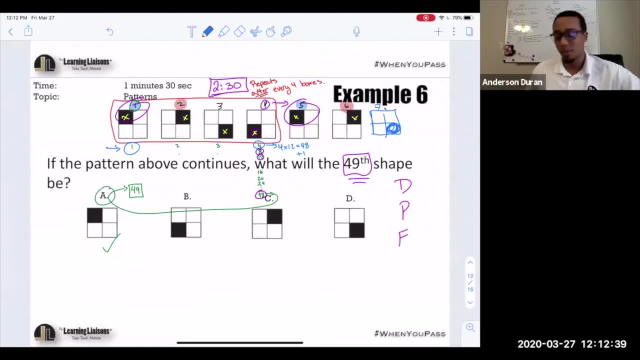 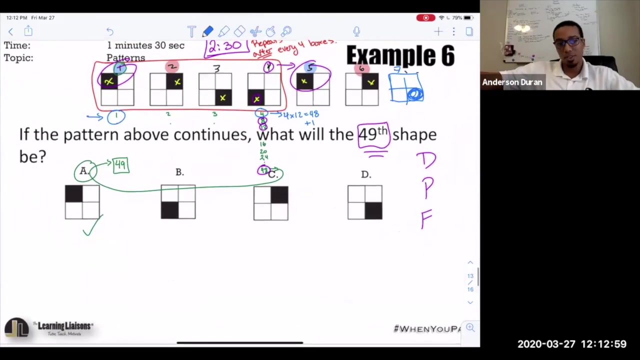 so we have one last problem to do here, everybody, we got one last problem. so who is excited? who's ready to tackle this? one last problem? that's right, who's ready to kill this? who's ready? give me a big old excited? yes, me. as many exclamation points as you want, less than 100? all right, everybody, let's go ahead and. 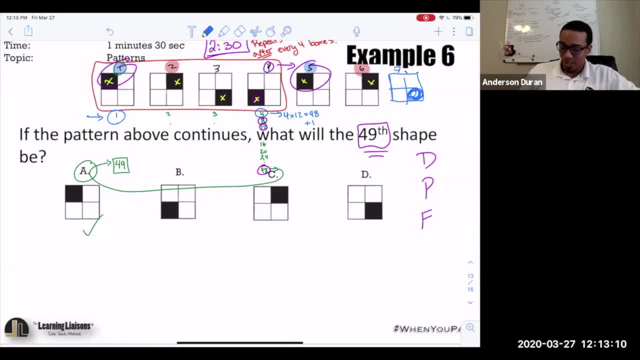 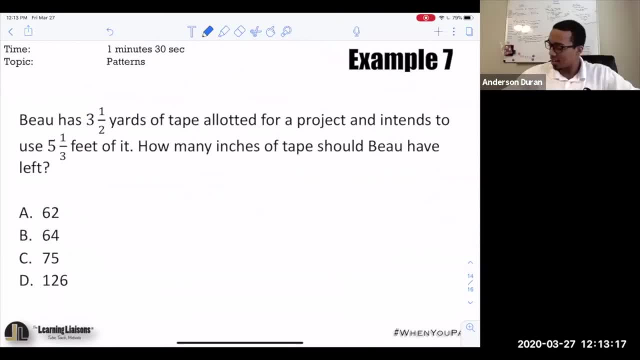 tackle this. one, let's get it. three, two, one go. i'm giving you one minute 30 seconds. let's get it done. you, you all. right, that is it time. three, two, one answers. and even if you- and let me know if you ran out of time, let me know if you weren't even able to get. 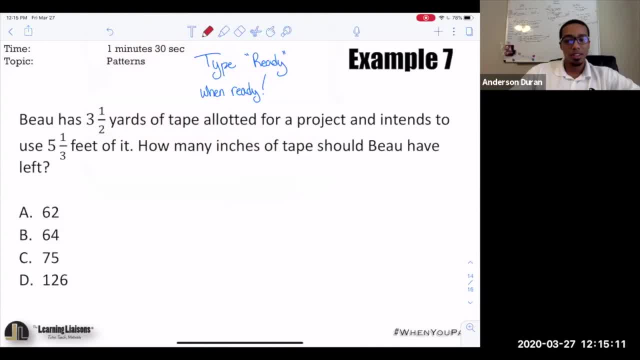 get to the answer. so a lot of us ran out of time. some of us are ready, didn't finish, so this is a type of problem that we're going to want to work to get right fairly quickly actually. so here is our solution, and we want to get quick of these because, again, these are topics that we can recognize. 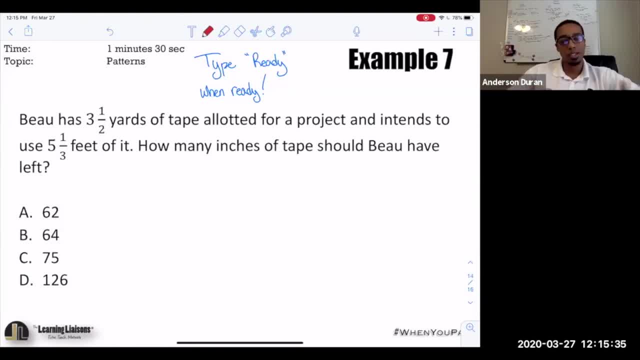 on an everyday basis may take us a little, you know a couple of seconds to know the relationships, but these are concepts that we know, so let's go ahead and start it off here: destination plan and follow as always. so destination: well, we're talking about bow, so bow has tape that he's using for 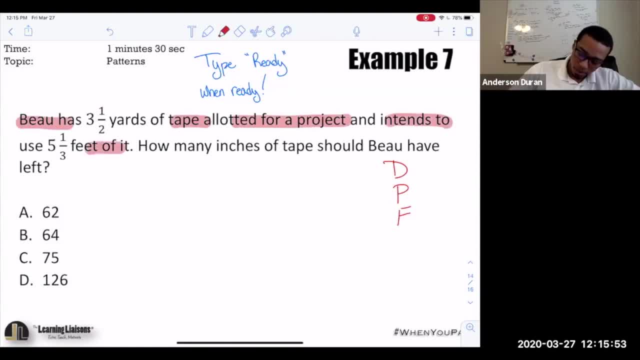 a project and he intends to use some of it. how much of the tape should he have left? did i read that in english, or what right? i just read them as english as possible. beau has this much tape for a project and he intends to use some of it. how many, how much tape? 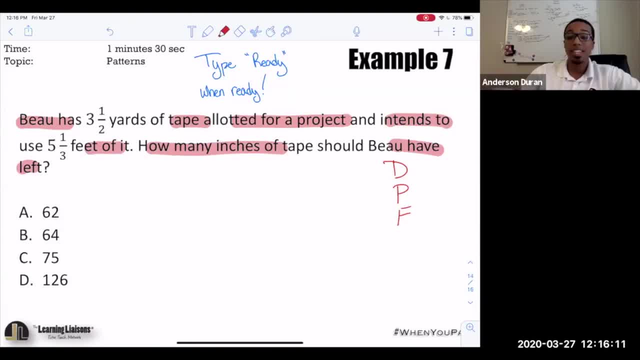 does he have left? that's in english. that's how you want to read it. avoid the numbers, avoid those measurements. you can go ahead and just gloss over it and talk about what it is generally. that's really what i recommend you do, simply because it's a lot harder to process everything when you're really 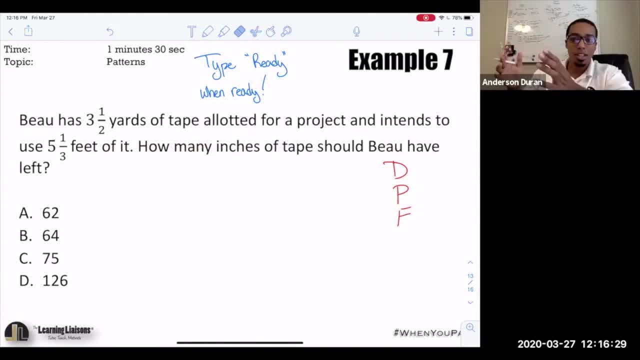 looking at the important information and the nitty-gritty at the same time, like no, just start off with the simple stuff, then build your way up. so destination: we want to know how much tape is left. okay, how much tape is left? so in real life, let's go ahead and just ask ourselves. very straightforward, very simple. 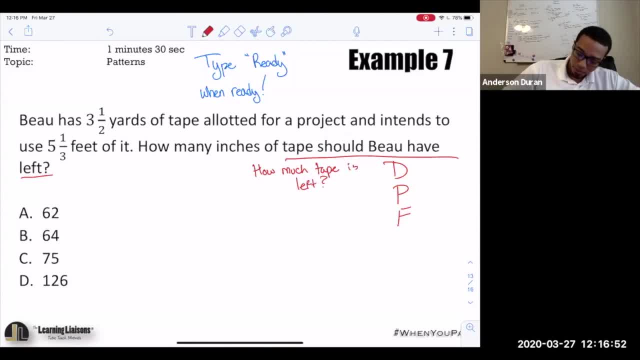 um, if we have this much tape and then we use some of it and we want to know how much is left, what math, what simple, simple, simple math idea applies here again: if we have this much tape, we use up this much and we want to know how much is left, what simple math do we do? 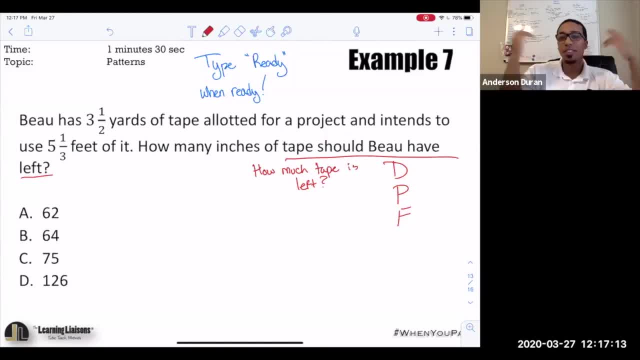 if we were actually there, i love it guys. yeah, subtraction, that's exactly what we would do. we would kill that right there, simply. so we are looking to subtract, subtract, and you know if we're thinking about this in english, the idea is subtract, total or subtract what we used from the total. 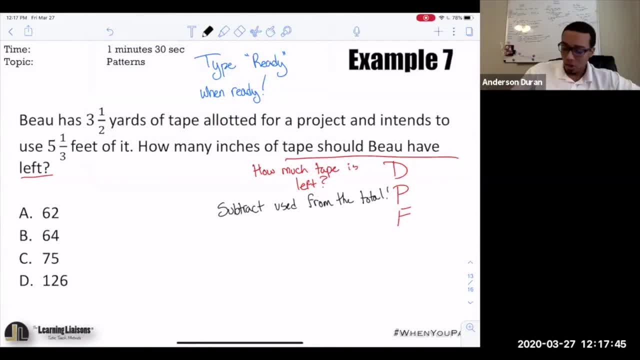 subtract what you used from the total. that's what you want to do, so that's the idea. now all we have to do is just plug in those numbers, all right, so what's the total? well, it looks like Boe has 3.5 yards of tape. 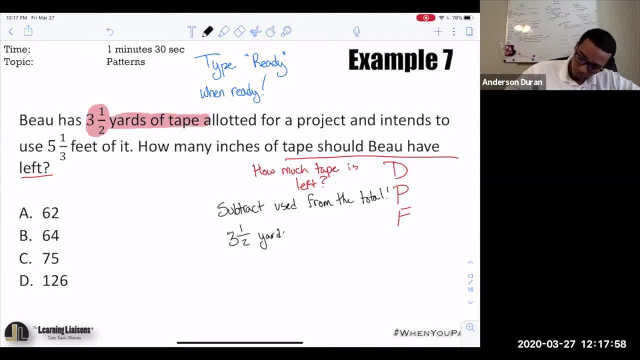 so we have three and half yards minus. all right. and how much did he use? five and a third of a foot. okay, five and one third feet, that's what we're subtracting. all right, that's my plan. now, another thing that i want to take care of. before i go into that half meter, is adding in a new exponent. okay, I already knew that i'll write a comma for the first. all right now. another thing that i want to take care of before i go into thousands of and I'm going to Quit: она минут dos. 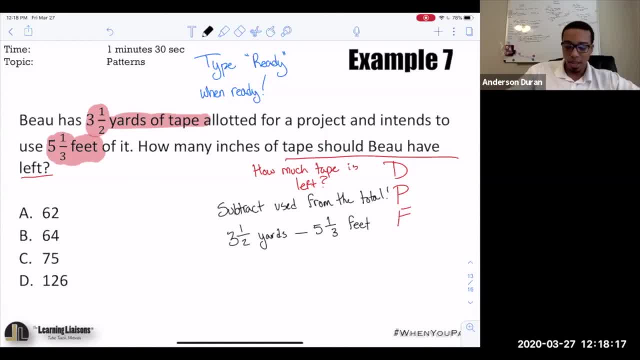 go into that following phase before I compute is recognize that, oh, yards and feet, that's not a good look. Also, well, if I'm trying to think of this, I need these in the same units. But to get these in the same units, we first need to ask ourselves: is there a unit that the problem wants? 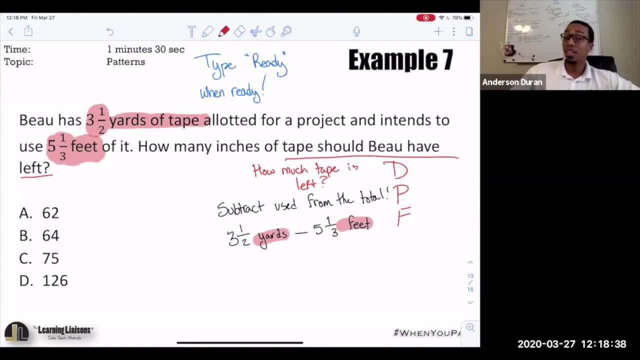 us to do? Is it yards or is it feet? Well, the thing is, the problem actually wants it in inches. So this is why reading a problem in the context is so important. Before we get to calculating, before we do all that hard work, we need to just analyze and see where we need to go. 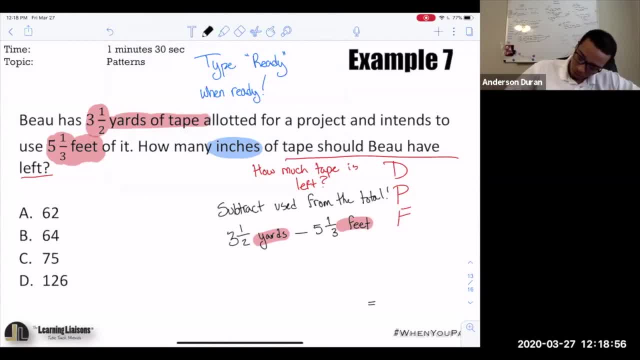 So we need to turn this into inches. All right, we need to turn this into inches. So here's what I'm going to do. I'm going to think of two ways to do this. The first way is to turn yards into feet, And the second way is to turn yards into feet. So we're going to do that in inches. 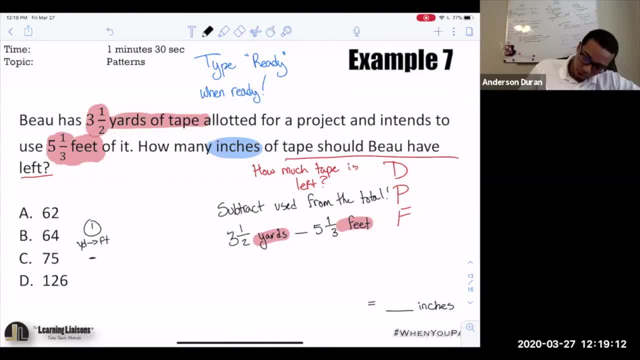 feet, then subtract and then turn the feet into inches. That's one way. Another way is to turn both into inches, then subtract and then I'm done. So one way is three steps, The other way is two steps. Which way would you guys like to see? Write it on the chat box: Would you rather see me go yards to? 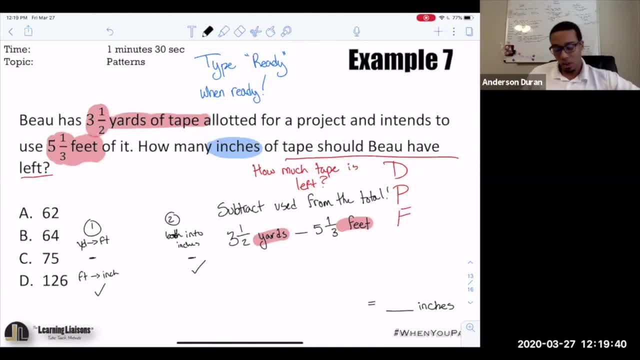 feet, then subtract and then turn those feet into inches, or turn everything into inches and then subtract. So some say straight to inches, some say yards to feet. first, option one, option two, the first way. So it looks like: see, this is not. this is really cool to see to me, because not everybody. 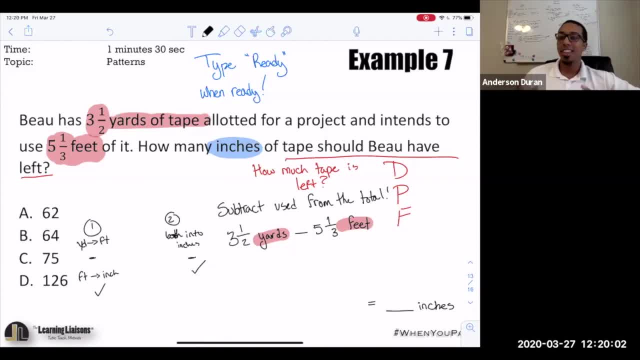 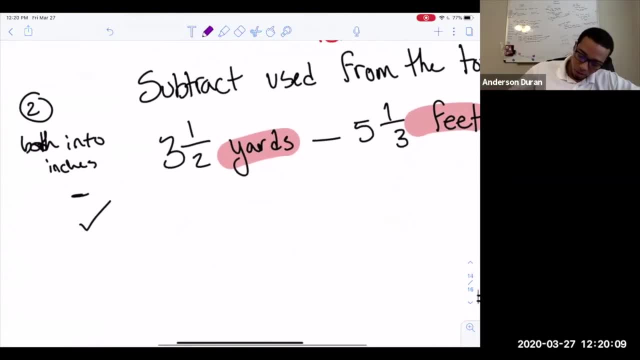 likes to do it the same way, See, And there's always more than one way to do it, So I'll do it in both ways to really satisfy both sides there. So let's go ahead and look at number one, turning them both into feet. 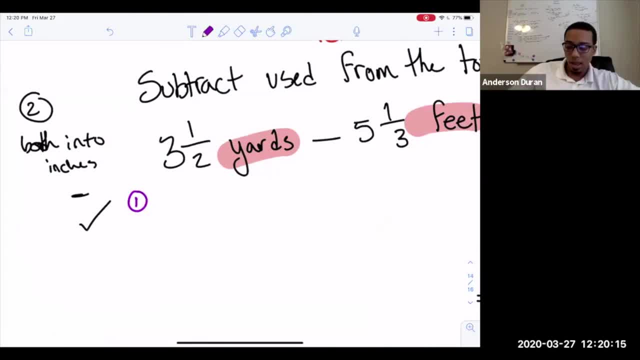 What I'm going to do is I will turn the yards into feet, and we know that one yard equals three feet. So what that tells me is that I need to multiply every yard that I have by three to see how many feet are in there. So it's taking three and a half times three. 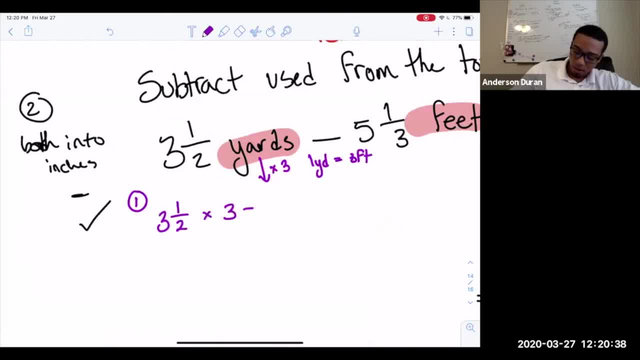 And then I can say actually turn everything in my first fraction by half. Well, I'm going to have to do here is I'm going to have to actually turn this mixed number into an improper fraction to multiply So three and a half. what do I do there? Remember to turn a mixed number into an improper fraction. 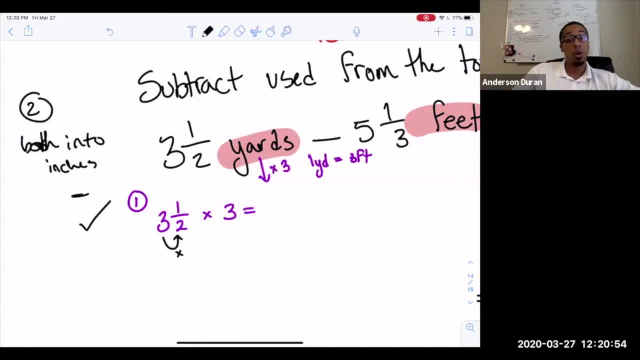 what you want to do is multiply the whole number and the denominator, because the denominator is the whole. So you have the whole is two pieces, so we have three groups of two pieces because there's three holes, and then you'll add the result to the numerator. 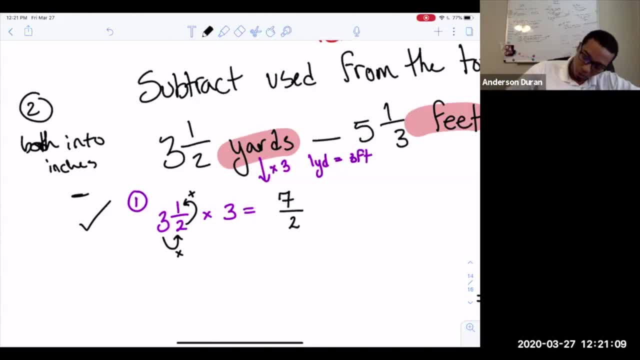 So that 6 plus 1 is 7.. 7 over 2 times 3.. 3 is the same thing as saying 3 over 1.. So I can just write it like that if I'd like to Again. anything divided by 1 is just itself. So 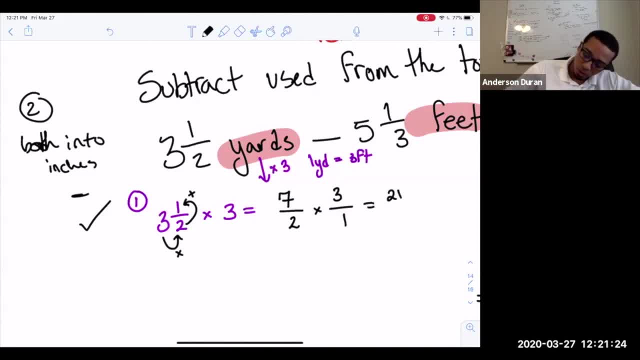 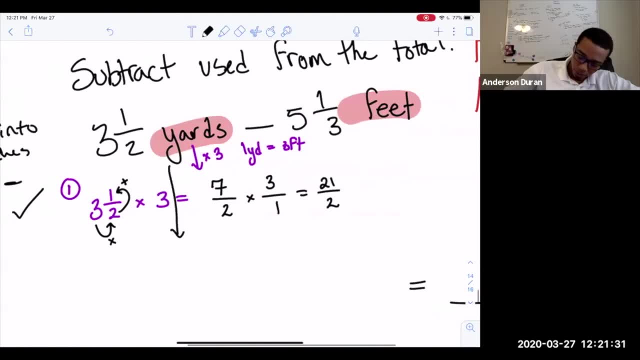 we have 7 halves times 3 over 1, which turns into 21 over 2.. So, with that said, this would turn into 21 over 2.. 21 over 2, we can go ahead and convert that back into a mixed number if we'd like to. 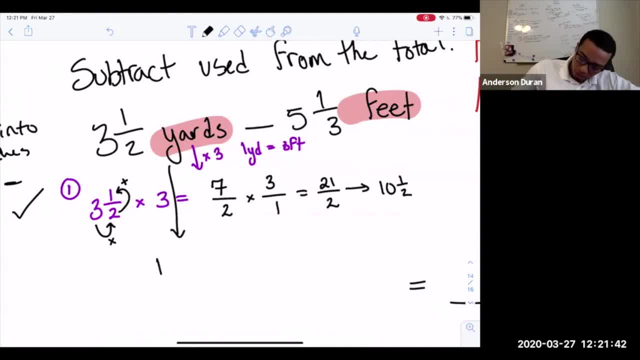 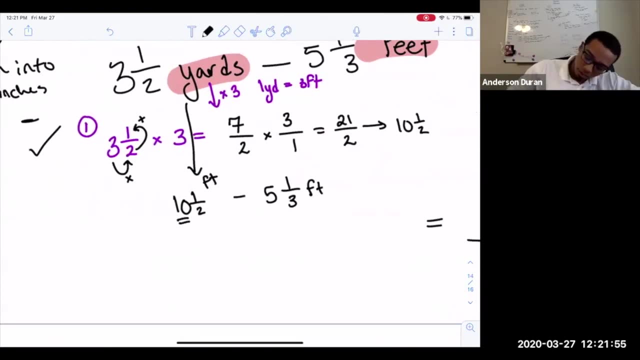 That would be 10 and a half. So we have 10 and a half feet, minus the 5 and 1 third feet that we had from earlier. So from here now we can just go ahead and subtract and we're done. So 10 minus 5 is 5.. However, though, what's? 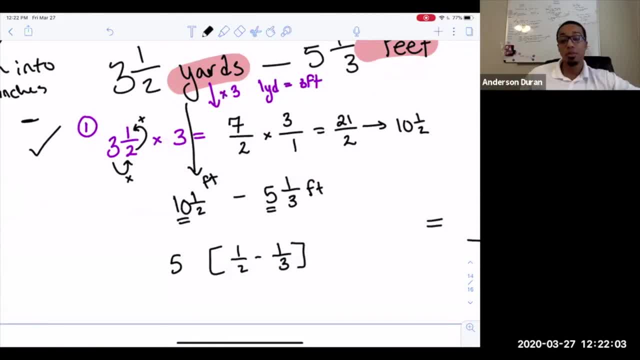 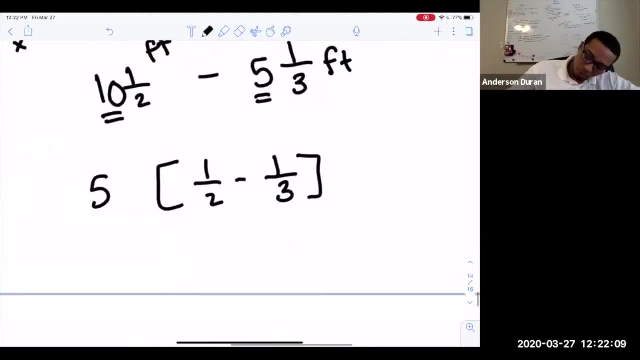 1 half minus 1 third. So from here, what we can do is, well, turn them into the fraction with the same denominator. So, with that said, I can turn these both into a denominator of 6. Because 2 and 3 both go into sixths. So with that said, 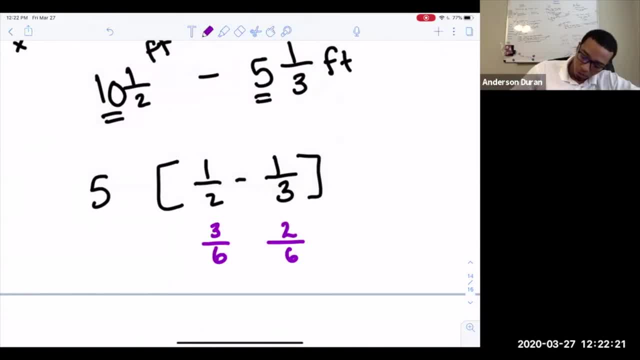 half of 6 is 3.. A third of 6 is 2.. So 3 sixths minus 2 sixths, that would become 1 sixth. So we have 5 and 1 sixths feet From there what we would do, remember? we wanted this to end up in inches. 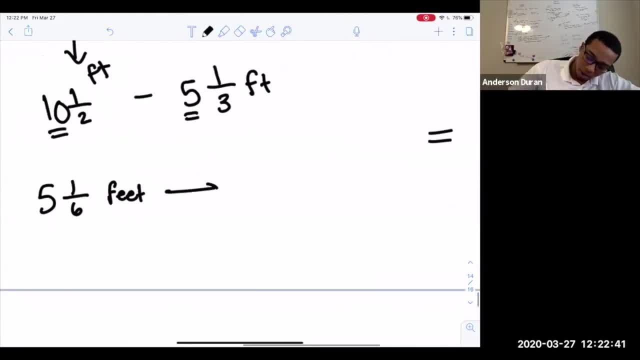 So what we have to do here is multiply by 12, because every foot contains 12 inches. We want that knowledge as well. So from there we multiply that by 12.. 5 and 1 sixths times 12 is 5.. 5 times 12 is 60.. 1 over 6 times 12 is 2.. 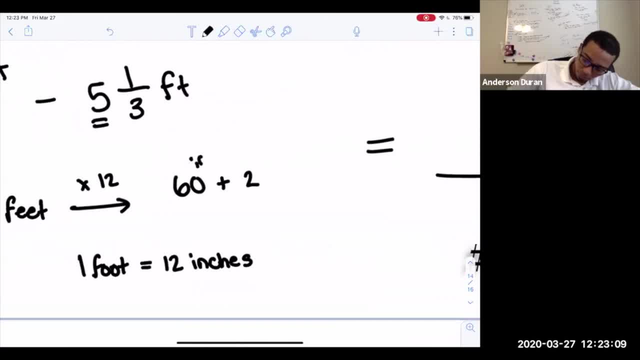 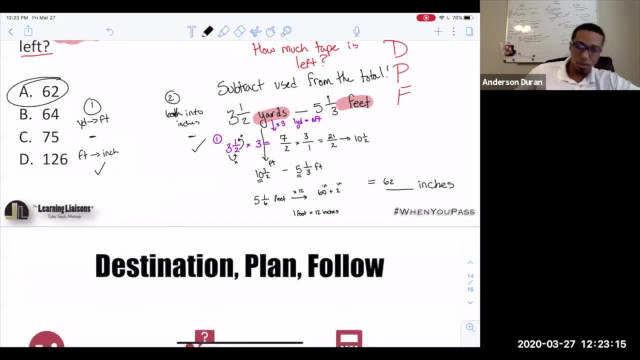 Oops, I didn't write it out there, Giving me 62 inches Making A the answer. So did that process make sense? And if not, let me know, because we're going to get ready to go over the second method now. But that's it. 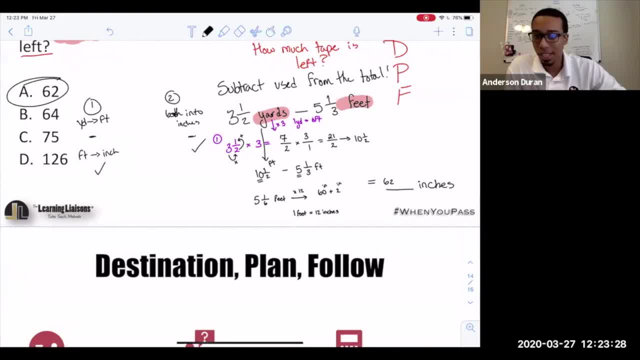 But that was the first method, Again, turning yards into feet, doing the subtraction and then doubling back and making it all inches at the end. Who liked that method, Yes or no? So Samantha likes it and Deer is like, not really. 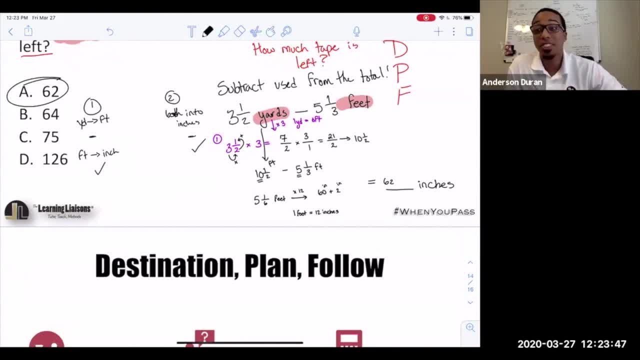 Veronica's like no, but Ollie Wendy got it, Clara. So look at that Half and half again. So it looks like those of us that really wanted this method enjoyed it, Those of us that wanted the other method, kind of said. 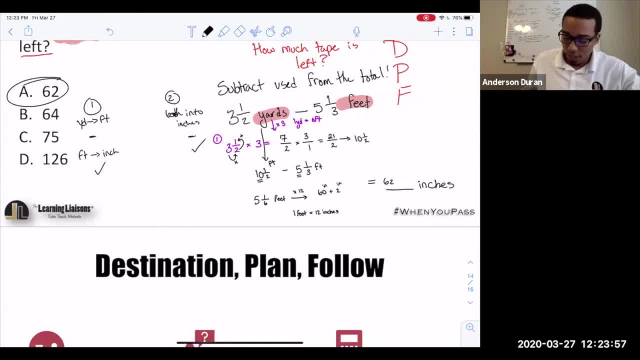 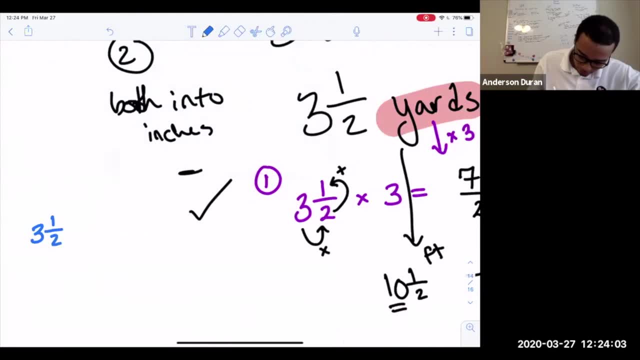 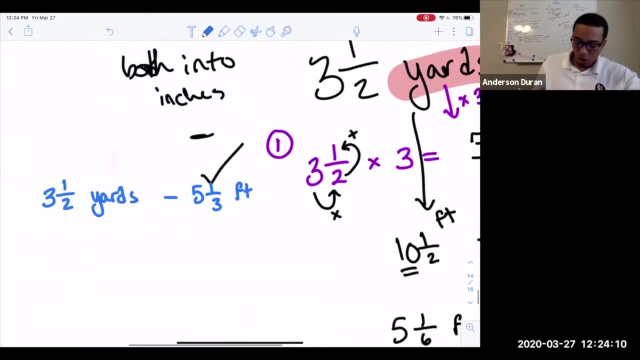 nah, The one-third into inches. So we're going to do that right now. So we're going to turn both into inches right now. Let's do this in blue: Three and a half yards minus five and one-third feet. So let's start off with the yards and 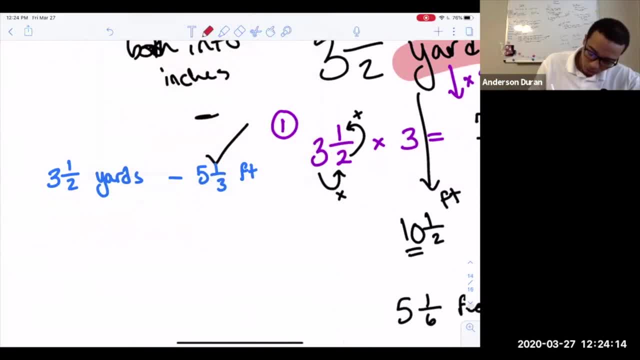 let's turn that straight into inches. So we're going to begin by converting this into a mixed number. just like last time it was 7 over 2 yards From here. to turn it into feet, we'll multiply it by 3.. 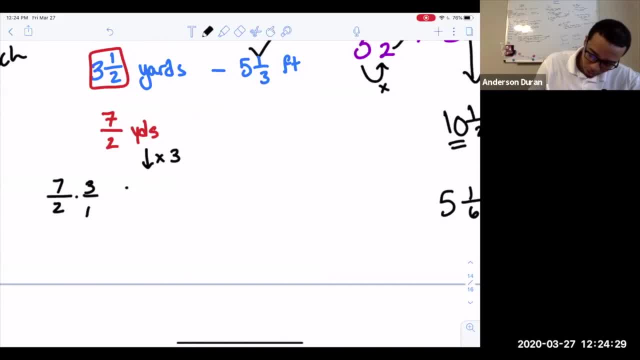 So 7 halves times 3 over 1, it gives us that 21 over 2, and this is 21 over 2 feet. Okay, now we want to turn this into inches. now, and what we're going to do: 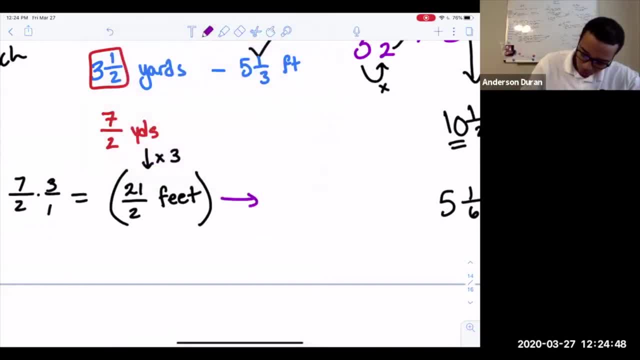 actually he's purple is. we're now going to multiply by 12 to make this into inches, So 21 over 2 multiplied by 12 over 1.. We don't have to do the complicated multiplication when we have a 2 and a 12. Cancels out to make a 6.. 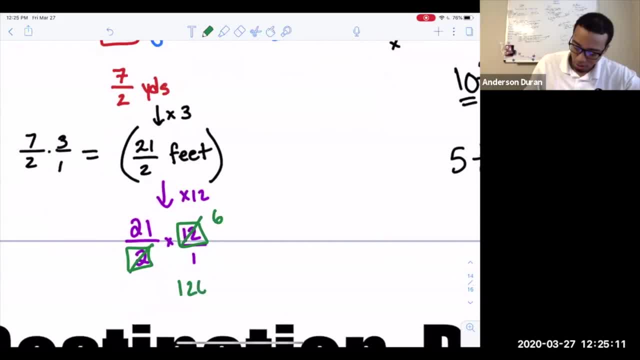 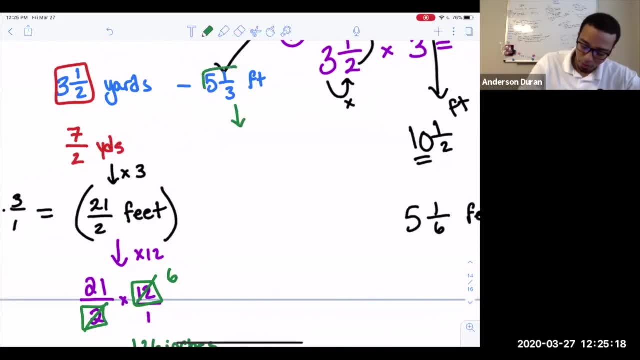 So from there we got 21 times 6, giving us 126 inches, The five and one-third feet. all we have to do here: convert that first into a mixed number, giving us 16 over 3,, again 5 times 3,, 15, plus 1 is 16.. 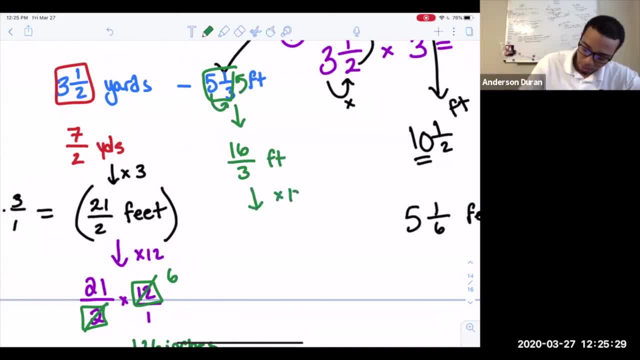 From there- that's how many feet- we have, times 12 to get to inches. So from here we're going to have 16 over 3, times 12 over 1, giving me 16 times 4, instead, and that's going. 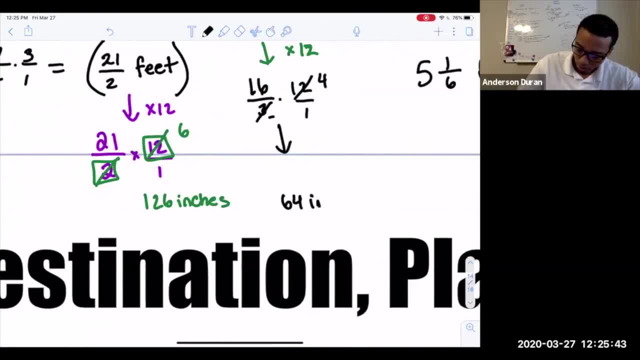 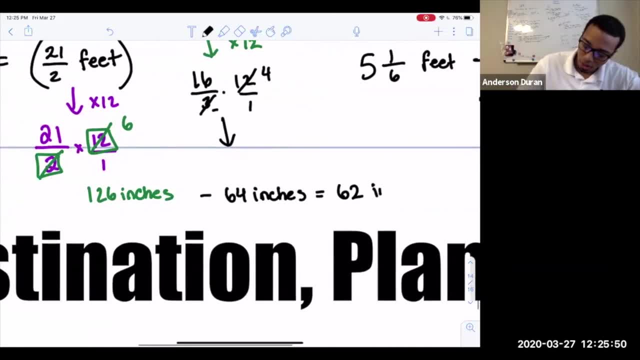 to end up being 64 inches. So once we subtract these two, we'll get 12 over 5.. That is our three times 3: two. we'll end up having 62 inches left over, and remember, this is 62 inches of tape, so i had to. 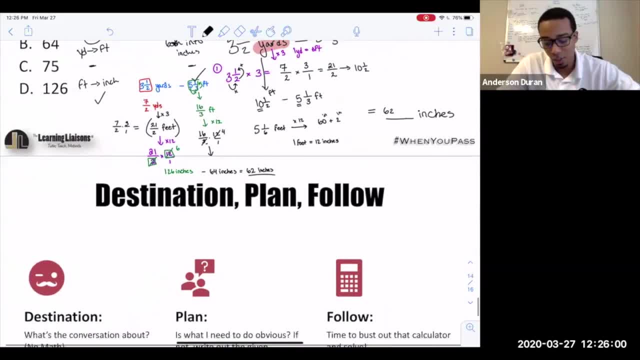 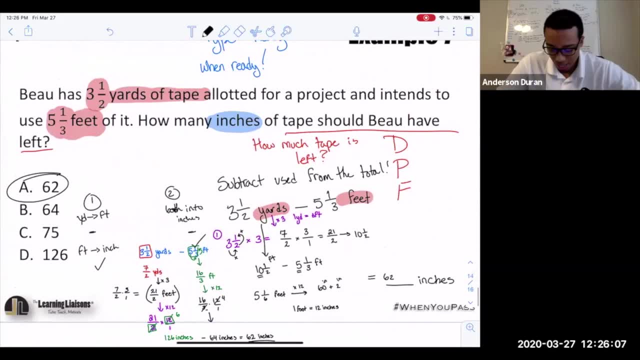 kind of speed up that process there at the end. so i do apologize because i want to make sure i let you guys out of here on time, but those are both methods. both are equally, i would say, as complicated because they both involve these same exact conversions. so, um, you know it really at that. 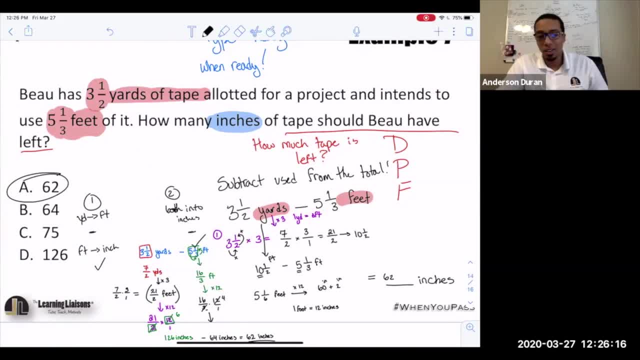 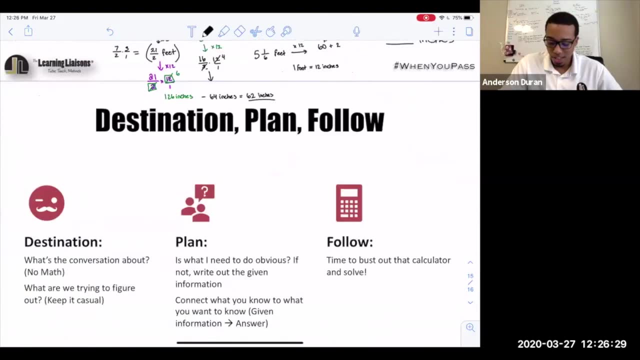 point just depends on preference, because again, all we're doing here is subtracting and then converting yards and feet into inches. the way that you do that, the order that you do that in, really doesn't matter in this problem. so it's really about your preference. so, with that said, 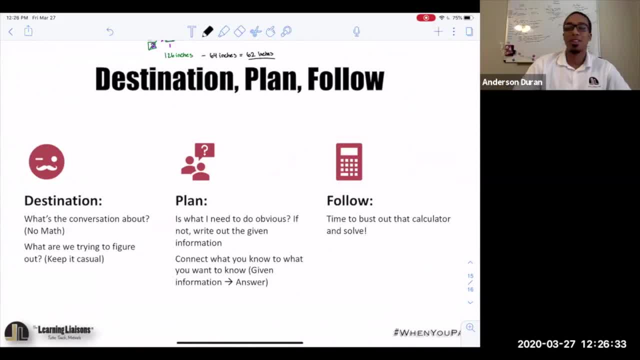 destination plan follow. what's the final verdict? on a scale of one to ten, how useful is destination plan follow? on a scale of one to ten, you? how useful is it? i am curious. you are supposed to be able to do that after a certain point. yeah right, i love that. we said eight now and then ten when you get it. that's exact, i love it, i love. 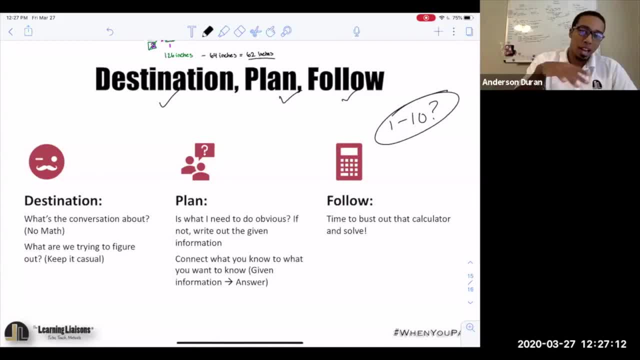 hearing that, because when you're practicing this for the first time, it takes a lot of effort to really, you know, guide yourself in that way and to recognize when you're stuck. but with practice you'll be able to see: oh, i get the destination part. i know what's going on, i know what i'm trying to look for, i just don't know. 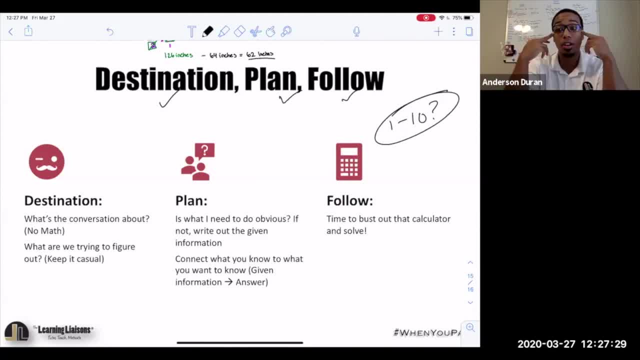 what math i need to use. boom, that tells you that you need to learn on how to recognize the math in the context. if you're not able to figure out what the question is itself, then interpreting the problem is another issue for you. so it's really about you're not able to figure out what the 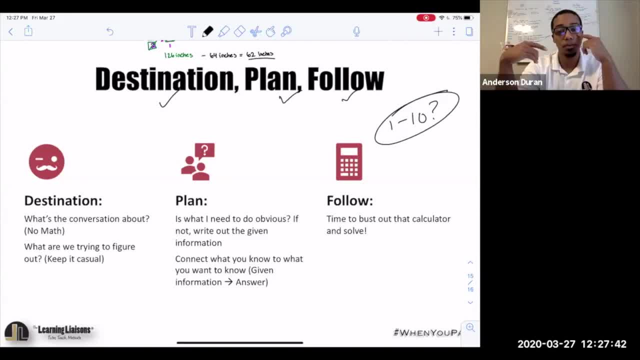 question is itself, then interpreting the problem is itself, then interpreting the problem is that you are working through, from what you have to what you need to figure out: practice, practice, practice, exactly, exactly. so, with that said, everybody you know, we, you know, throughout this whole craziness going on in the world, it's really all about making sure that we're 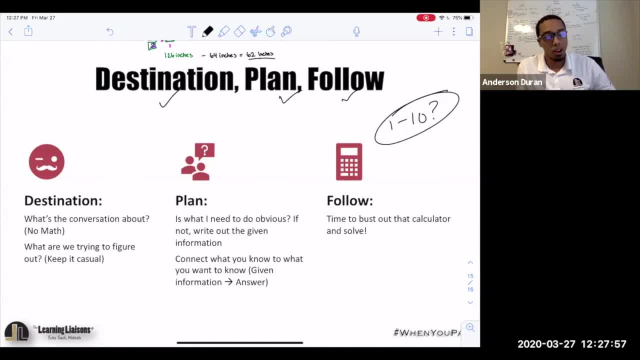 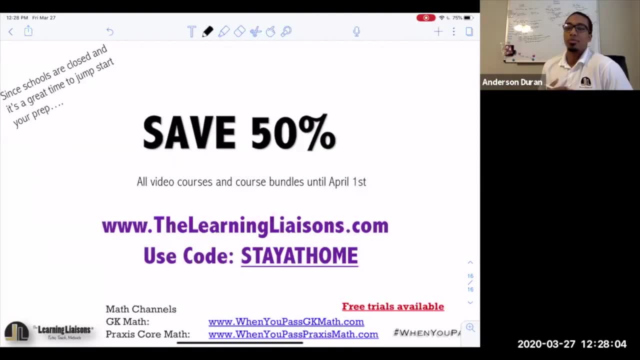 still preparing the right way. you know, i know we have a lot of time and a lot of us are at home. so, with that said, a lot of us have been to these webinars and what we've been doing is we've made everything on our websites 50 off, absolutely everything. so you know i'm going to 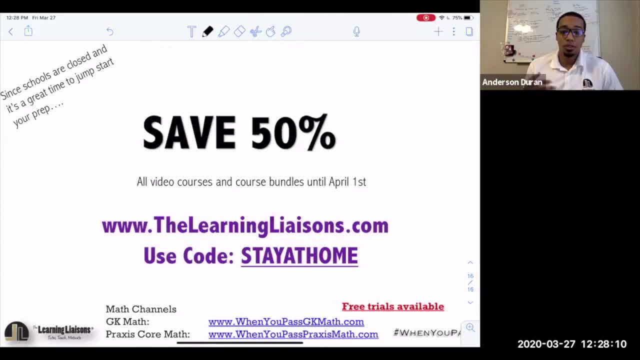 know with the. with that said, if you're looking for test prep certification, that actually helps. if you're looking for courses and materials and resources that actually work because the teachers there are actually speaking in a way that you can understand it, hey, the learning liaisonscom is for. 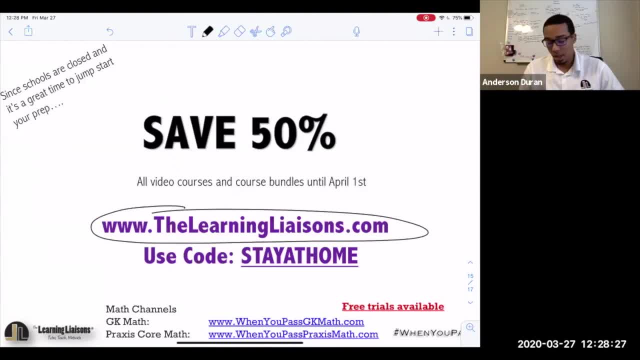 you: all of our online resources, all of our stuff, 50 off all the way through april 1st using the code stay at home in all caps. there you go, it's easy to use and you're good. but with that said, you know what did you guys think of the entire session? because i know the destination plan follow. 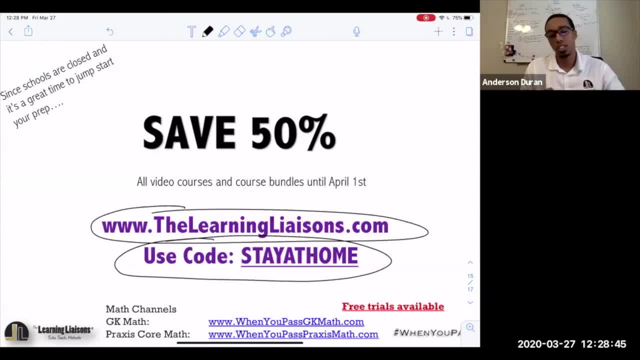 was a theme, but did you guys like the flow of the session? you like how many problems we did, how we got through it? give me that live feedback. i love it. that way we can continue improving for next time. oh sweet, perfect. thank you guys for your time. are you serious? you guys are taking an hour out. 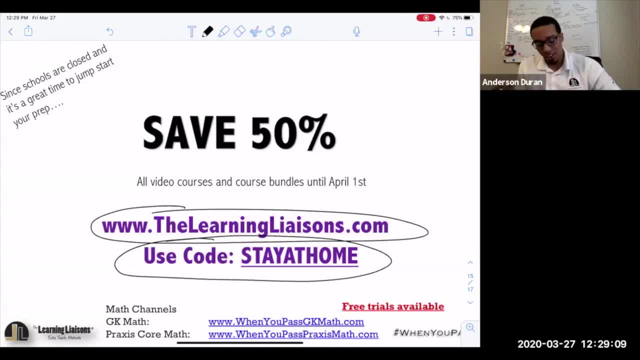 of your day, an hour and a half out of your day to be here, and you know i'm just here to help anybody that wants to help themselves, and that's clearly y'all. so i'm proud that i can be part of this. i'm glad that i can help y'all seriously. 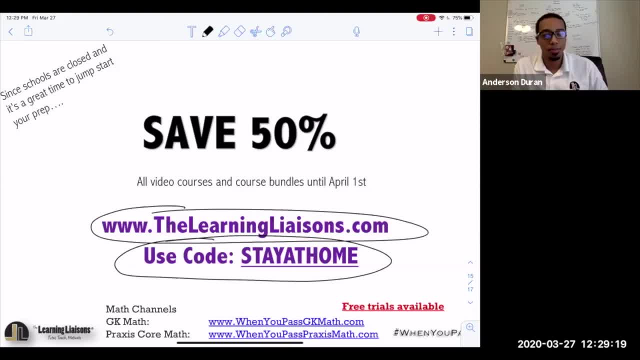 fred out to keep that in mind. thank you you. hey, you guys are welcome. so again, guys say 50 off. if you are trying to pass and get ready to pass those tests. once this craziness is over, this is your chance here. take 50 off of everything on. 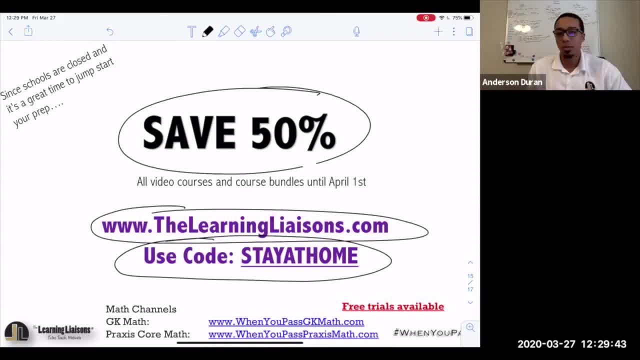 the website, get our courses, ask us questions, communicate with us all the way until you pass. we put in all that work and we have everything on your side to pass. so, diana, we will be posting this. this is actually available in our facebook groups that you're in. 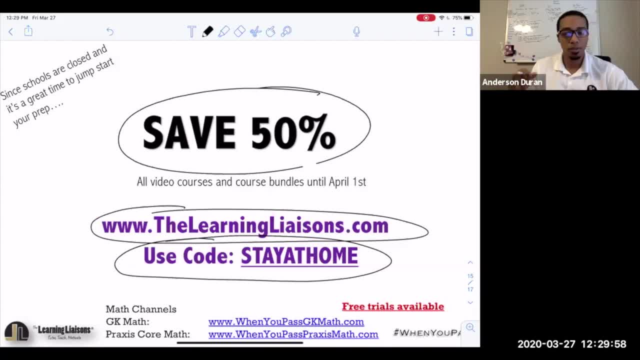 you found this through, so if you are on facebook, the video is actually live in there right now that you can go back and search through. very good, yeah, clamar. so with all the questions that i'm involved in in terms of the video, i always go through every type of solution as in detail as possible because again remember how. 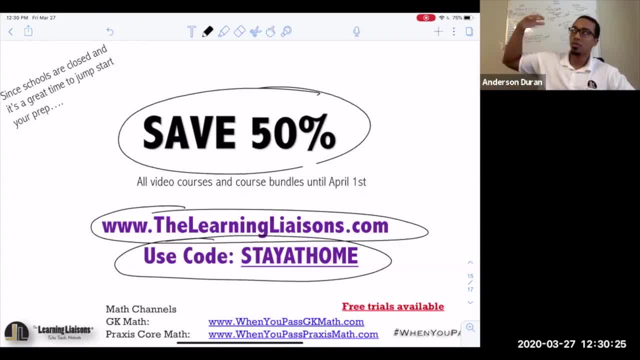 earlier i said i hated it when my professors didn't take us from where we were and i didn't go over to where they were. they were kind of just speaking from a textbook, hoping they grabbed whoever they could. i go the complete opposite way. i want to meet every learner where they are, bring them up. 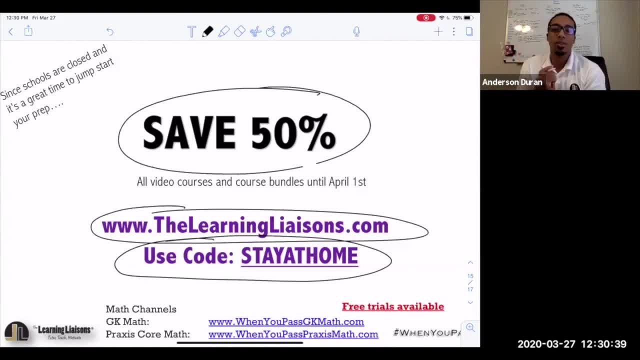 to where i believe they need to be to be successful. that's what i do and that's how i do. oh, dana, you don't have facebook, so we're going to email you a link to the recording then. that way, you have access to the recording on your email.